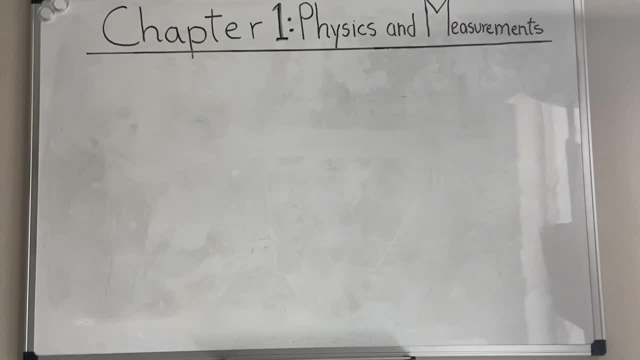 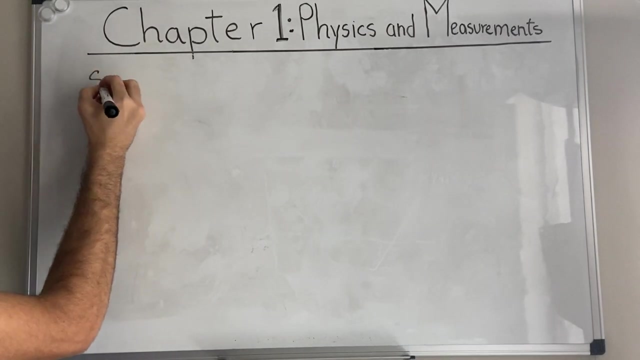 So, first of all, the first part of Chapter 1 discusses measurements. So in 1960, an international committee established a set of standards for fundamental quantities of science. It is called Système International, which is French for International System. 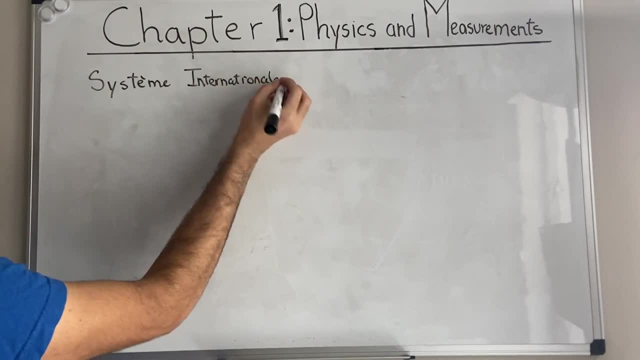 And so we usually call this SI, and you're going to hear this a lot in your physics course, And so these the fundamental units of length. this organization basically pinpointed a number of units to describe length, mass, time, among different, a number of other different types of measurements. 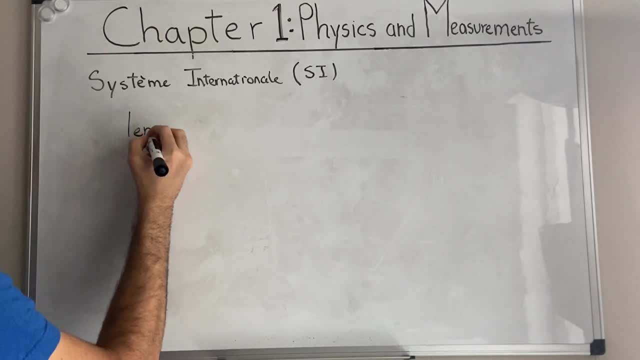 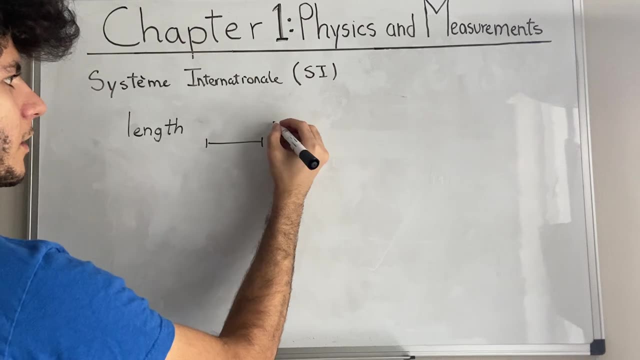 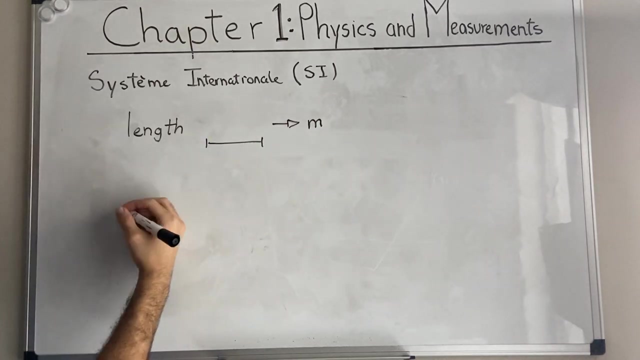 So for length, whenever we talk about length, so, like the distance, distance we're going to be dealing with meters, which we abbreviate with m, Whenever we deal with mass, which is basically the quantity of matter. I guess this is a good like image to show what it is. 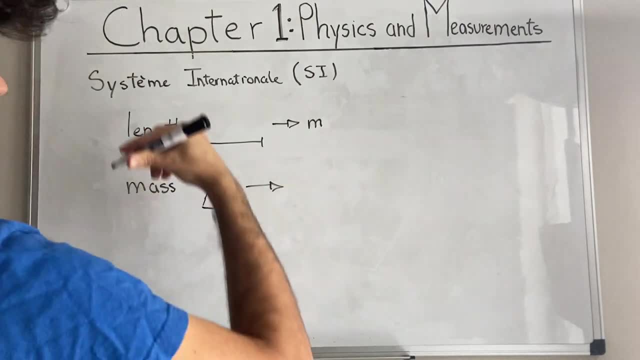 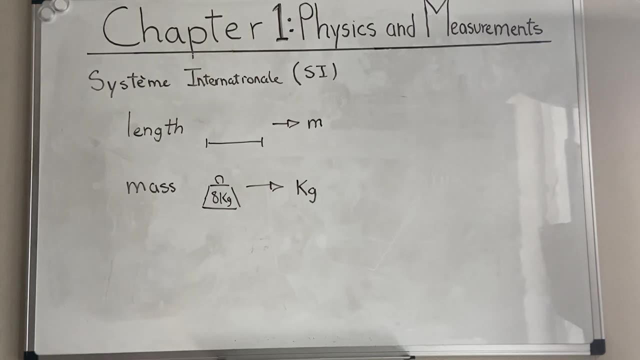 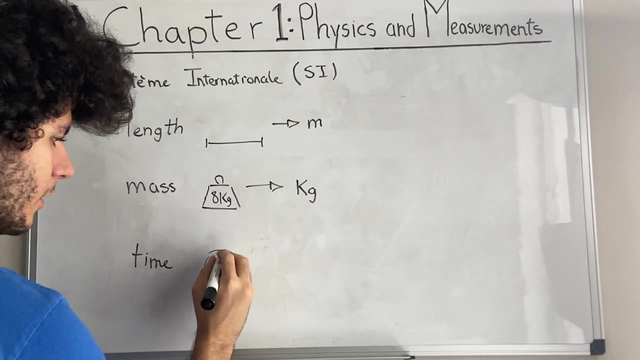 And so whenever we deal with mass- because we're working the SI units- we're going to be dealing with mass, And so we're going to be working with kilograms. And as for time, so I guess I can put a little clock here. 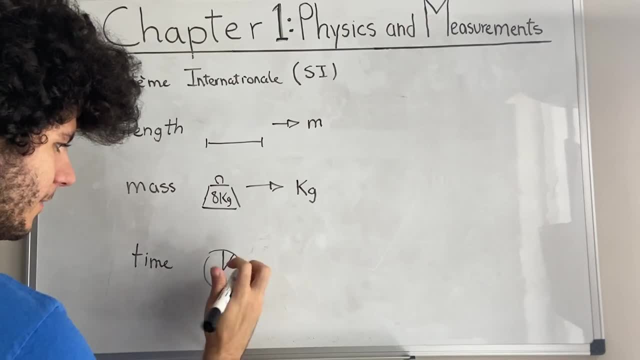 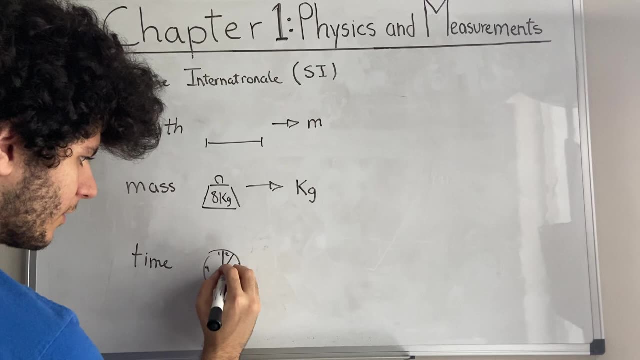 That's a really bad clock. Let's put like 9,, 3,, 6,, 12., 12., 12., 12. 13., 14., 15. 16. 17. 18.. 19., 20., 21., 22., 23., 24., 25., 26., 27., 28., 29., 30., 31., 32., 33., 34., 35.. 36., 37., 38., 39., 40., 41., 42., 42., 43., 44, 44., 44., 44., 45., 46., 46., 47., 47.. 47., 48., 48., 49., 49., 50., 51., 52., 52., 53., 53., 53., 53., 53., 54., 54., 55.. 56., 58., 59., 61., 62., 63., 64., 65., 66., 68., 67., 68., 67., 68., 69., 67., 68.. 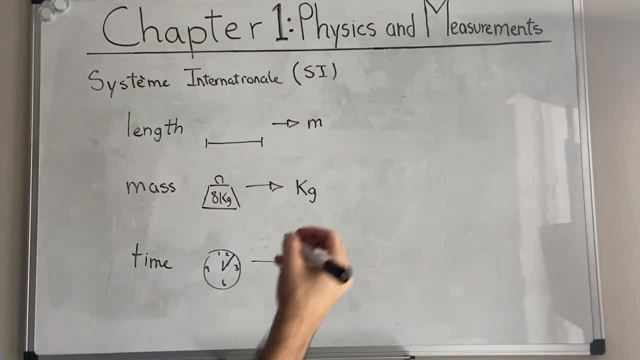 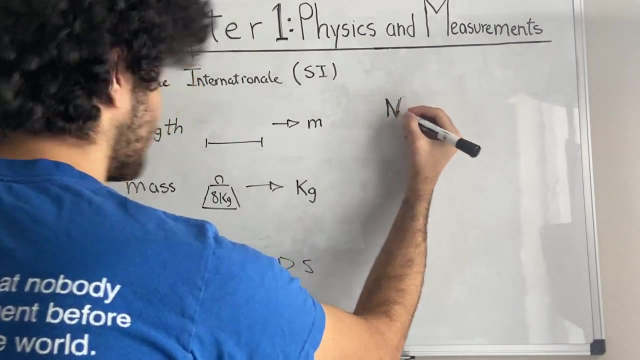 göch, 67., 67., 68., 69., 70., 71., 72., 72., 73., 74., 74., 75., 65., 76., 76.. The way that we can measure how hard I'm pushing is with the unit Newton, named after Isaac Newton, of course. 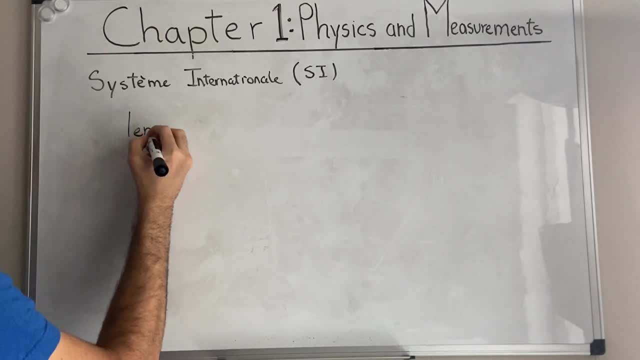 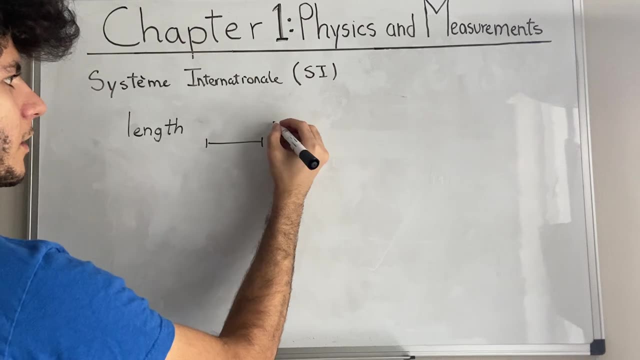 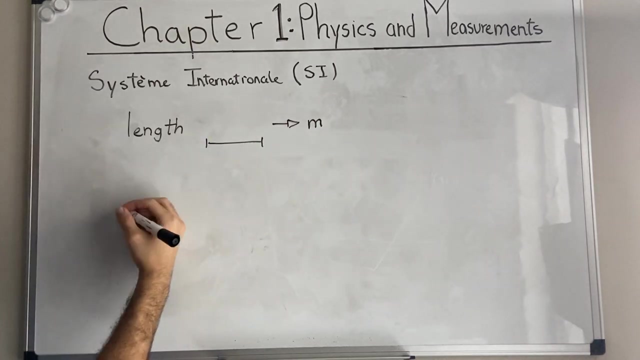 So for length, whenever we talk about length, so, like the distance, distance we're going to be dealing with meters, which we abbreviate with m, Whenever we deal with mass, which is basically the quantity of matter. I guess this is a good like image to show what it is. 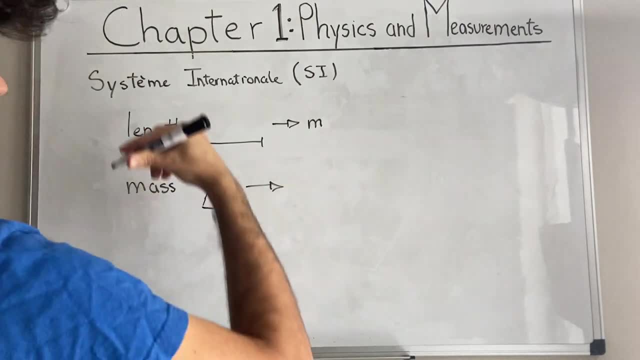 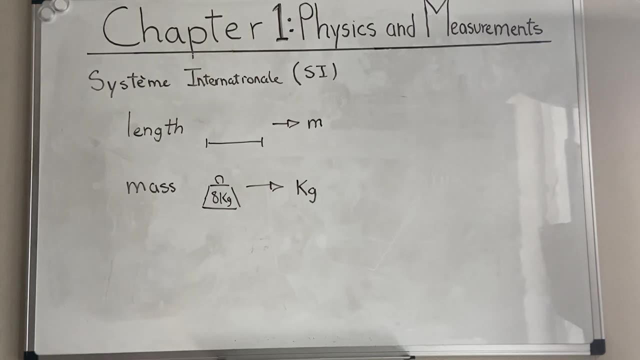 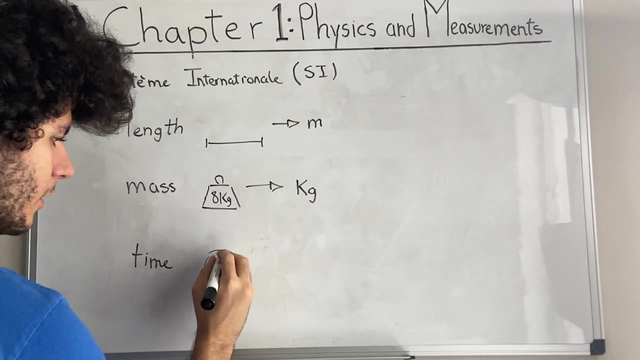 And so whenever we deal with mass- because we're working the SI units- we're going to be dealing with mass, And so we're going to be working with kilograms. And as for time, so I guess I can put a little clock here. 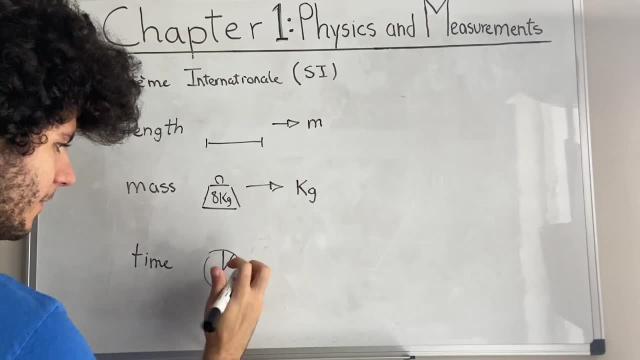 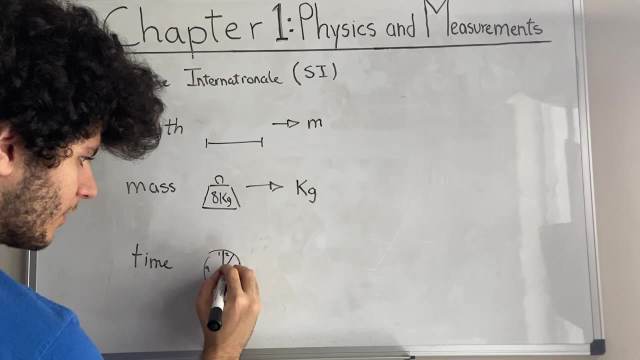 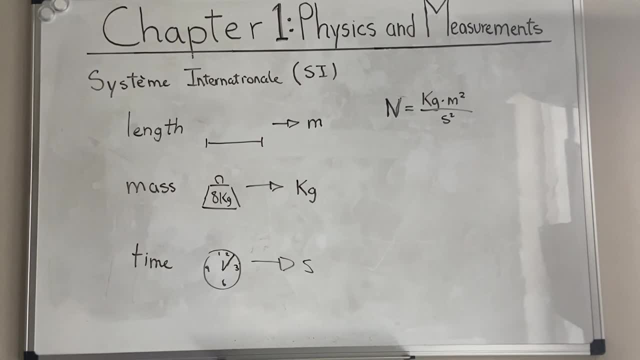 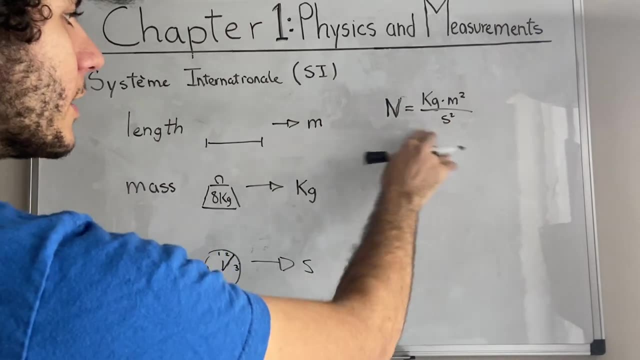 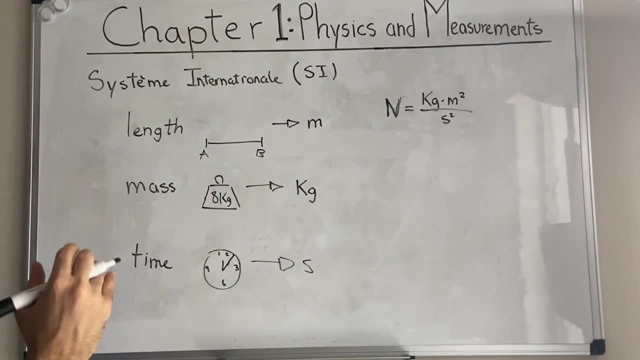 82. period that defines the progression of events from past, present to future. I wanted to give a little bit of a definition, but I'm sure you guys already know what time is. of course, All right, and speaking of unit analysis, let's go right into it. Unit analysis is a method of 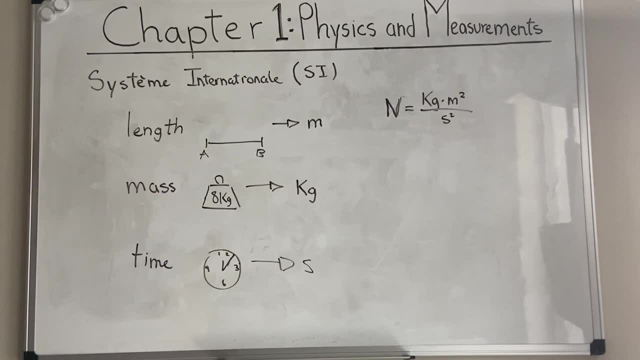 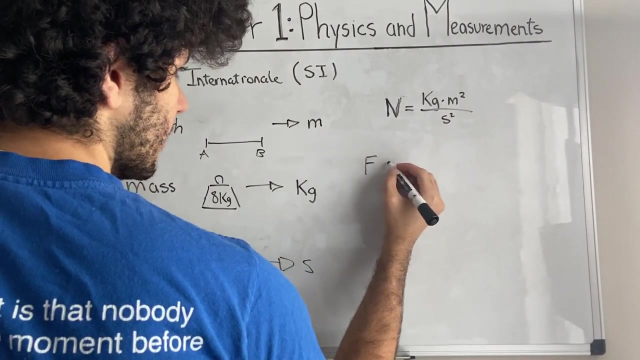 keeping track of units, and it can often serve as a method of checking our calculations. So an example of this is: let's see if we're dealing with, say we're working with. Newton's second law force is equal to mass times acceleration. You're going to see this a lot. 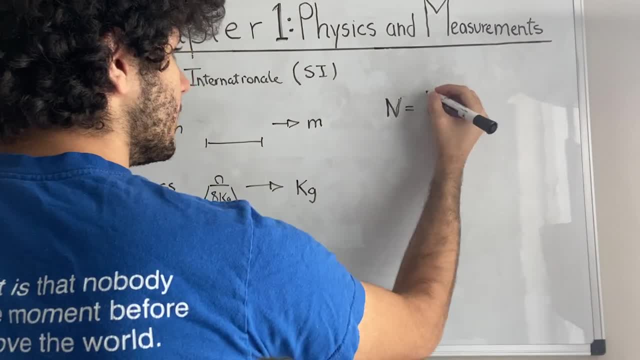 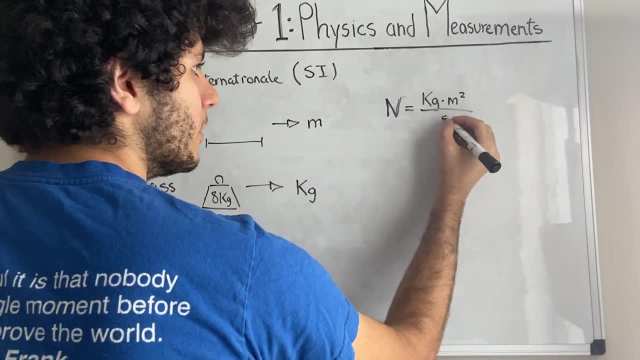 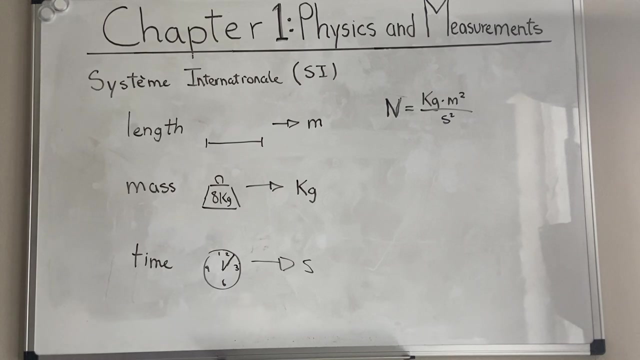 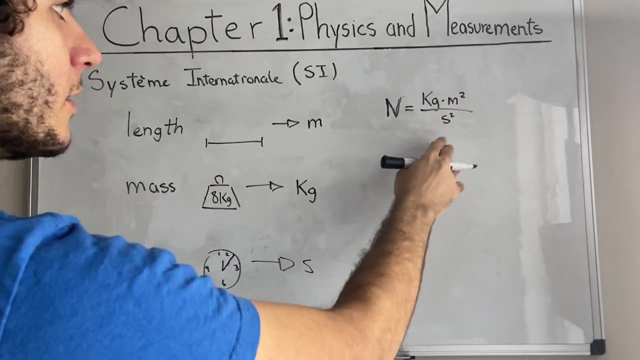 So, for example, Newton can be written as: kilogram times meter squared, over seconds squared. And if you go into the unit analysis, which I'm going to discuss shortly, if you go into the unit analysis, you'll see that you can even prove that this is an existing unit, like conversion or whatever you want to call it. 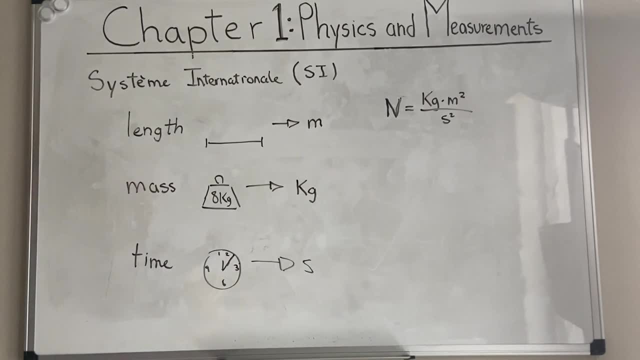 So if you want to define these three base units pretty simply, then we can say: length is the distance between two points in space, A and B. Mass is the measure of the amount of matter in an object Right, And time is a measurable period that defines the progression of events from past, present to future. 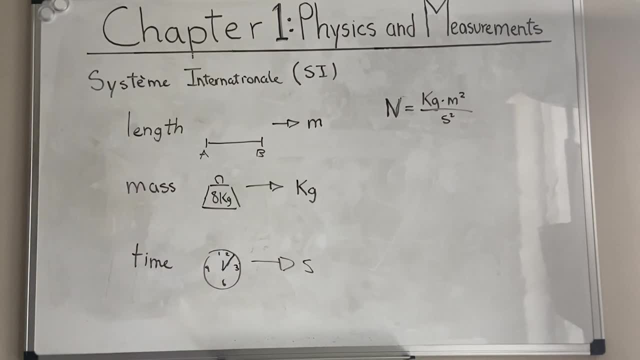 I wanted to give a little bit of a definition, but I'm sure you guys already know what time is, of course, Alright, and speaking of unit analysis, let's go right into it. Unit analysis is a method of keeping track of units and it can often serve as a method of checking our calculations. 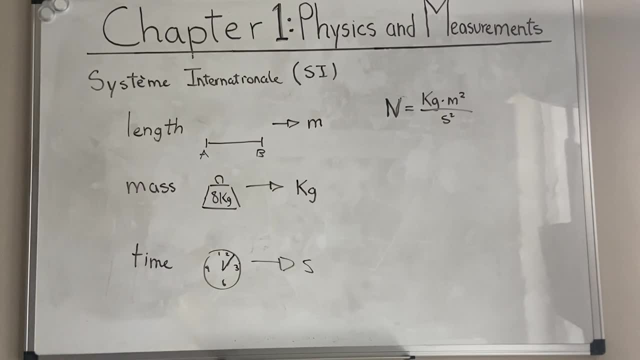 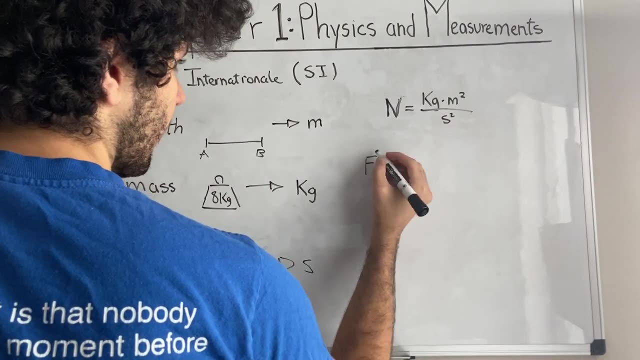 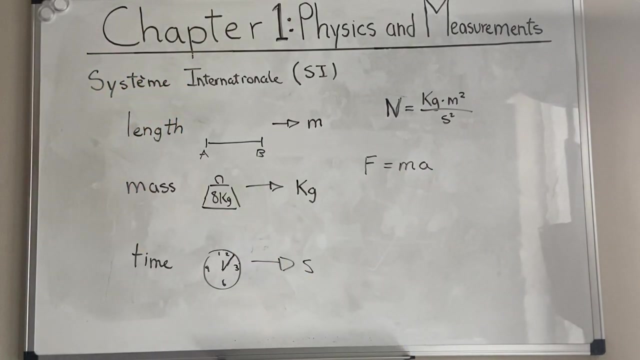 So an example of this is: let's see if we're dealing with, say we're working with, Newton's second law force is equal to mass times acceleration. You're going to see this a lot in your class if you haven't already taken the physics course. 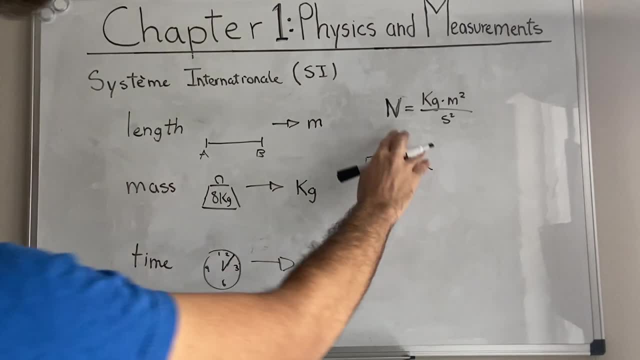 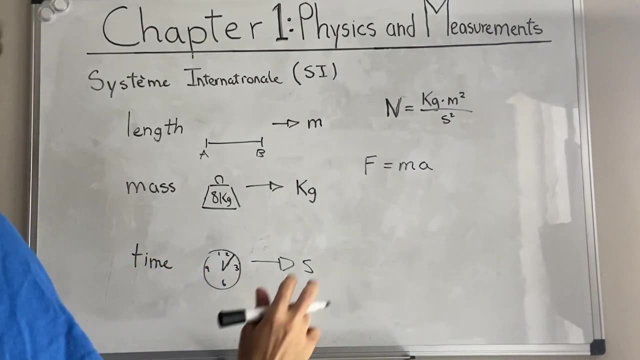 If you want to double check what? if you want to check this, we want to double check that this is, in fact the correct unit conversion- then all we need to do is the unit analysis of this formula, Since force is defined as newtons. 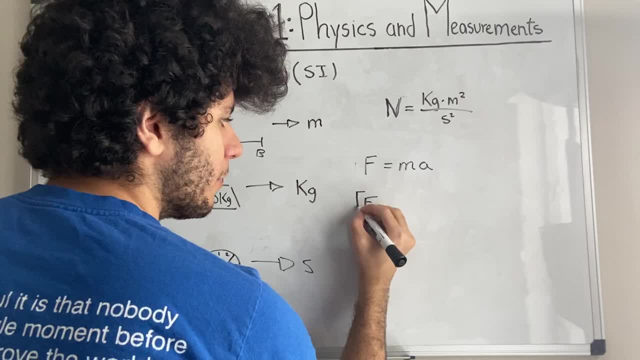 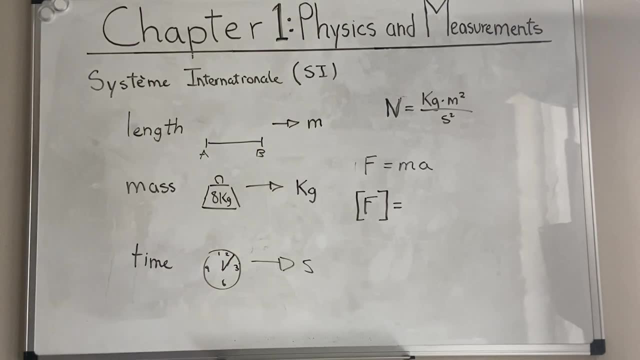 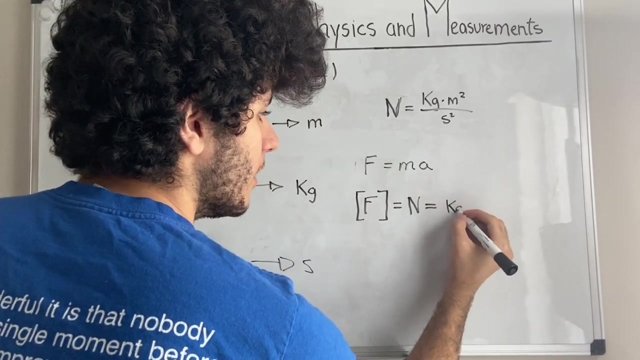 So all we do is we take force, we put these little symbols around it and then we basically break down the units of the formula. So we have newtons on one side equal to what mass, which I just said we can define as kilograms. 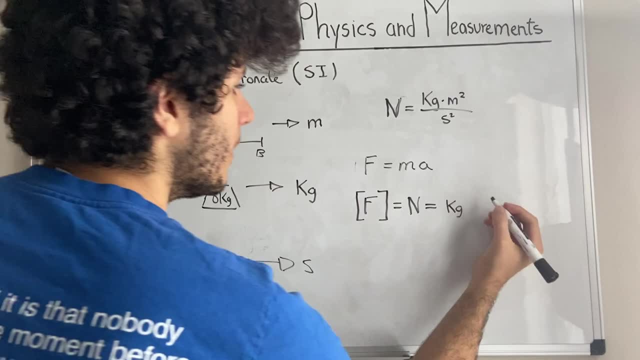 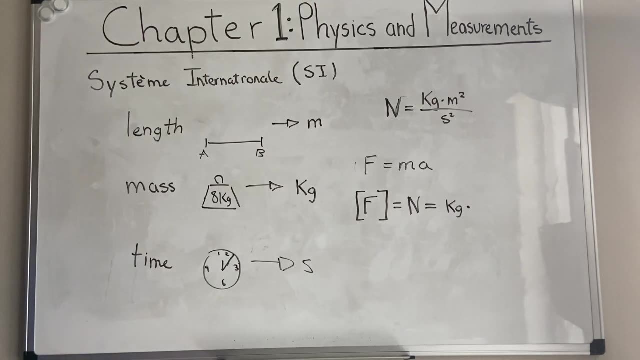 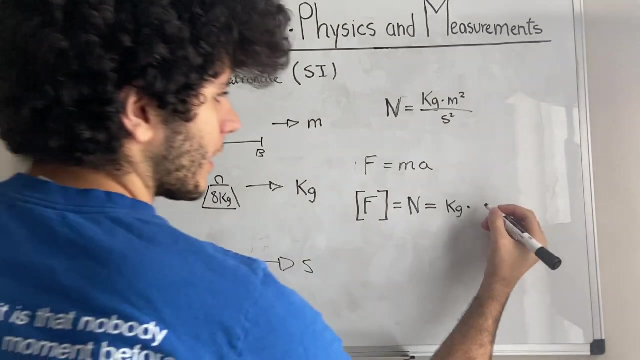 We use kilograms to measure mass times and then we use acceleration And, as we go through this, the many chapters of mechanics. we're going to get used to this. but acceleration is defined as a change of velocity over time. So basically we're going to have velocity. 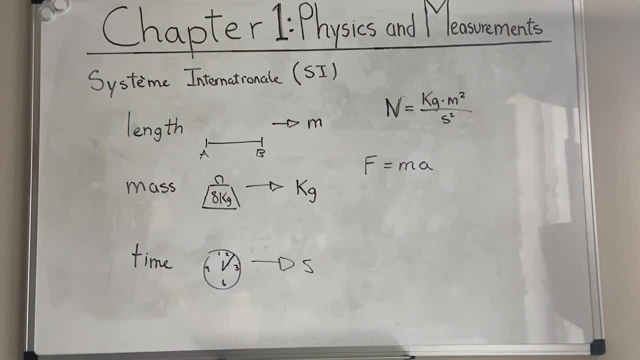 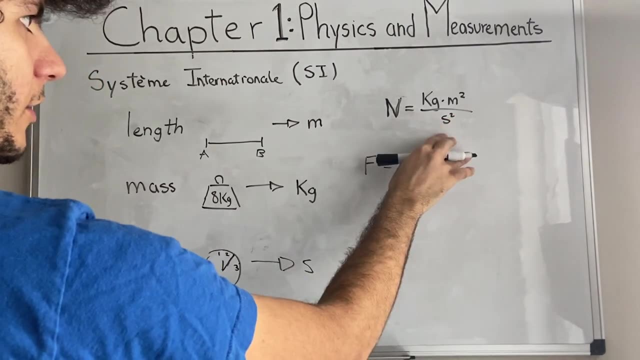 in your class if you haven't already taken the physics course. If you want to double check what? if you want to check this, we want to double check that this is, in fact, the correct unit conversion- then all we need to do is: 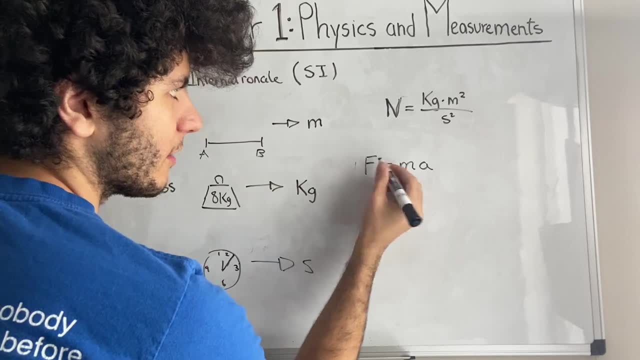 you're going to have to do a little bit of a math test. So if you want to double check the unit conversion, then all we need to do is you're going to have to do a little bit of a math test, unit analysis of this formula, since force is defined as newtons. So all we do is we take force. 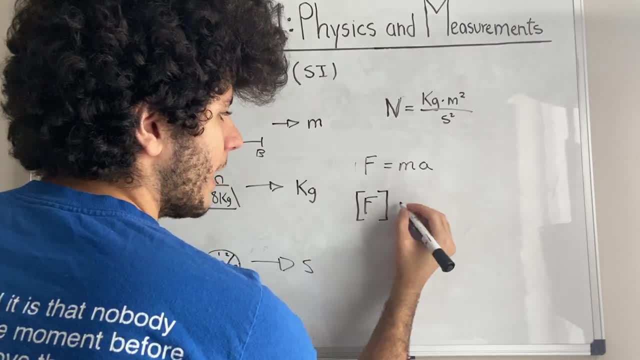 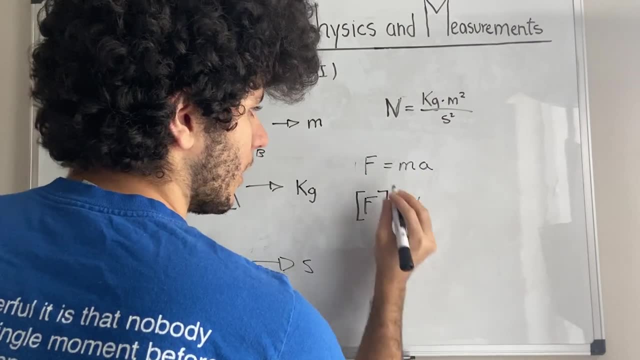 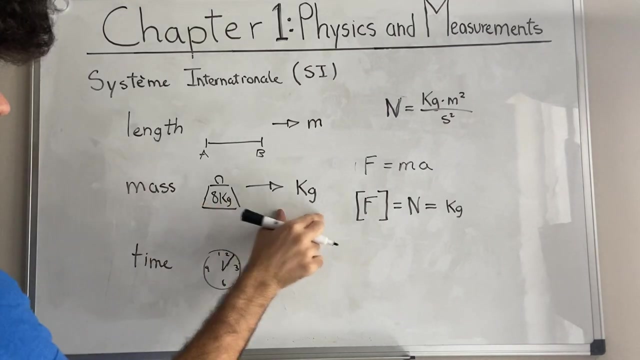 we put these little symbols around it and then we basically break down the units of the formula. So we have newtons on one side, equal to what mass, which I just said we can define as kilograms. We use kilograms to measure mass. 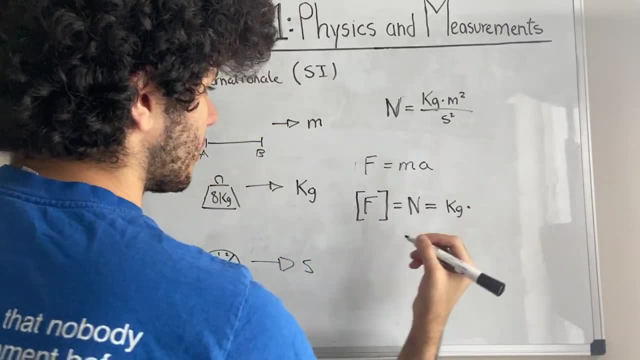 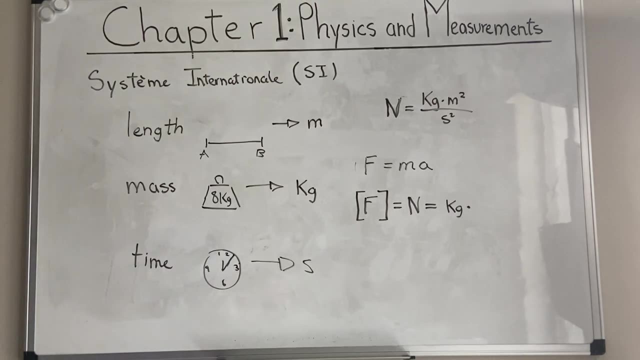 times acceleration And, as we go through this, the many chapters of mechanics. we're going to get used to this. but acceleration is defined as a change of velocity over time. So basically we're going to have velocity which is- I guess you could call it- speed. 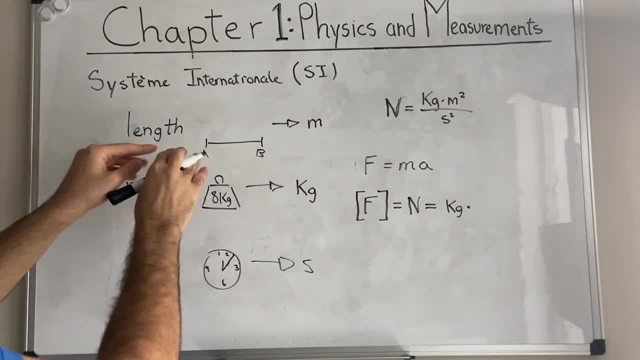 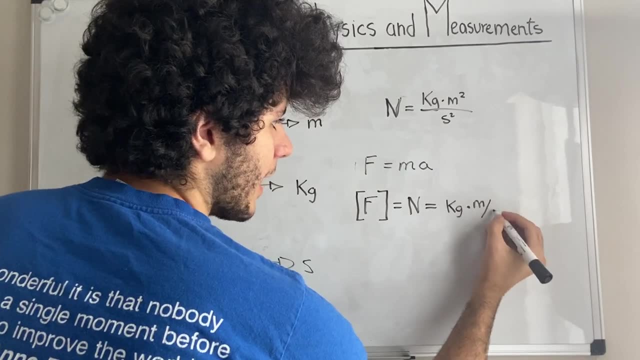 now that we're just like warming ourselves up. So which is basically mass length over time, a distance over time, and then we're going to add another s to it which makes it squared. Maybe it's a little bit complicated As we get into the review. 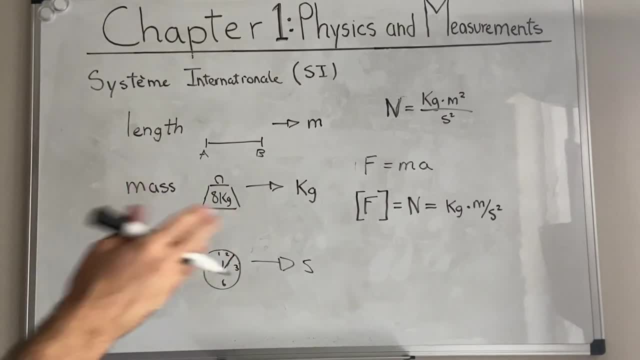 you'll probably understand it a little bit better. So that's that, And, as you see, these match. They're written a little bit differently, but they are equal. Therefore, we have, we found a method of double checking our units And we call this: 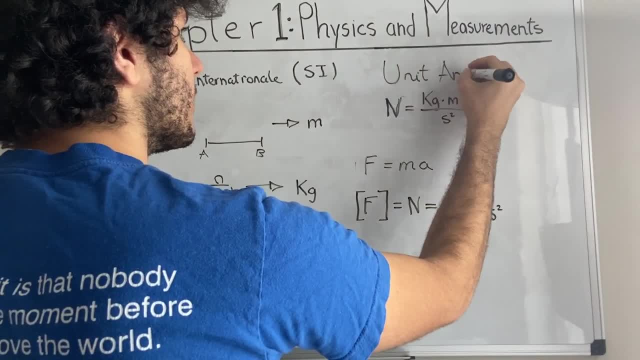 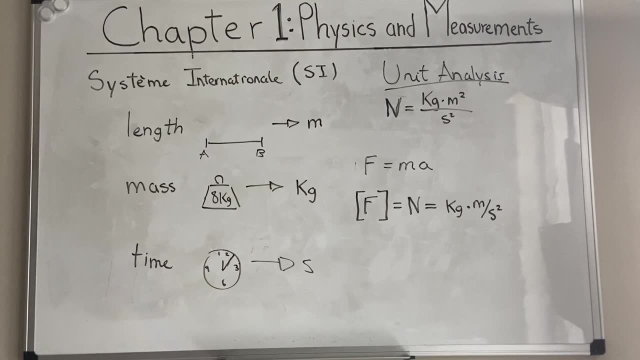 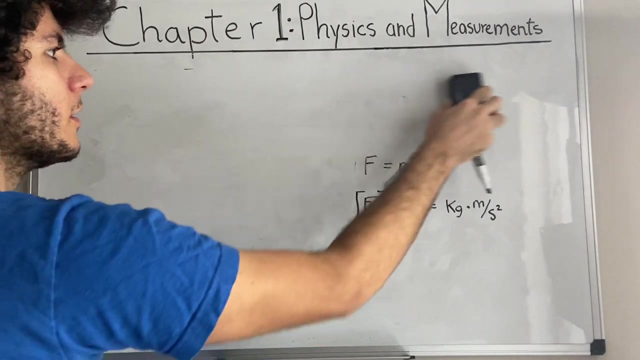 unit analysis. All right, All right. Next, we can maybe do a little very, very, very simple problem regarding conversions. So basically taking one unit or finding an answer and then changing that answer from one unit to another. 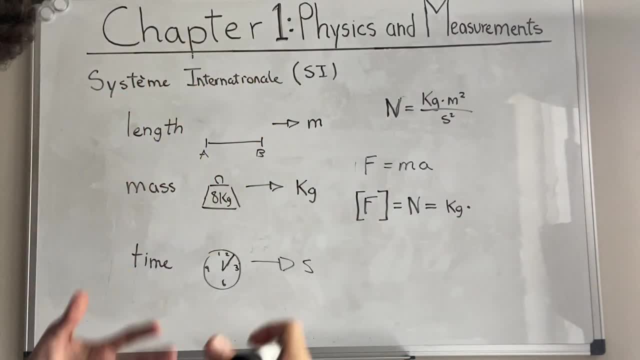 which is- I guess you could call it- speed, now that we're just like warming ourselves up, So which is basically length over time, A distance over time, And then we're going to add another s to it, which makes it squared. 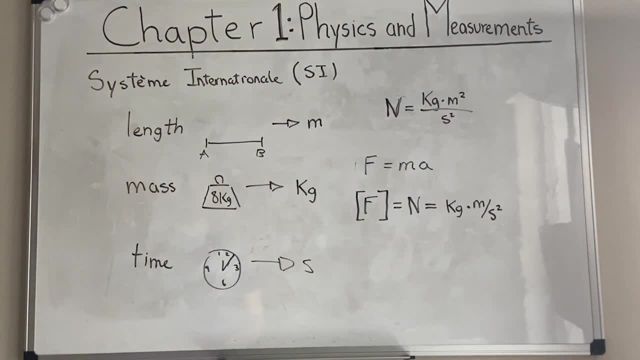 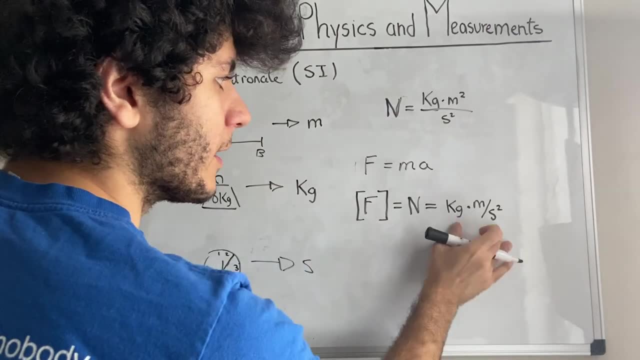 Maybe it's a little bit complicated. As we get into the review you'll probably understand it a little bit better. So that's that, And, as you see, these match. They're written a little bit differently but they are equal. 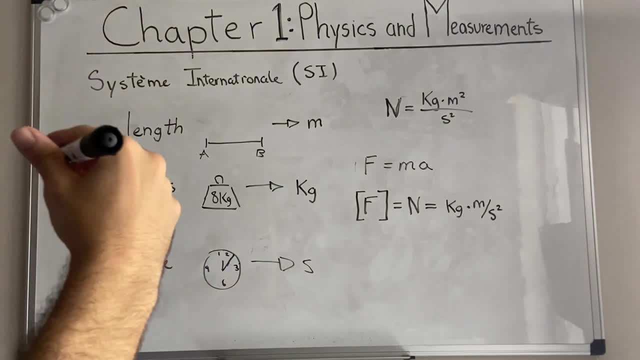 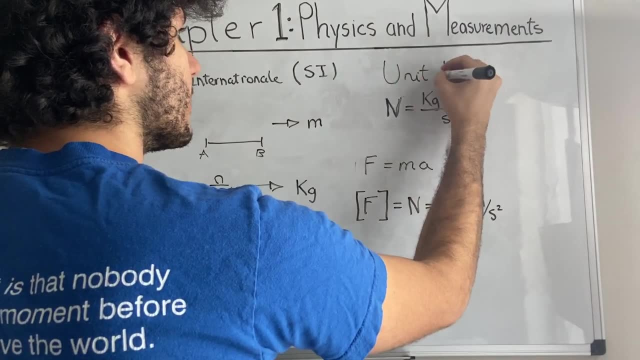 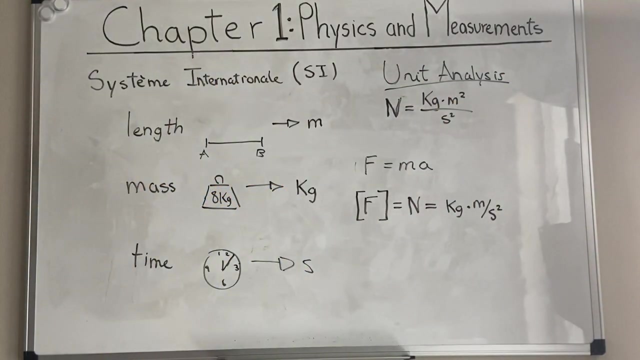 Therefore we have, we found a method of double-checking our units And we call this unit analysis. All right, All right. Next, we can maybe do a little: very, very, very simple problem regarding conversions. So, basically taking one unit, 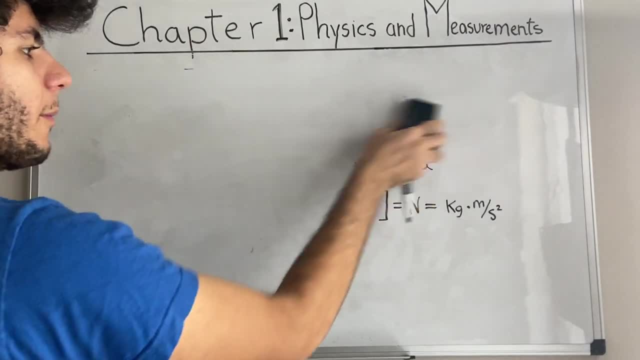 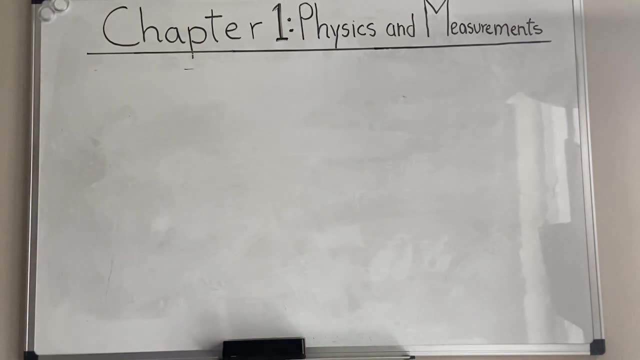 we're finding an answer and then changing that answer from one unit to another, Because you can measure length, mass, time in different ways. You can say 60 seconds ago something happened, Or you can say one minute ago something happened. 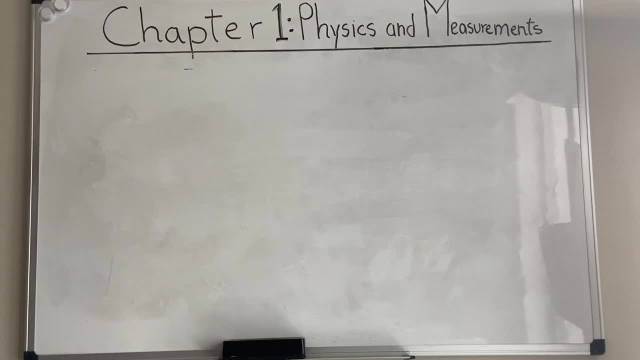 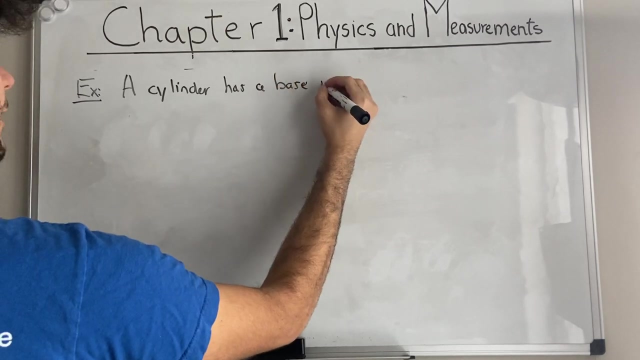 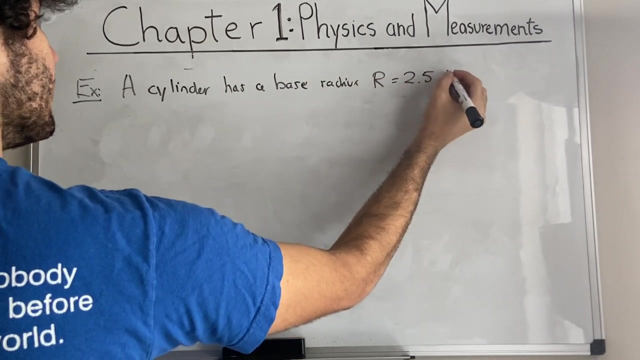 There are many different ways of quantifying measurements, Or there's many different units that we can use to measure anything, basically. So in this example, I am asking you to calculate the volume of a cylinder. Here's the context: A cylinder has a base radius r which is equal to 2.5 feet. 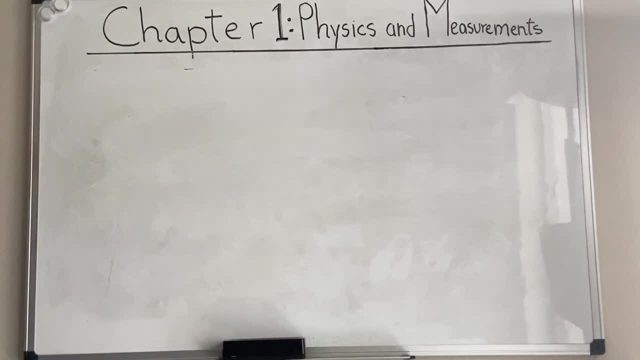 Because you can measure length, mass, time in different ways. You can say 60 seconds ago something happened, or you can say one minute ago something happened. There are many different ways of quantifying measurements. There's many different units that we can use to measure. 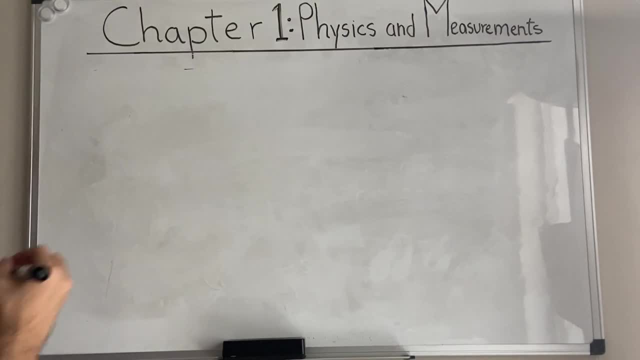 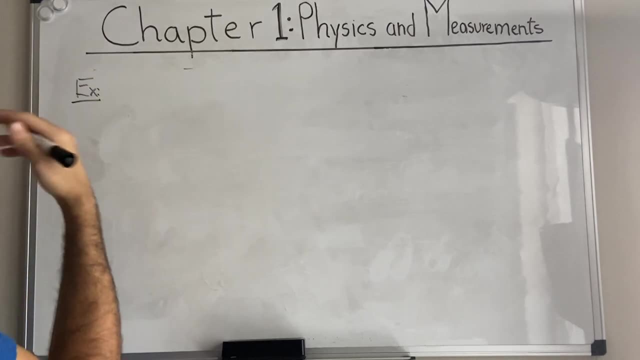 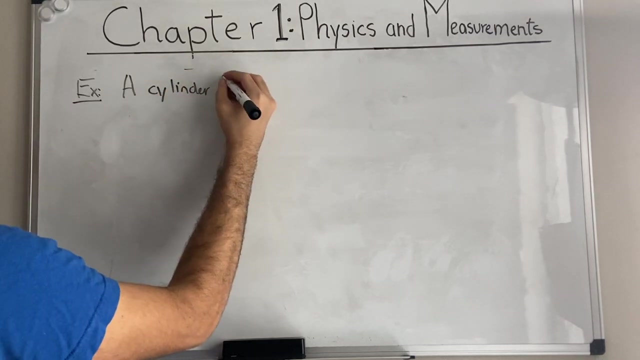 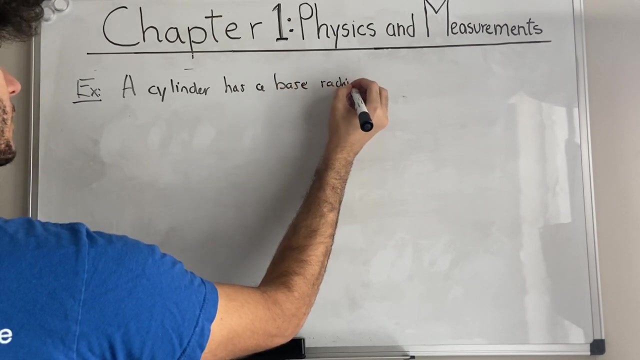 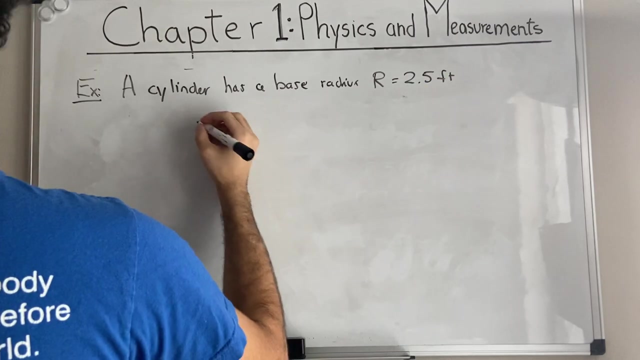 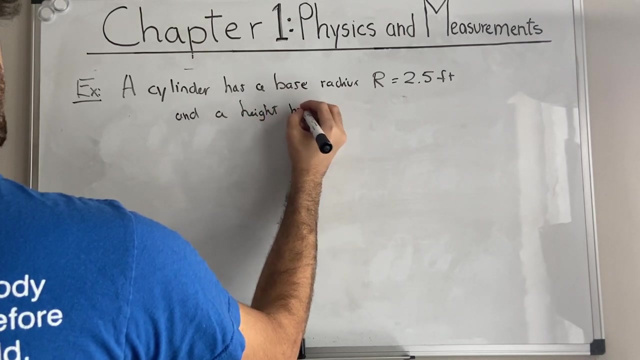 anything, basically. So in this example, I am asking you to calculate the volume of a cylinder. Here's the context: A cylinder has a base radius r which is equal to 2.5 feet and a height of h equal to 6 feet. 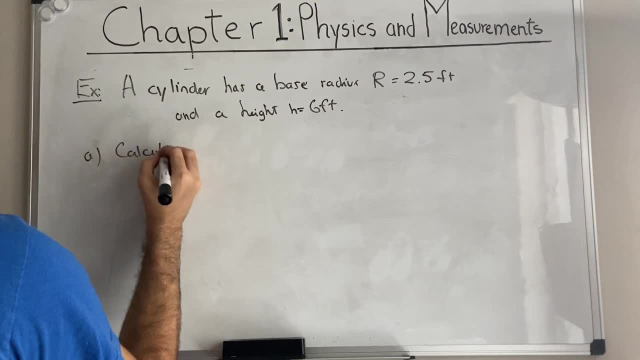 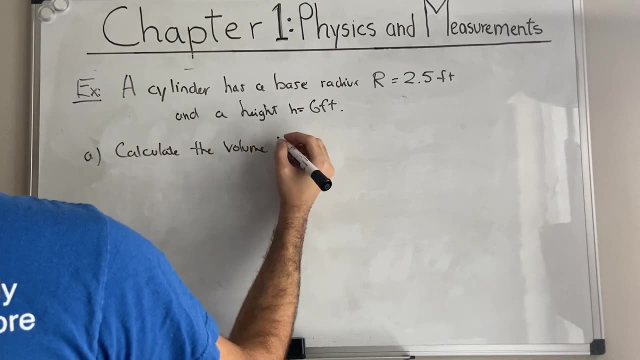 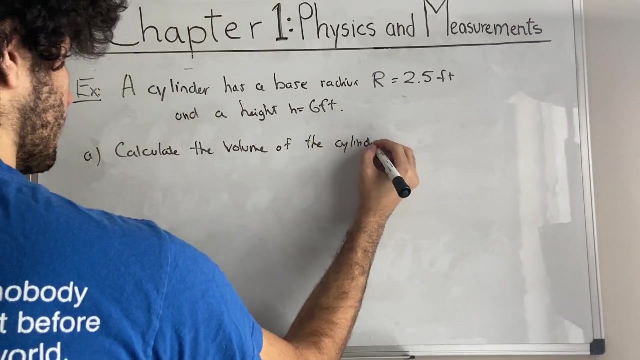 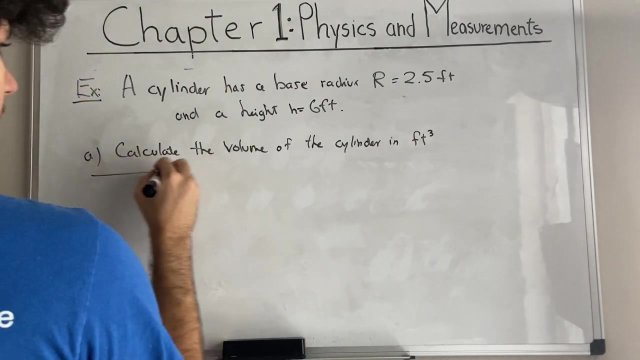 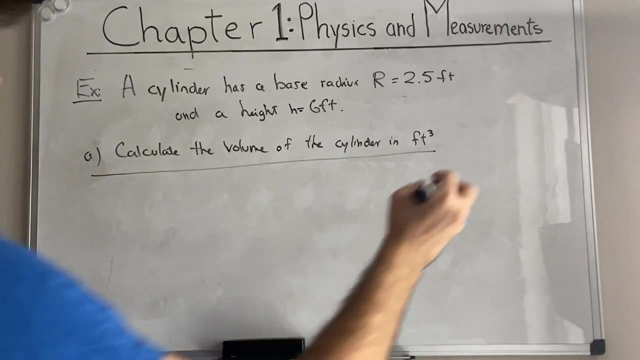 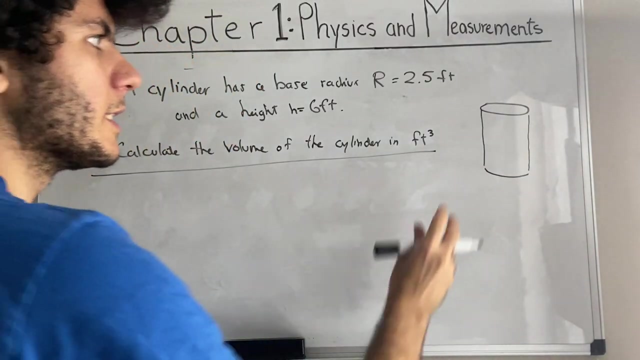 Question A is asking to calculate the volume, The volume of the cylinder in cubic feet. okay, so basically, if you remember what the formula for the volume of a cylinder is, it's pretty simple actually. it's basically the area of the base. I can write it over here. 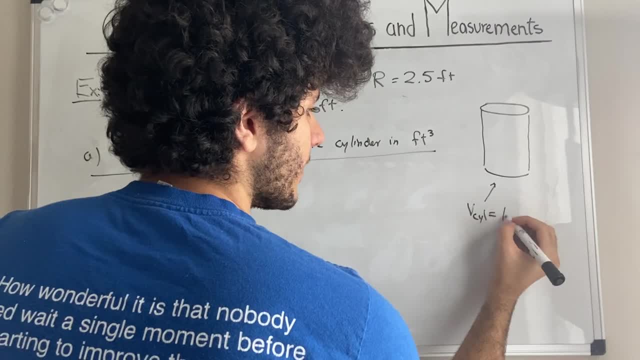 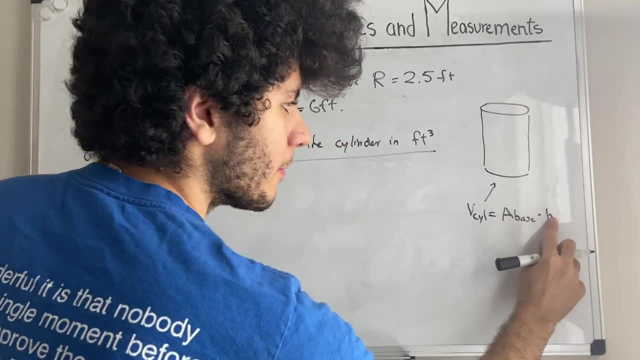 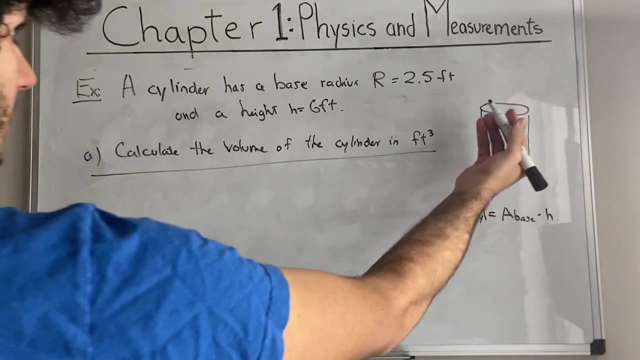 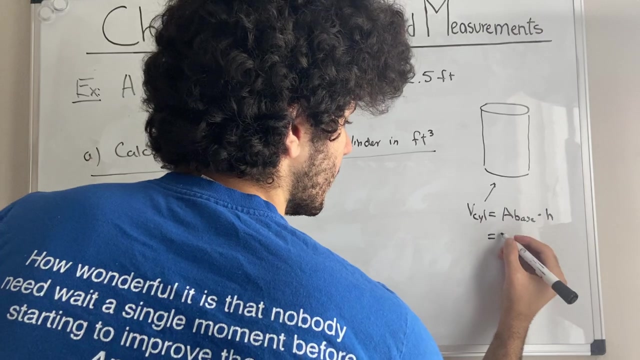 volume of the cylinder is equal to the area of the base times the height. confuse that with a B: area of the base times the height, and so if you think about what the area of the base is, well, basically we have a circle over here. so it's basically pi? r squared times h, and what do you? 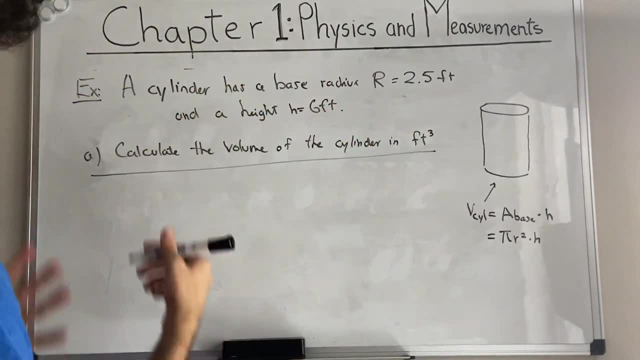 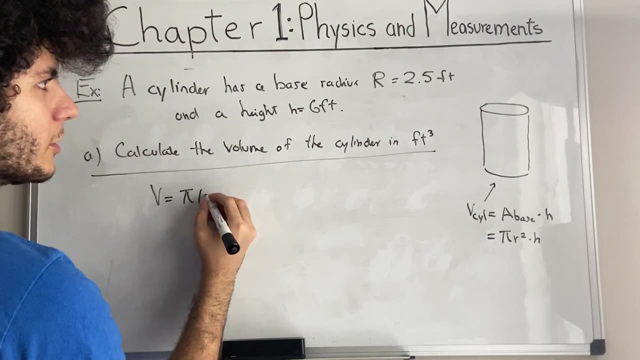 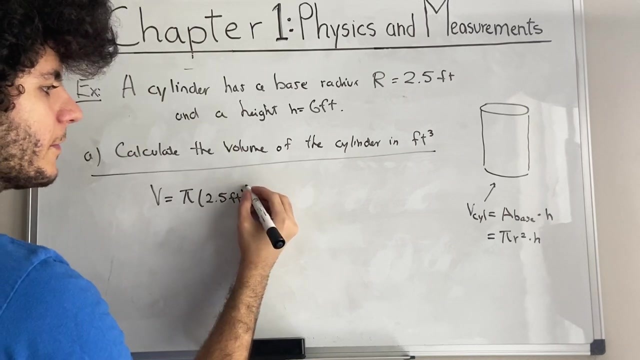 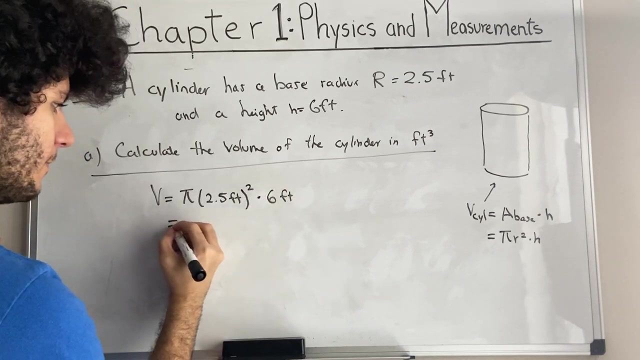 know we have radius and we have height. therefore we can just plug in our numbers. I are, which is 2.5 feet for this example, I'm going to write the units inside the formula squared times height, which is 6 feet. all right, and if we plug, 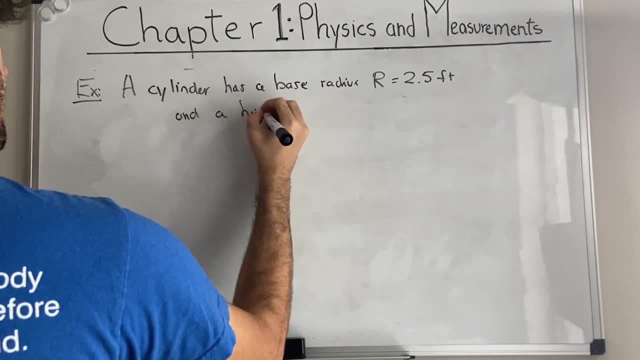 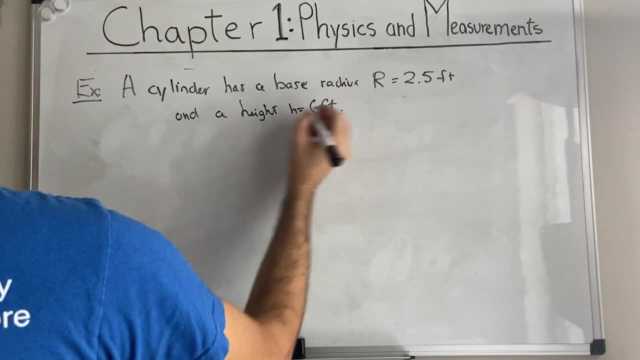 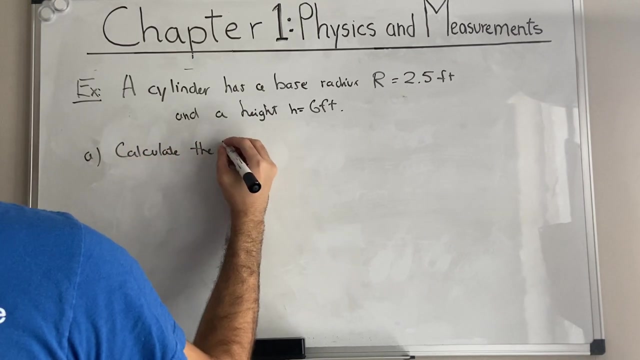 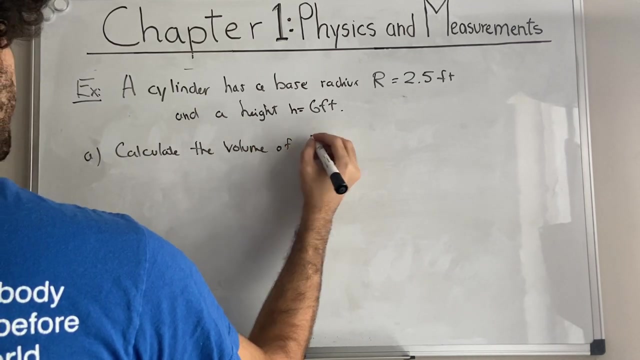 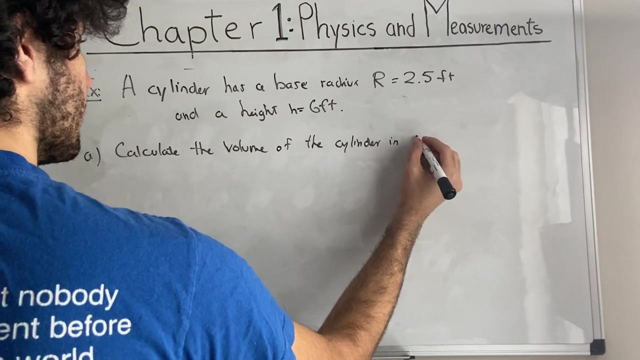 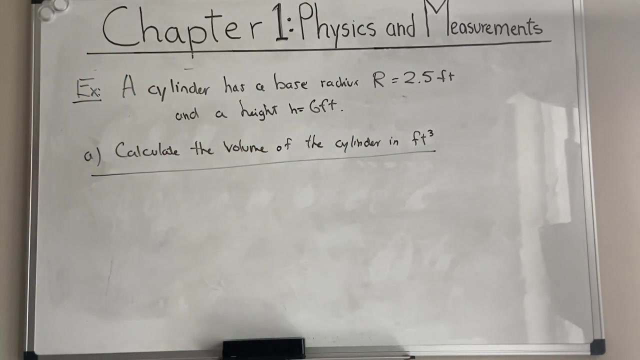 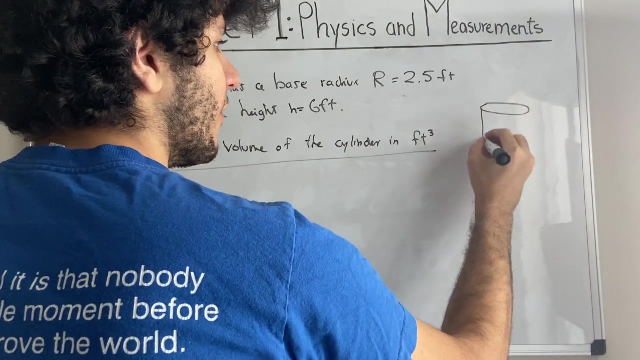 And a height of h is equal to 6 feet. Question A is asking to calculate the volume, The volume of the cylinder in cubic feet. Okay, So basically, if you remember what the formula for the volume of a cylinder is, it's pretty sad, simple actually. 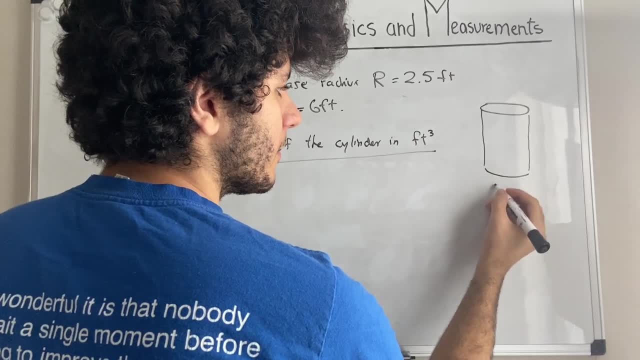 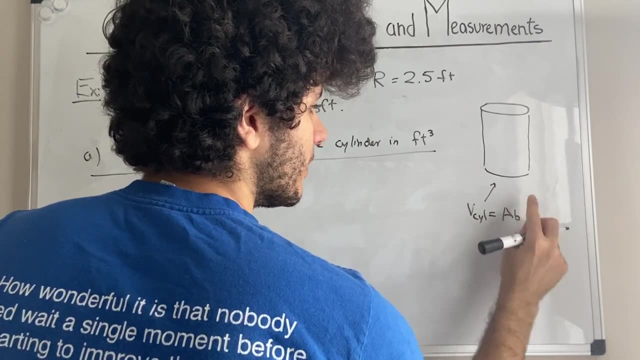 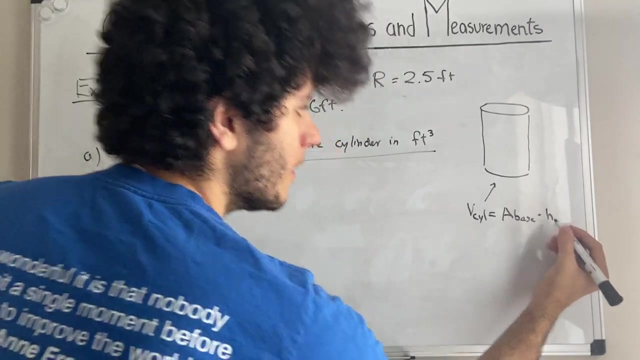 It's basically the area of the base. I can write it over here: Volume of the cylinder is equal to the area of the base times the height. let me not confuse that with a, b area of the base times the height. And so if you think about what, 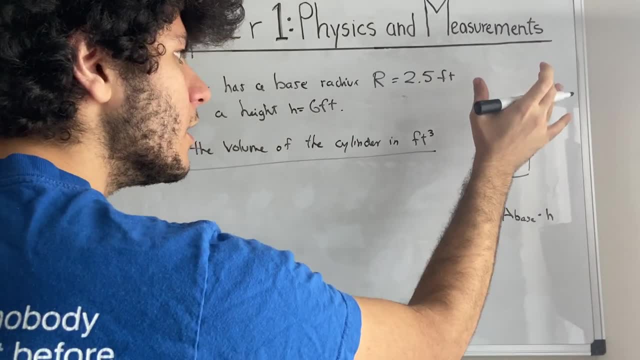 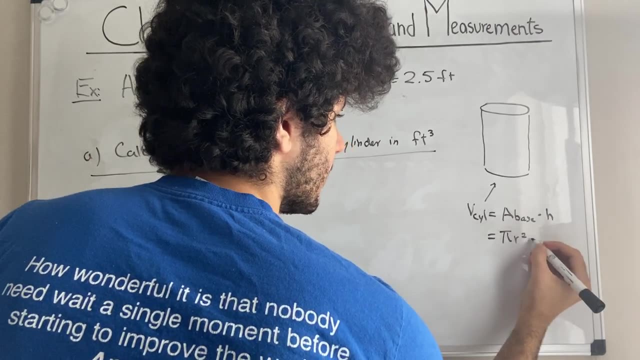 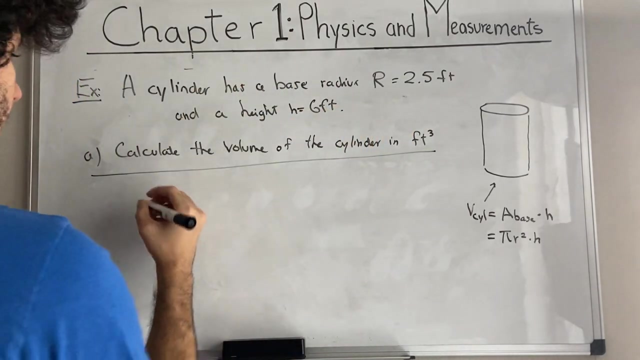 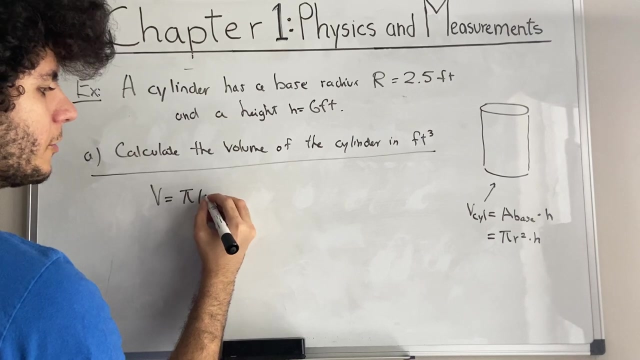 the area of the base is. well, basically, we have a circle over here, So it's basically pi r squared times h. And what do you know? We have radius and we have height. Therefore, we can just plug in our numbers Pi r, which is 2.5 feet For this example. I'm going to write the units inside the formula. 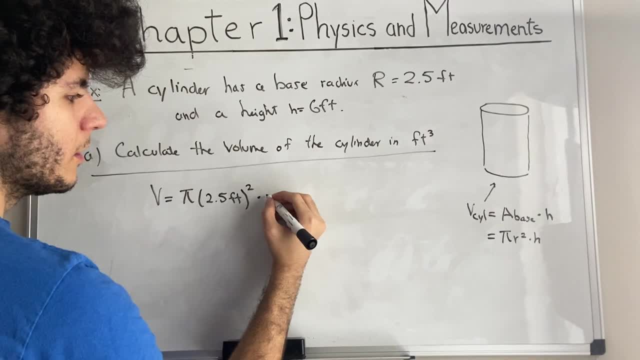 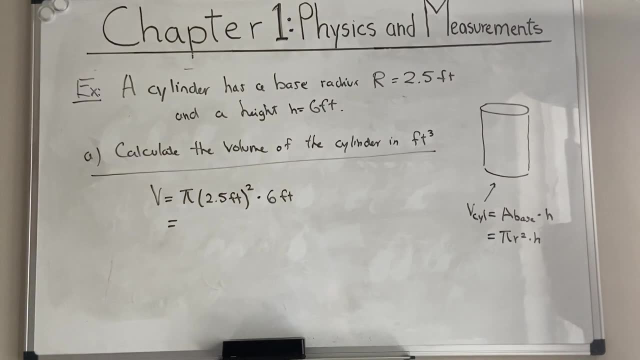 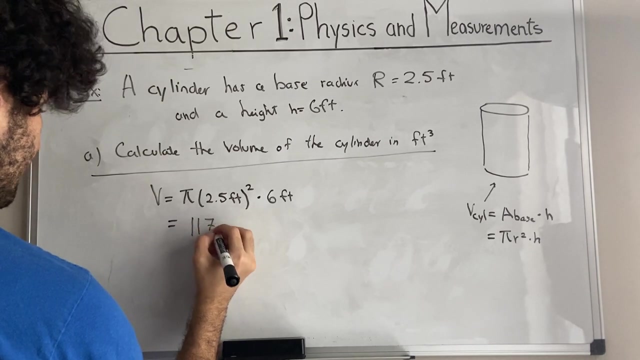 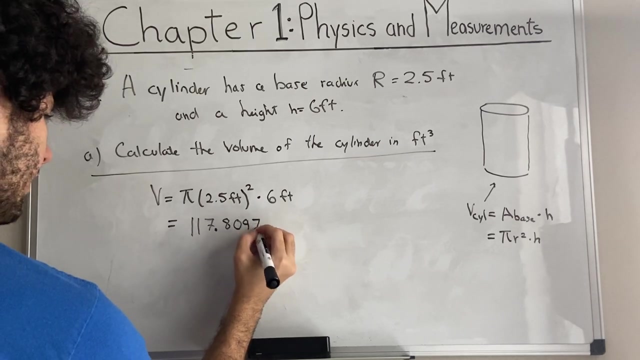 Square times height, which is 6 feet, All right. And if we plug that really quickly into our calculator, we will see pi times 2.5.. 5 squared times 6 is equal to 117.8097245.. I added a lot, of a lot of decimals, which is not. 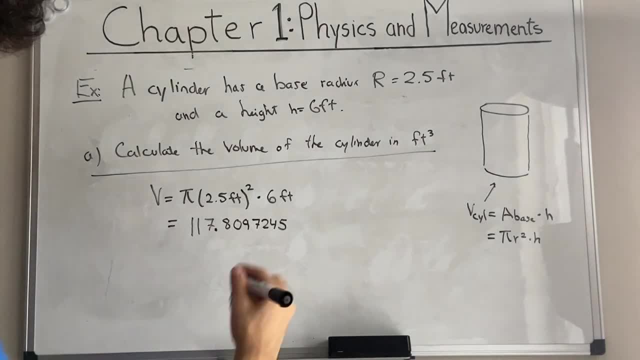 necessary, But ask your professor about it. Some professors have different standards. We're not working with significant figures over here. We'll only work with significant figures in labs. So what about the units though? They're asking for feet cubed. Well, here we have feet. 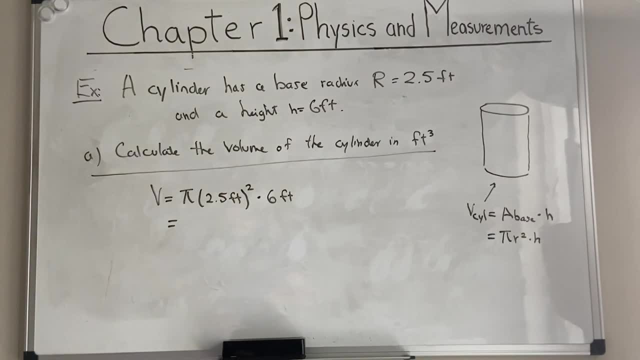 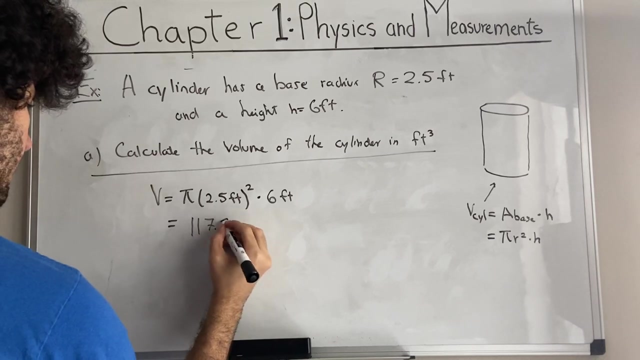 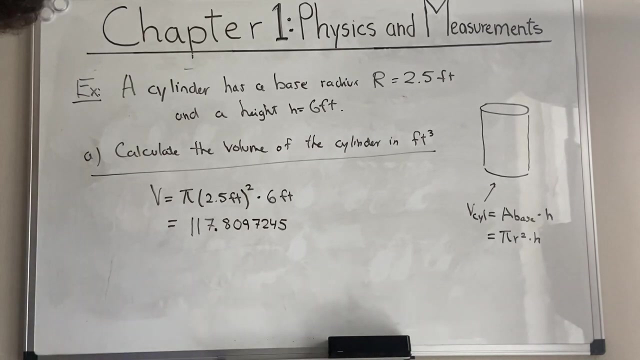 that really quickly into our calculator. we will see: pi times 2.5 squared times 6 is equal to 117.8097245. I added a lot of a lot of decimals, which is not necessary, but ask your professor about it. some professors are different standards. we're. 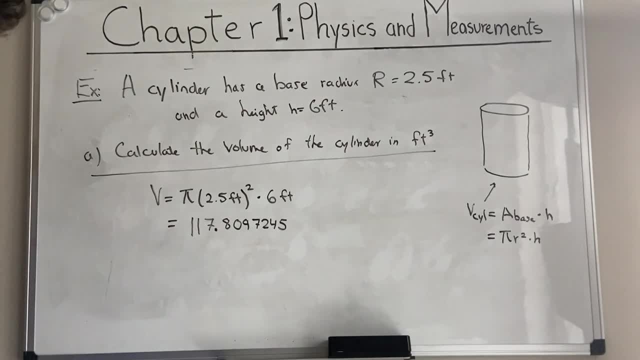 not working with significant figures over here, only work with significant figures in labs. so what about the the units, though? they're asking for feet cubed. well, here we have feet squared times feet, and what do you know? that's feet cubed. wow, that's great. okay, so we have our answer. now the next question is: 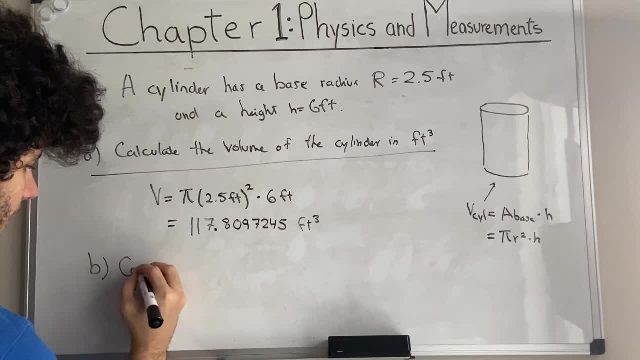 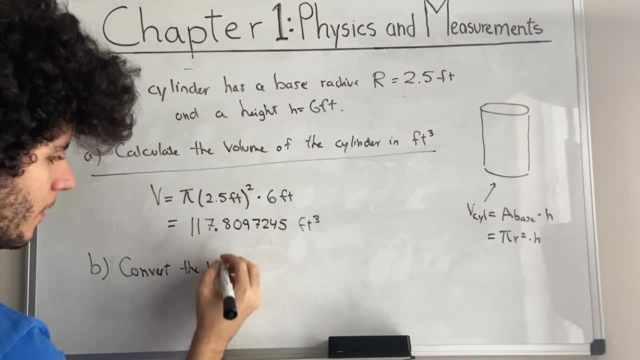 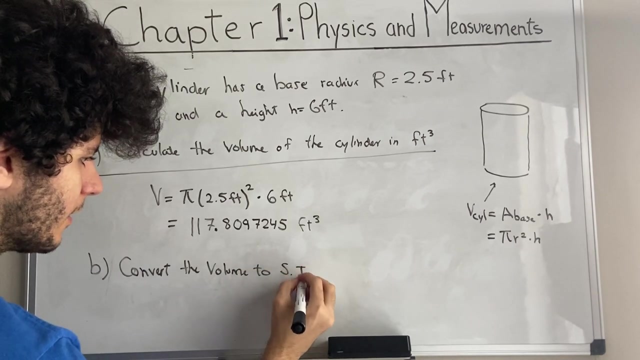 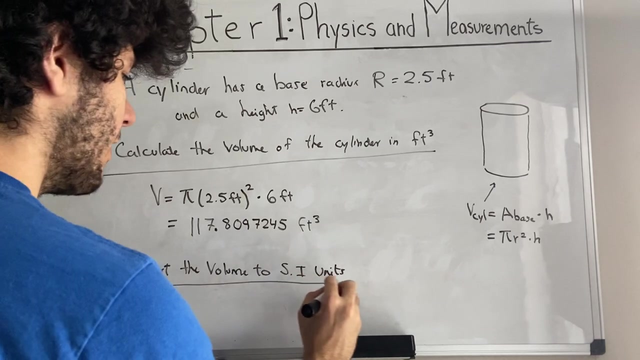 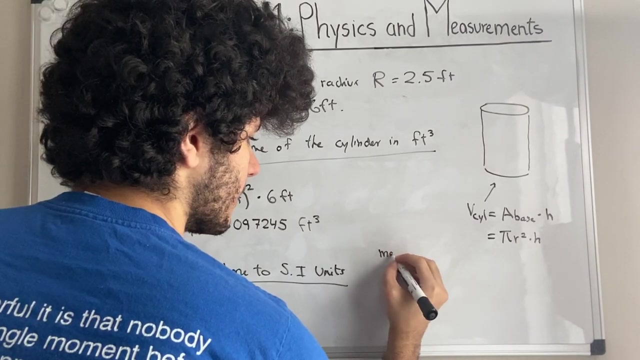 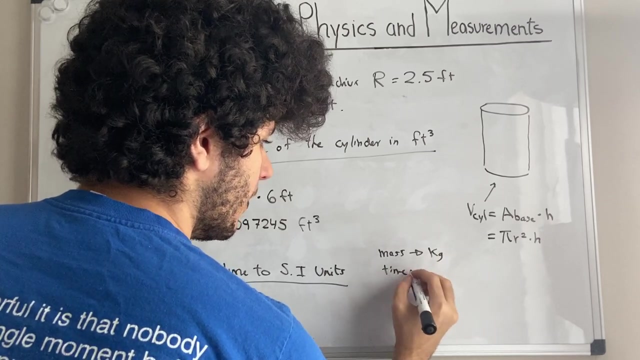 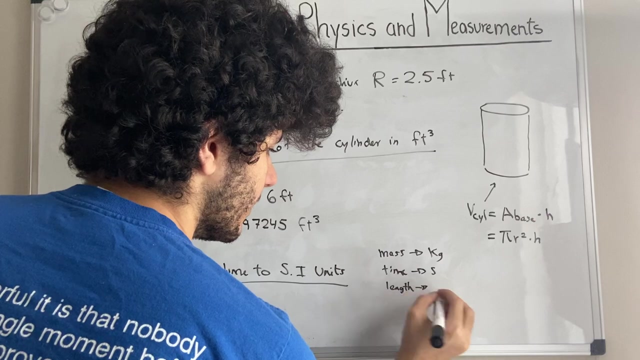 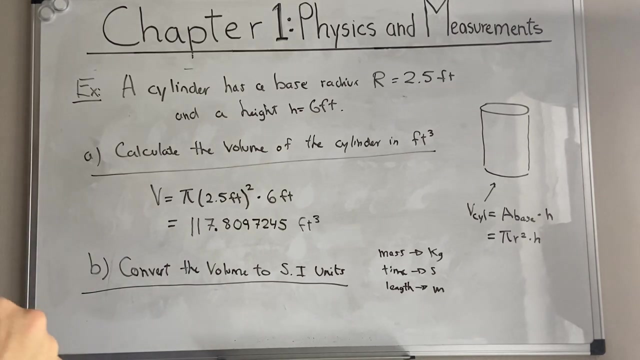 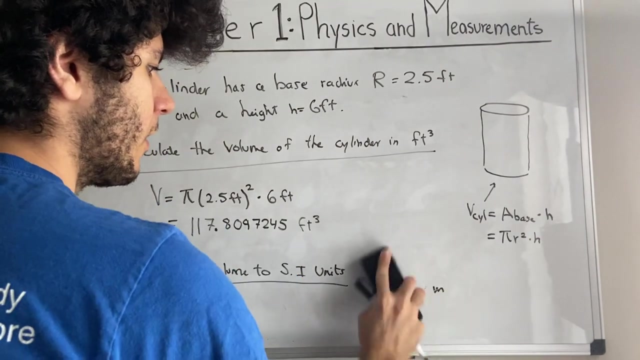 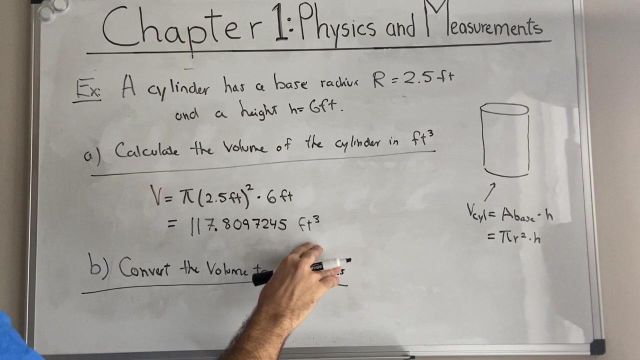 asking us to convert, convert the volume to SI units, the volume to SI units. and so we- this is finally like an application of what we just went over. what would do? what do we remember? we remember that mass, mass, mass mass. we're going to end up with the alternative to feet cubed, which in SI units would be. 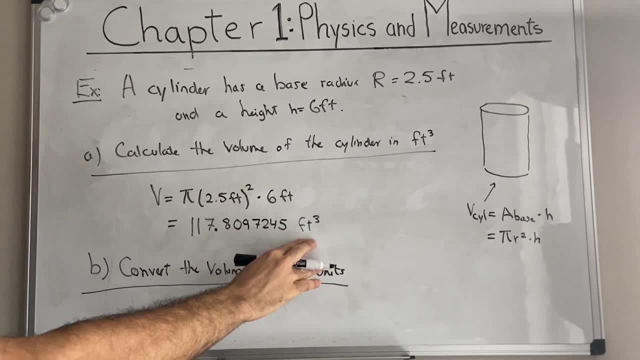 meters cubed, then we need to find the conversion ratio between feet and meters. so I'm actually going to just look that up. I'm not very used to using feet, feet, two meters, so in one foot we have 0.3048 meters, and then we're going to find the conversion ratio between feet. 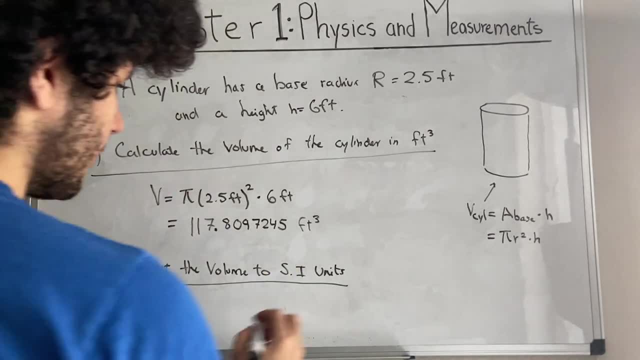 and meters, so I'm actually going to just look that up. I'm not very used to using feet, feet, and that could have been written in the other way too, but we're going to work with it in this way because that's what first came up on the internet: one foot. 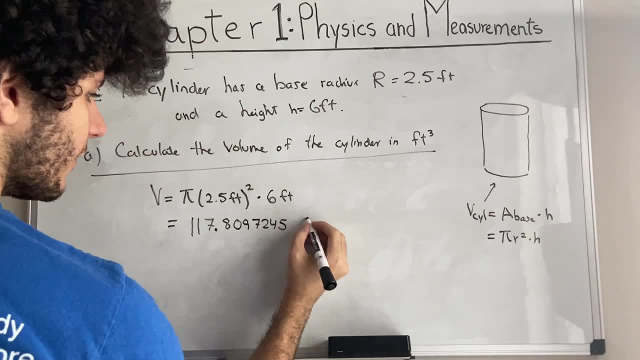 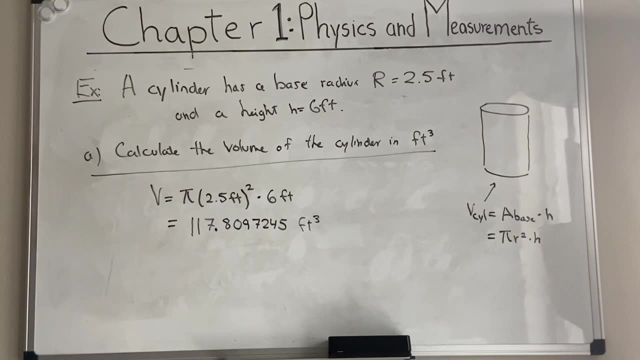 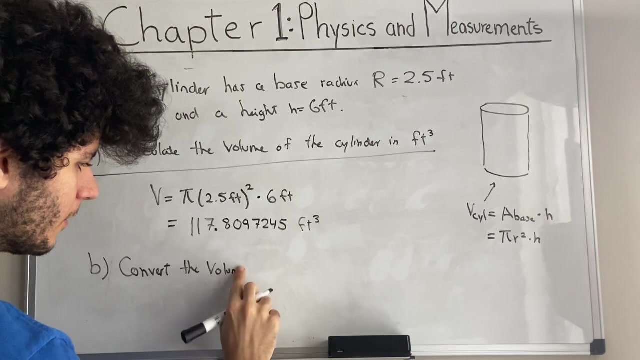 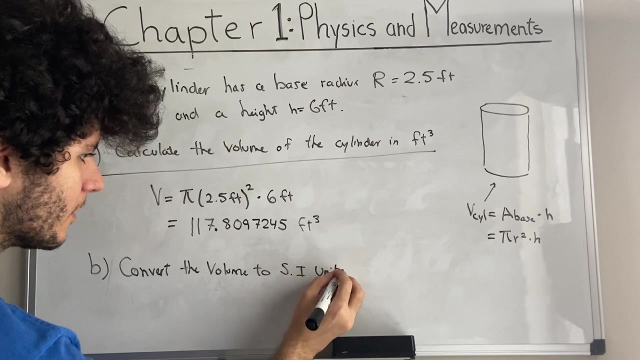 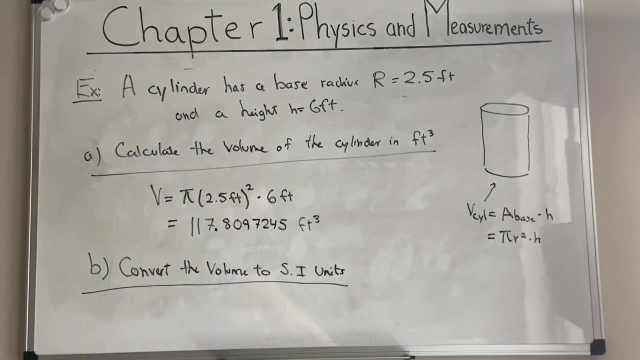 squared times, feet, And what do you know? That's feet cubed. Wow, that's great. Okay, so we have our answer. Now the next question is asking us to convert. convert the volume to SI units, The volume To SI units. And so we- this is finally like an application of what we just went over. What do we? 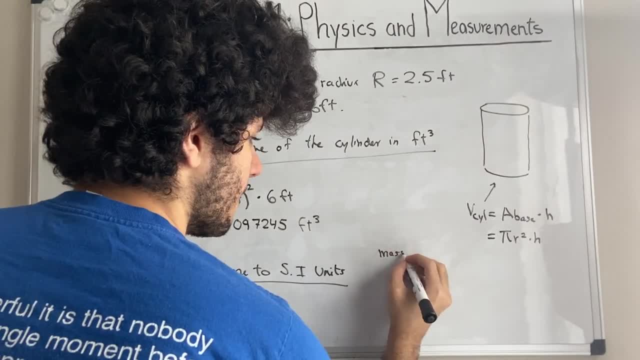 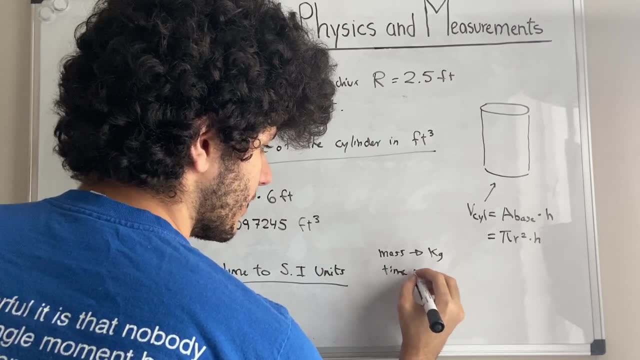 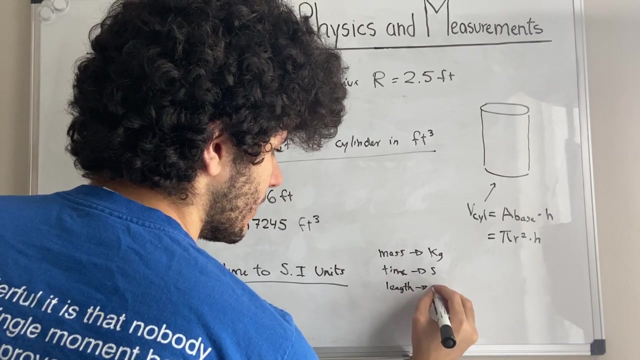 remember. We remember that mass, its SI unit is the kilogram, We know that times, that the SI unit for time is seconds, And we know that the mass is the kilogram. And we know that the mass is the unit for length is a meter. It's just like a little reminder. So the way that we're going to 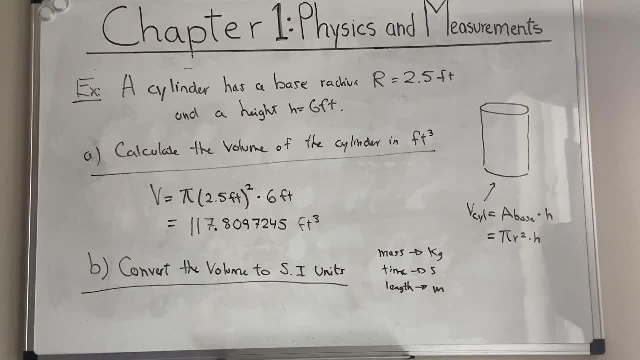 convert. this is by using conversion ratios. So if we know that we have feet cubed and we want to end up with the alternative to feet cubed, which in SI units would be meters cubed, then we want to find the conversion ratio between feet and meters. So I'm actually going to just look that up. I'm not very. 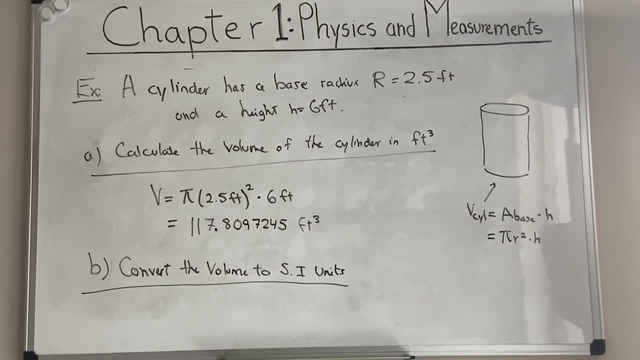 used to using feet, Feet to meters, So in one foot we have 0.3048 meters, And that could have been written in the other way too, But we're going to work with it in this way because that's what first. 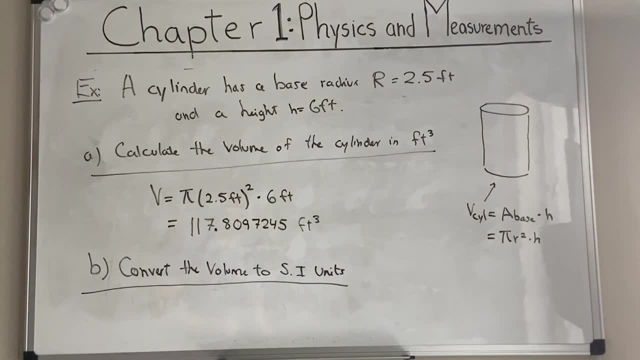 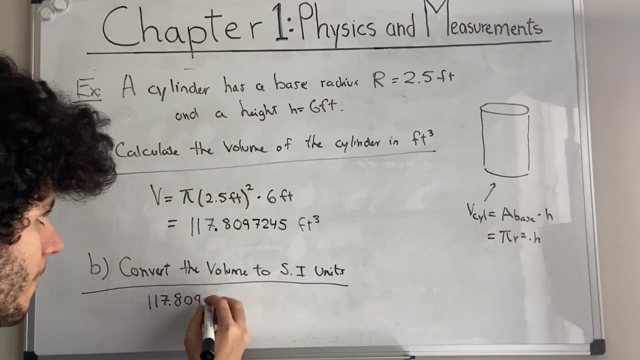 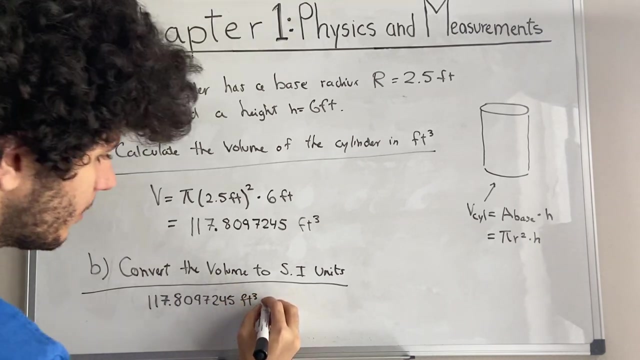 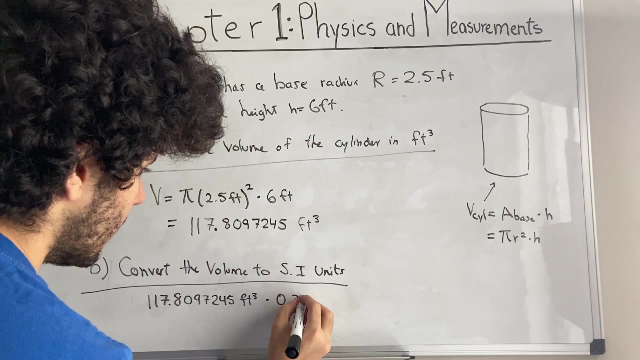 came up on the internet: 0.3048.. So we take our result. Let's see if you guys can see. Yeah, it's pretty visible: 7245 feet cubed times. oh, what was it? 0.3.. We want meters to be equal to meters, So we're going to. 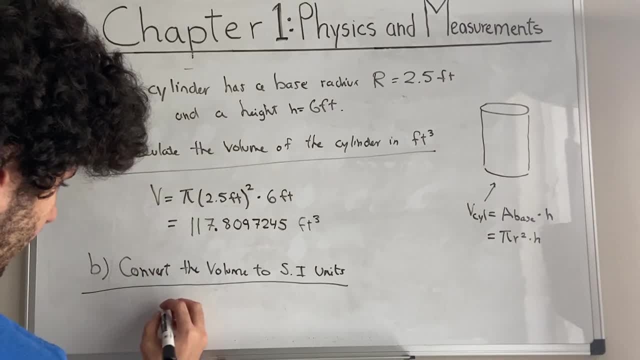 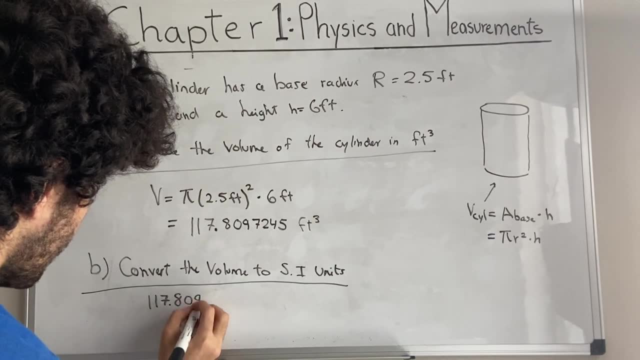 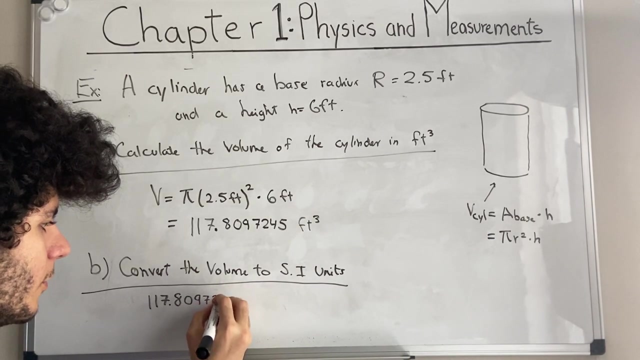 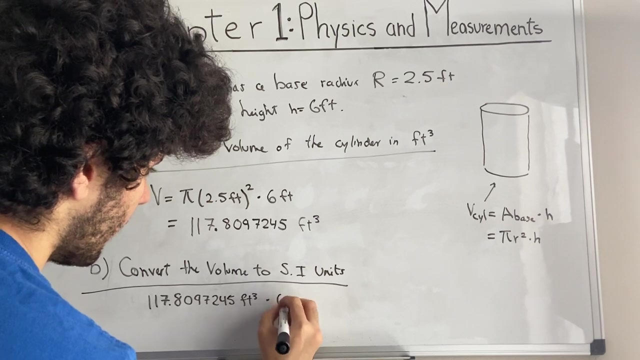 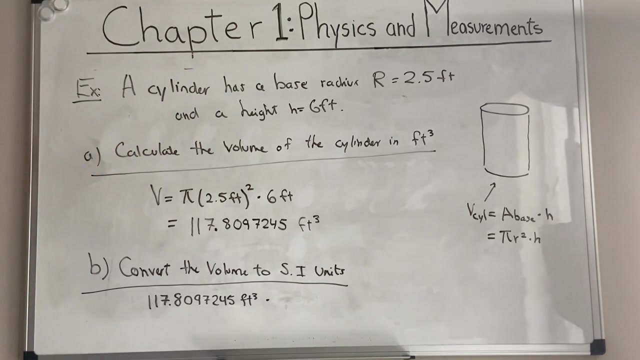 zero point three, zero four, eight. so we take our result, see if you guys can see. yeah, it's pretty visible. seven, two, four, five feet cubed times. what was it? 0.3? we want some meters to be on top. yeah, so it was just double checking. 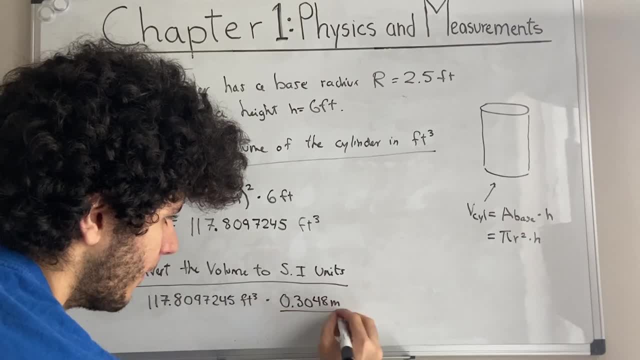 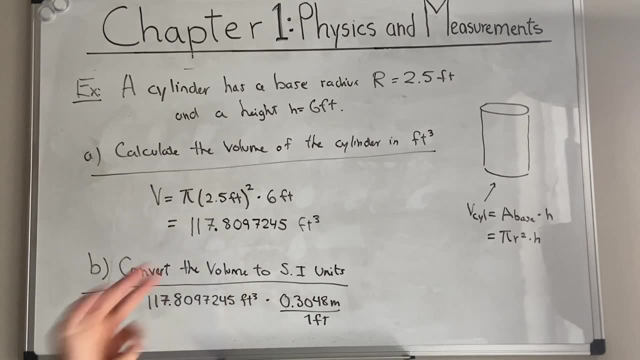 and we're going to be of 0.3048 meters per foot. and you might ask yourself: wait, Noah, we, this is feet cubed, and here we only have feet. so if we multiply these two fractions, considering that there's a one underneath here at the denominator, if we 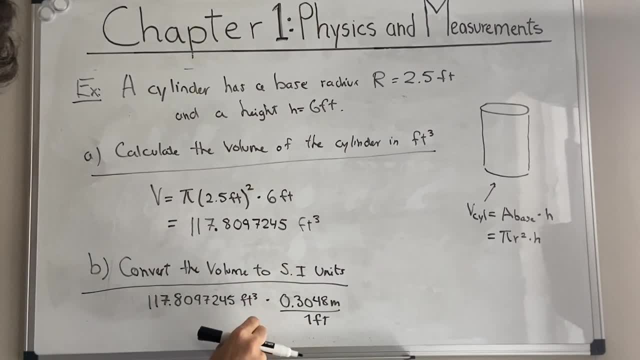 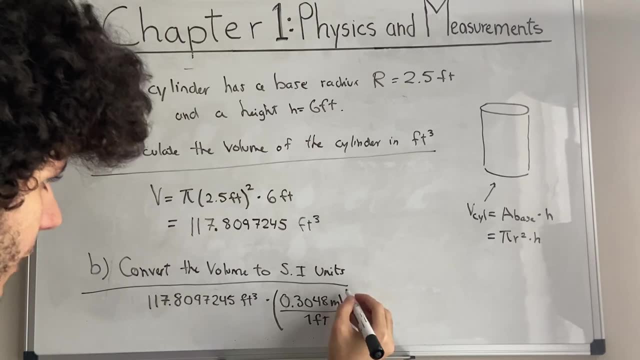 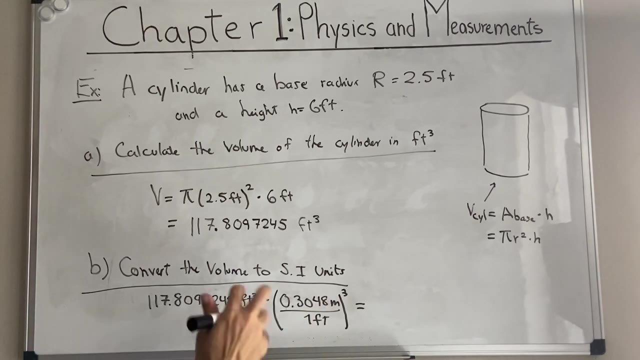 multiply, we're only gonna. we're going to have feet squared times meters, which is not what we want. so what we need to do is actually cube this fraction, this conversion ratio, in that that way, we'll have feet cubed and meters cubed. these will cross out and we'll have meters cubed as a result. so when we do that, we 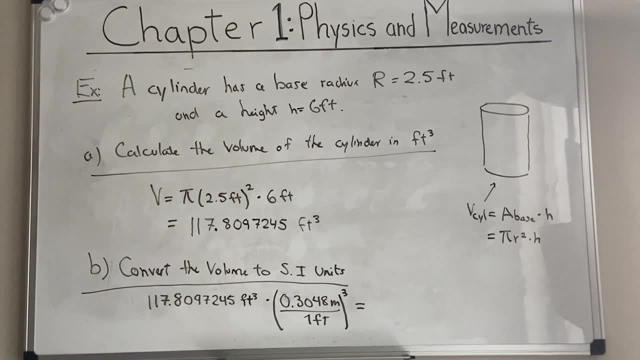 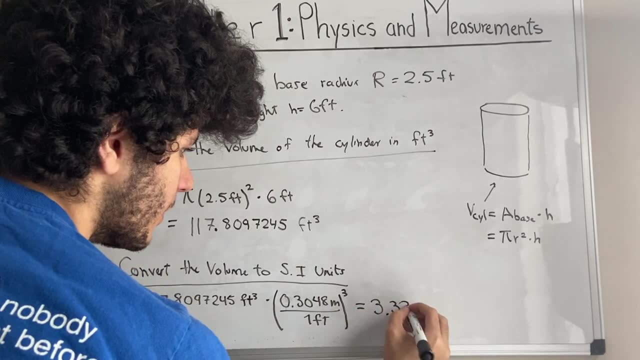 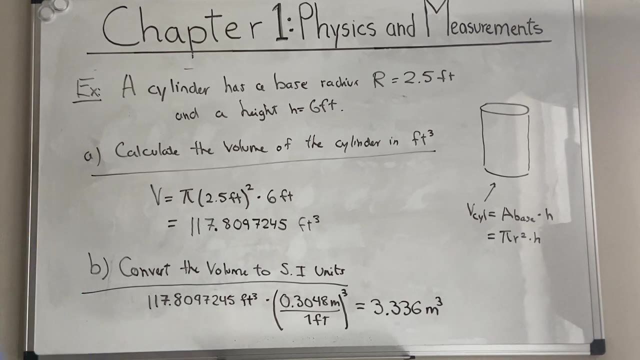 end up with three point three, three, six meters cubed, of course, because we're dealing with a volume okay. well, fantastic, we have our result and that's an example, a very brief example, of conversion ratios. you're gonna deal with these a good bit in physics. well, usually we want to. usually the problem will: 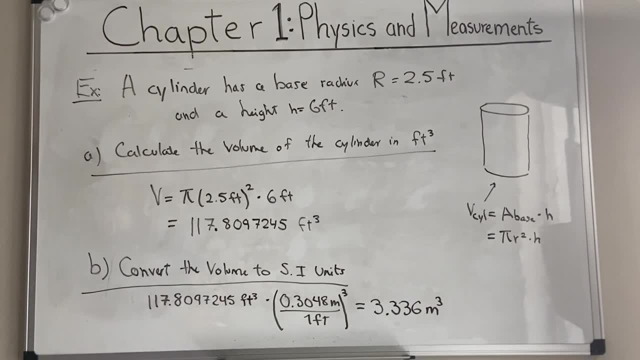 already give you the SI units, because the emphasis is more on the how rather than these little meticulous changes of units. it's that's not what we're trying to do. that's all, professor. they're trying to test you with, they're trying to find out if you actually know how to apply formulas, not change units something. 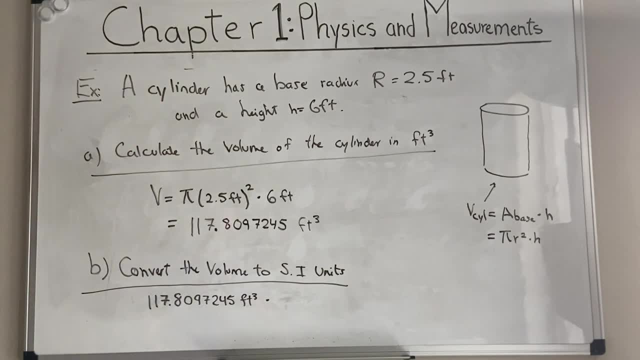 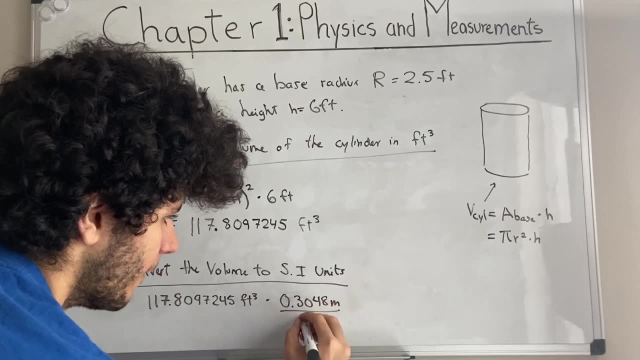 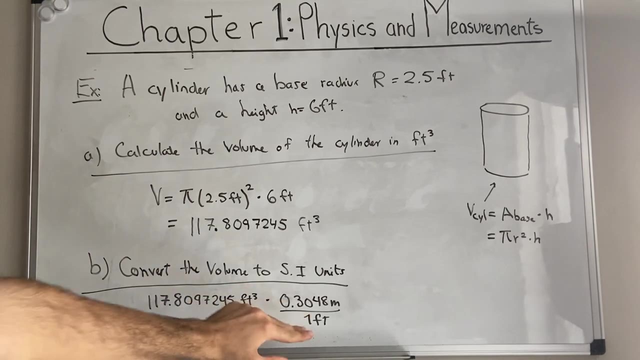 write that and then we put it on top. Yeah, So it was just double-checking: 3048 meters per foot. And you might ask yourself: wait, Noah, this is feet cubed and here we only have feet. So if we 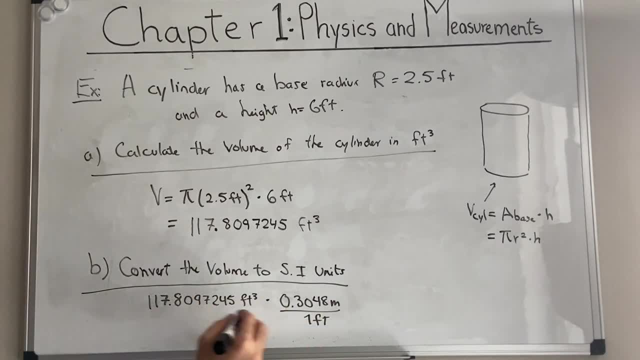 multiply these two fractions, considering that there's a one underneath here as the denominator. if we multiply we're going to have feet squared times meters of height. So 1.255 feet cubed, So we're going to have feet squared times meters. So if we multiply, we're only going to. 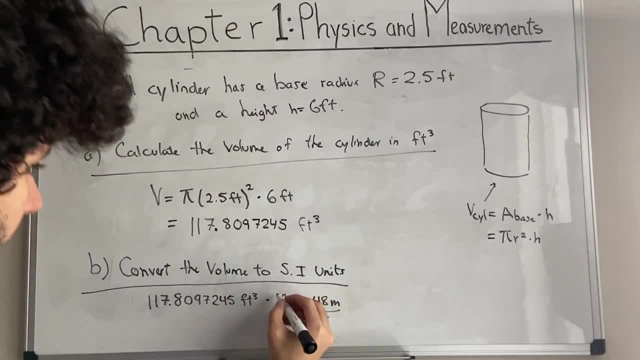 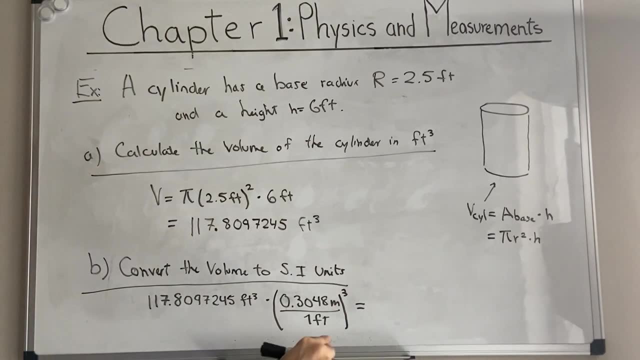 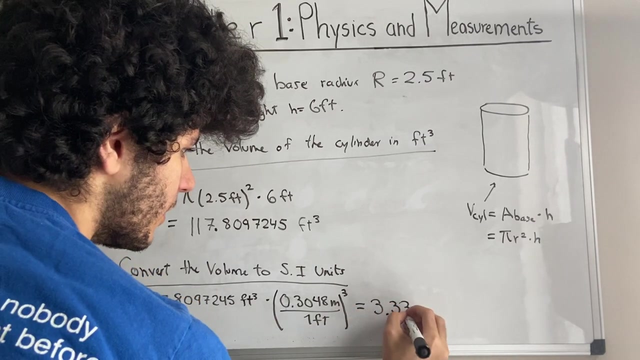 meters, which is not what we want. so what we need to do is actually cube this fraction, this conversion ratio, in that that way, we'll have feet cubed and meters cubed. these will cross out and we'll have meters cubed as a result. so when we do that, we end up with three point three, three, six meters cubed of. 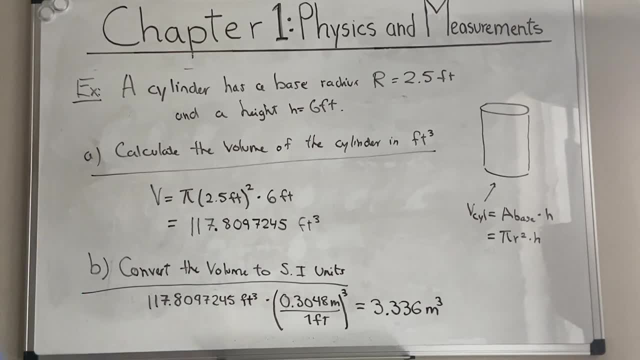 course, because we're dealing with a volume, so it's three dimension, okay, well, fantastic, we have our result and that's an example, a very brief example, of conversion ratios. you're gonna deal with the a good bit in physics. well, usually we want to, usually the problem will already. 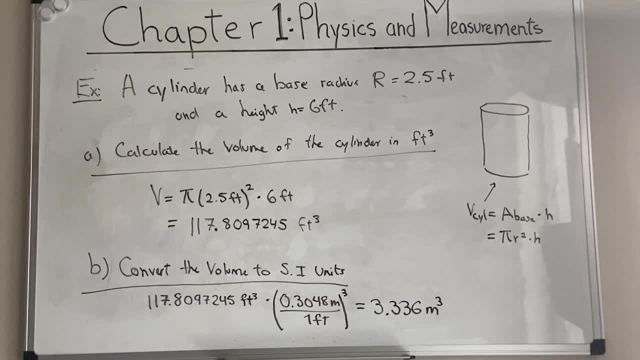 give you the SI units, because the emphasis is more on the how rather than these little meticulous changes of units. it's that's not what we're trying to. that's all professors are trying to test you with. they're trying to find out if you actually know how to apply formulas, not change units. something that's a. 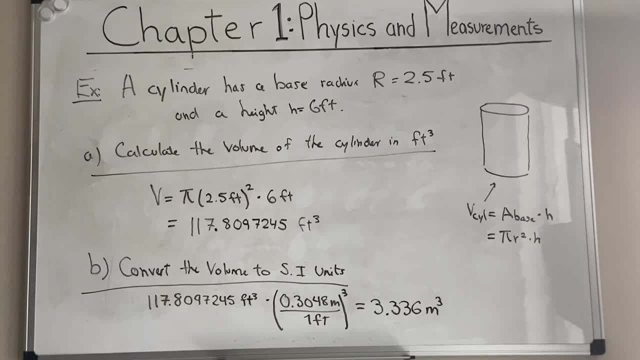 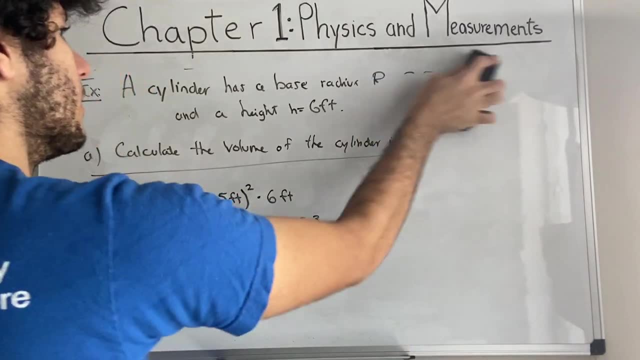 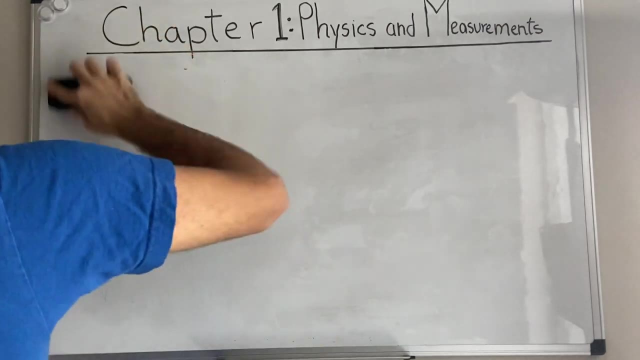 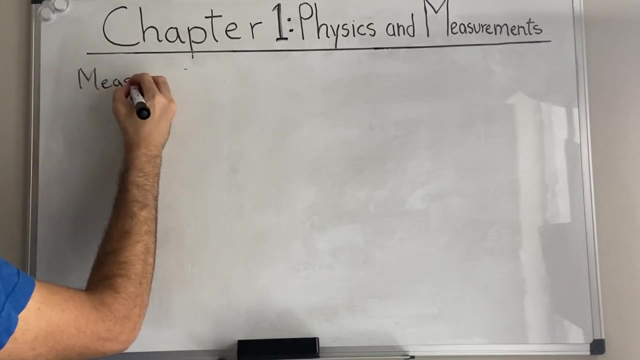 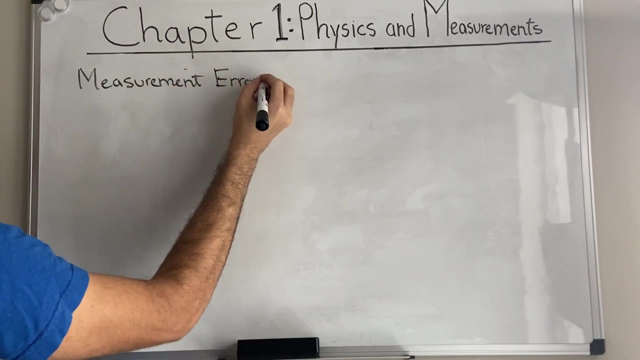 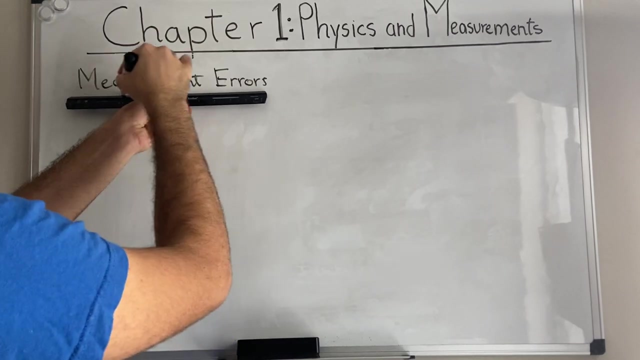 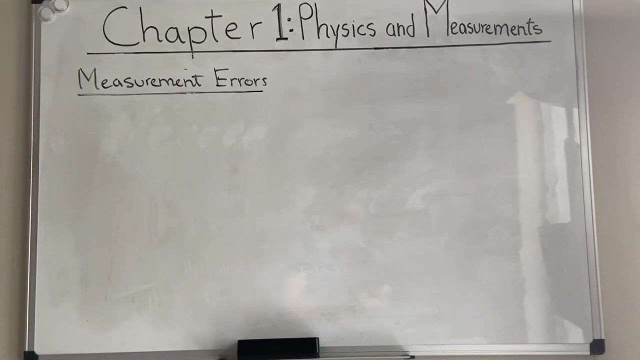 that's a little less, a little more casual. okay, we will now move on to our next section, chapter one, which is measurement errors. measurement errors: I can only find by my loom. okay, here we go. all right, so measurement errors. One very, very important idea to consider in physics and in any science is that 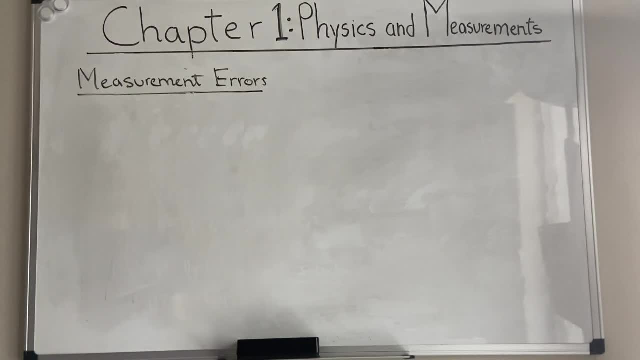 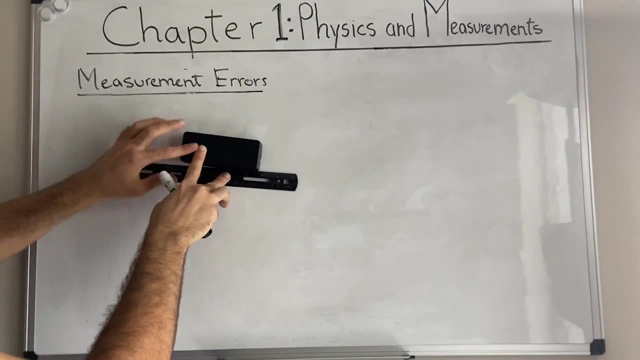 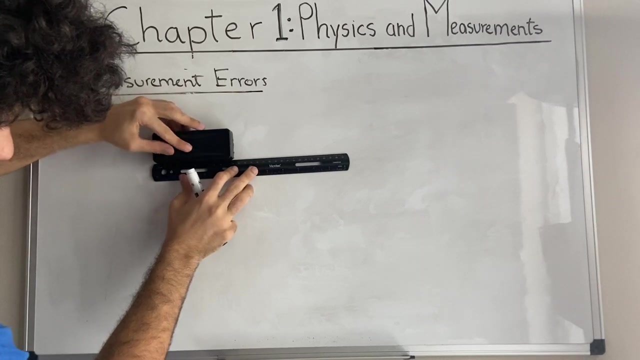 all measurements are subject to error. If I'm going to try to measure how long this this eraser is, I will put my ruler up to it say that this will be 0.0. So we put 0 centimeters along with it, and then we can see how long it is. 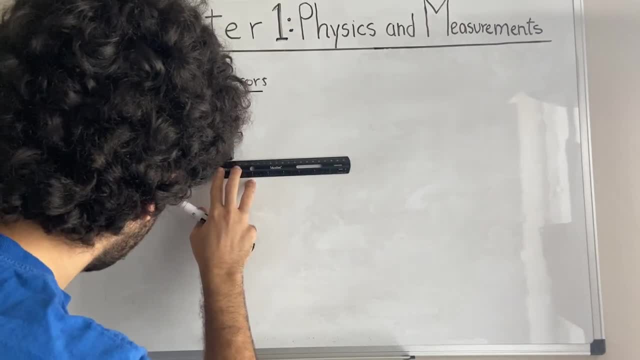 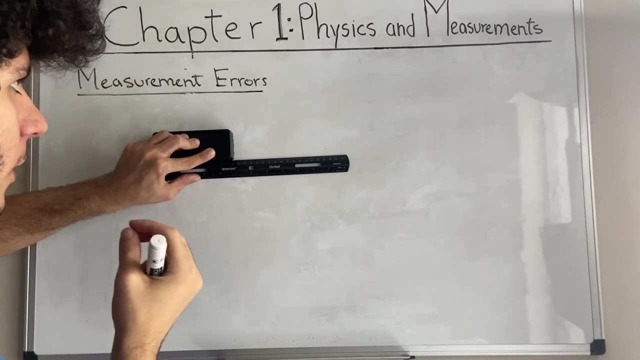 right. So we'll end up with about 12, a bit more than 12 centimeters, but the thing is that we don't know how we can never be sure about our amount of measurement, like exactly down to the very decimal. Sure, we know that it's. 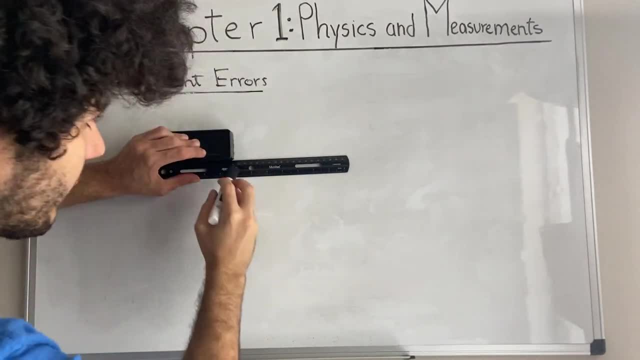 above 12, it's very clearly above 12 for me, Look, it's a little bit difficult to see, But we don't know which is more difficult. So this one: it's symbolized above the first digit of the matrix, so we filled in the 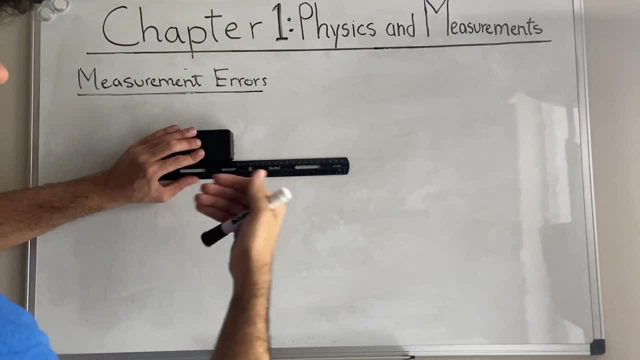 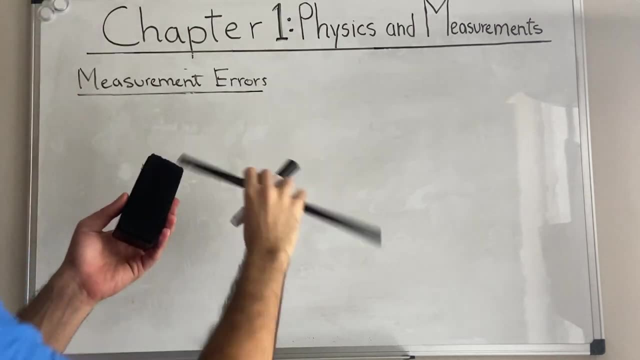 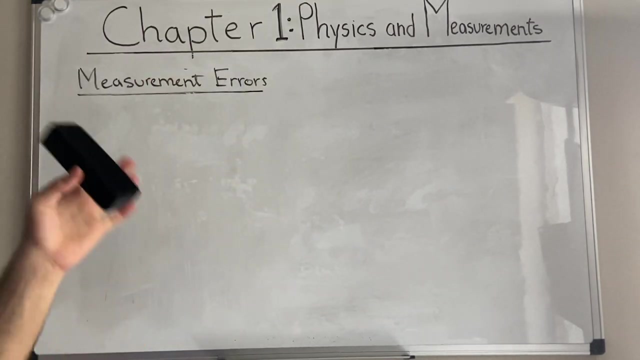 know exactly what to like. to what decimal do we have to go to be sure that we have the exact measurement? we'll never be able to perfectly measure anything, except for whole entities like this. this is one eraser. if i had another, there would be two erasers. those aren't things that. 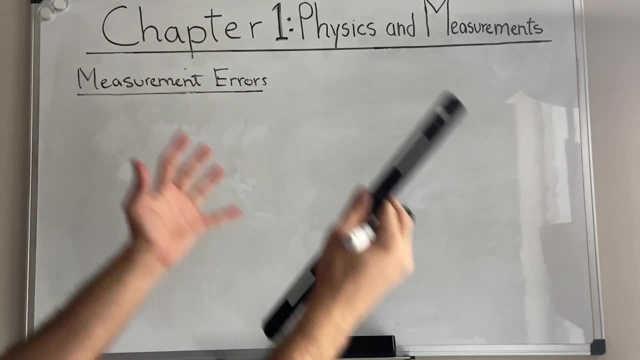 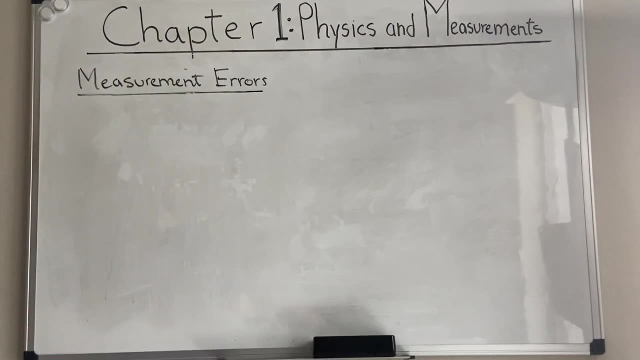 i don't measure those with tools. those are like they're very visible. maybe it's a little bit simple to see, but yeah, when you're measuring anything with a tool, or even with your eye, if you you're trying to guess how long this is- you'll never have a perfect measurement. thus, 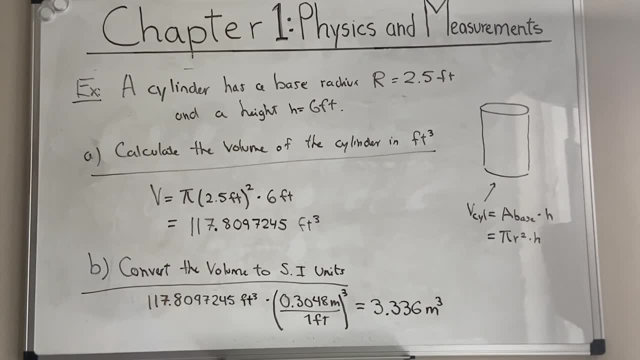 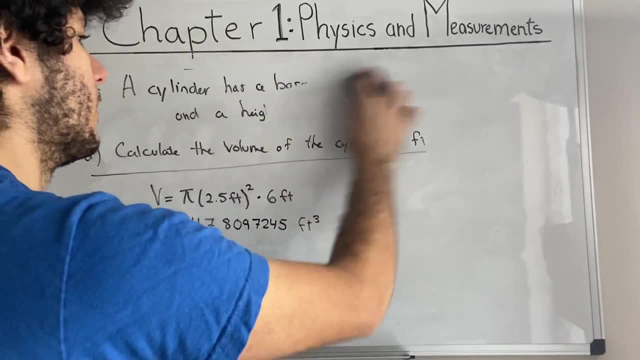 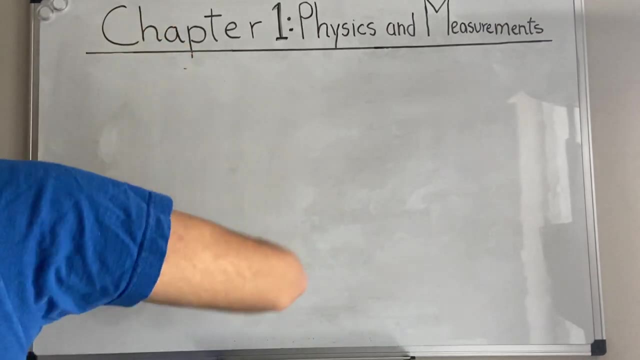 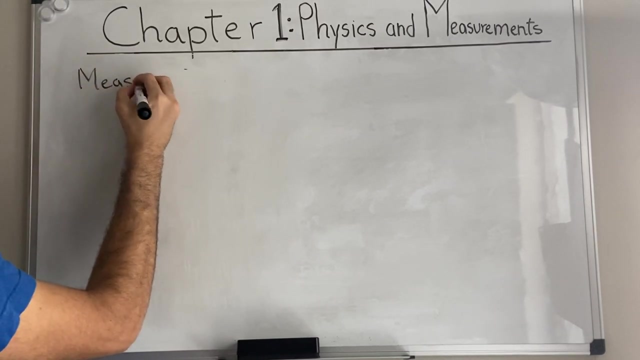 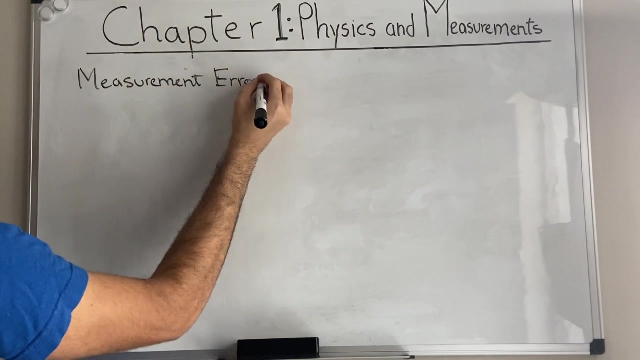 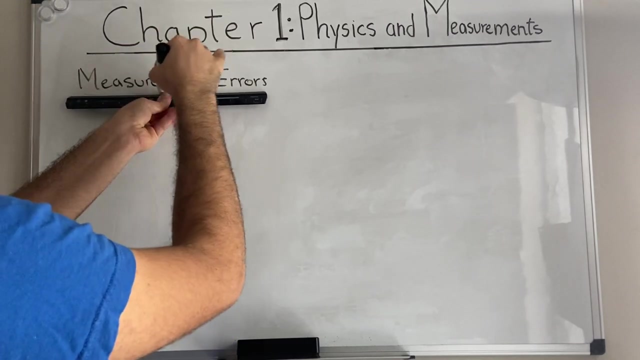 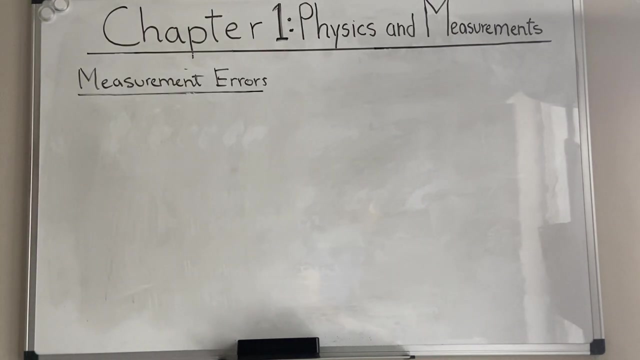 little less, a little more casual. okay, we will now move on to our next section, chapter one, which is measurement errors. measurement errors: I can only find my lower okay rooms. it's too bad. all right, so measurements: one very, very important idea to consider in physics and in any science is that all measurements are subject to error. if I'm 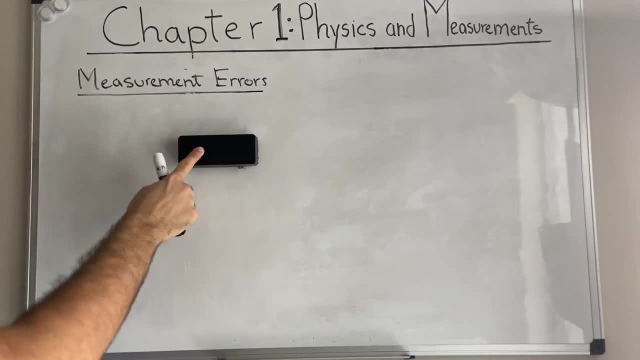 going to try to measure how many limits 100 schools an answer rule. I wouldn't try to measure how many limits one answer in this picture because it would solve it to see just how many time the least. so anybody want have to say: please stop how long this this eraser is. I will put my ruler up to it, say that this will be. 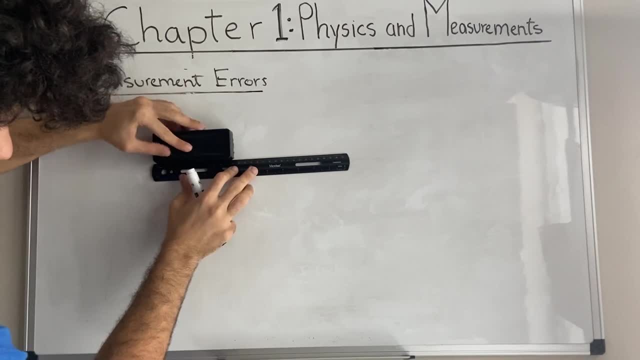 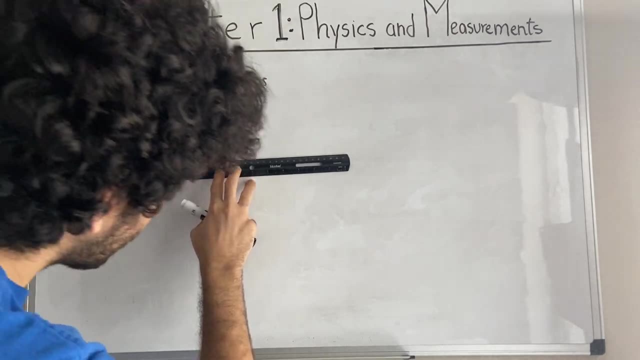 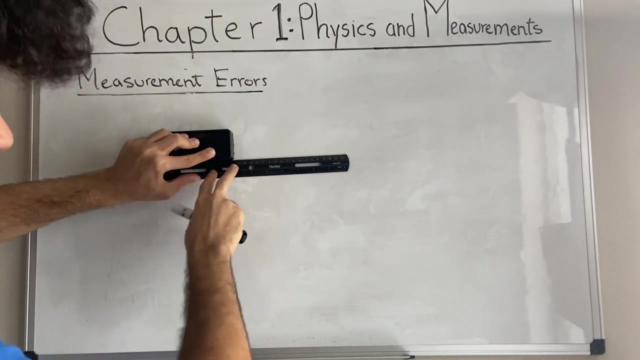 0.0 and we. so he puts 0 centimeters along with it, and then we can see how long it is right. so we're. we end up with about 12, a bit more than 12 centimeters, but the thing is that we don't know how. we can never be sure about our. 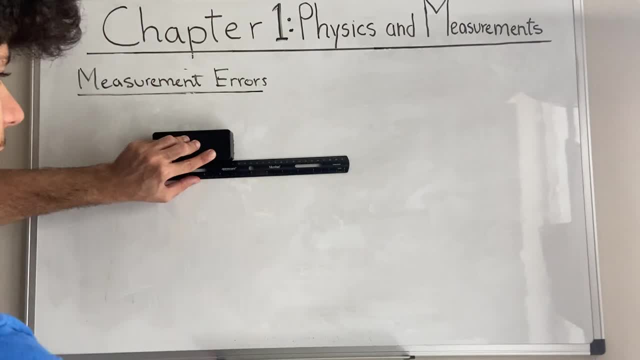 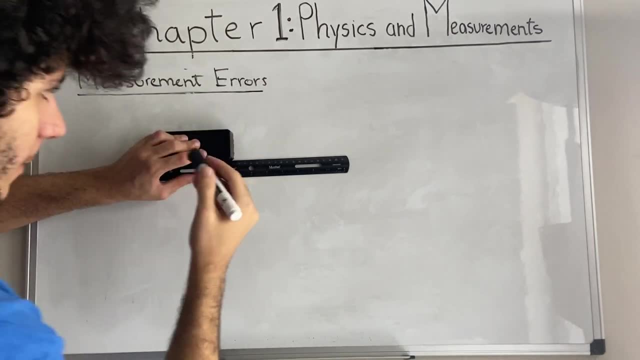 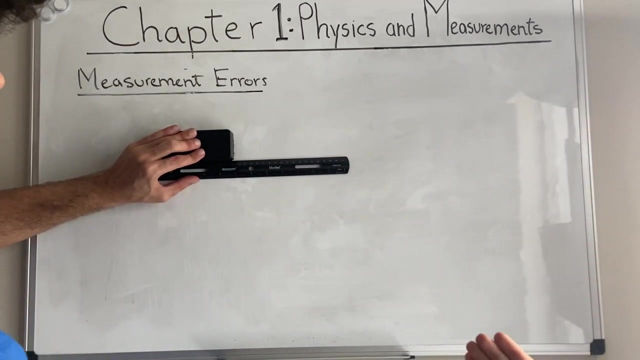 measurement like exactly down to the very decimal. sure, we know that it's above 12. it's very clearly above 12. for me, maybe it's a little bit difficult to see, but we don't know exactly what to like. to what decimal do we have to go to? 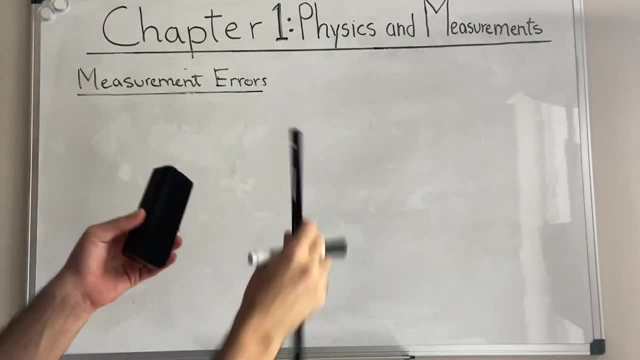 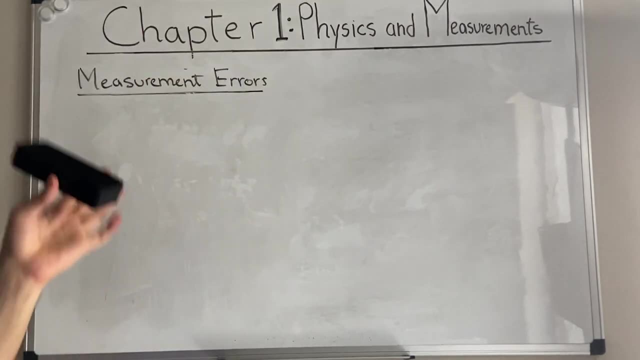 be sure that we have the exact measurement. we'll never be able to perfectly measure anything, except for whole entities like this. this is one eraser. if I had another, there would be two erasers, and then there would be three erasers, and then there would be two. 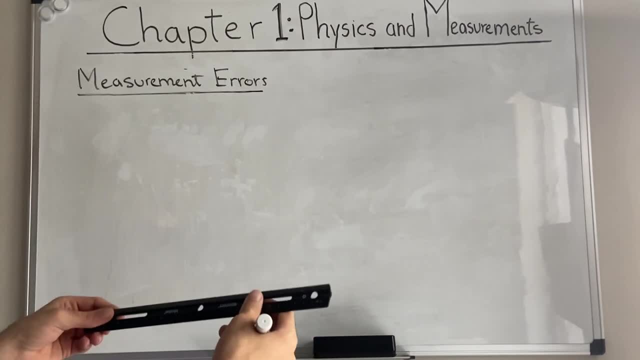 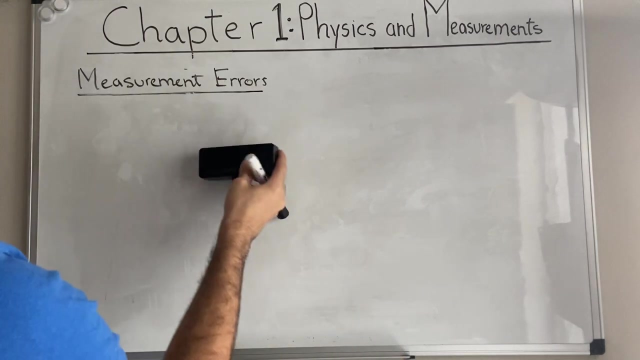 erasers. those aren't things that I don't measure those with tools. those are like they're very visible. maybe it's a little bit simple to see, but yeah, when you're measuring anything with a tool, or even with your eye, if you you're trying to guess how long this is, you'll never have a perfect measurement. thus, 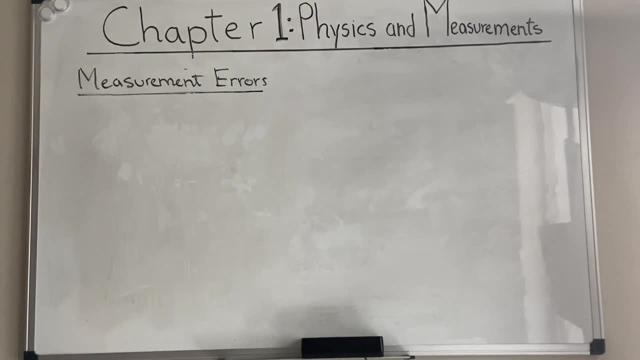 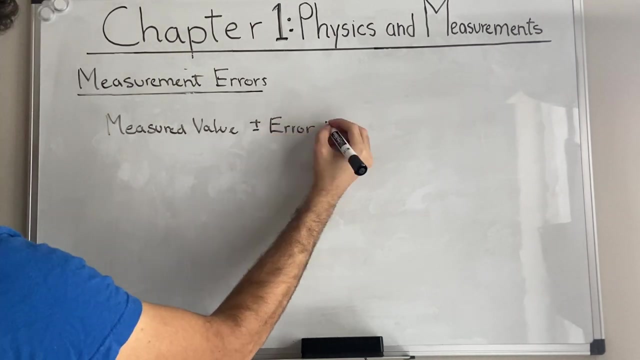 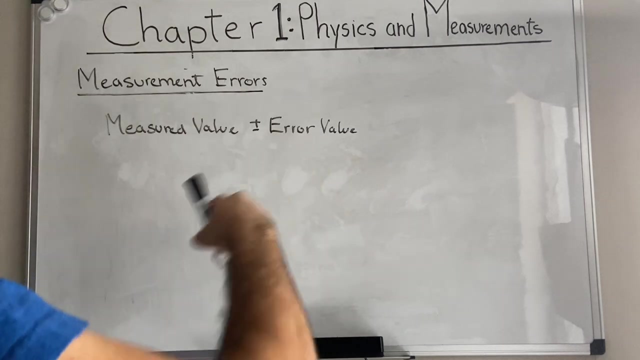 all measurements are subject to error, and so, ideally, every measurement should be reported as a measured measured value. we're really running out of ink plus or minus an error value. by adding this, we're basically considering or accepting the fact that our measurement will not necessarily be perfect. 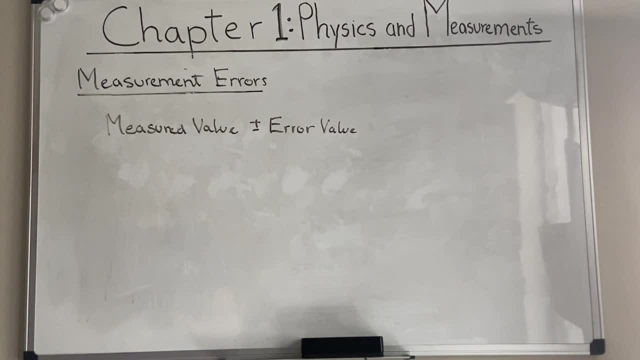 and that there will. actually, it will never be perfect. there's always going to be a certain amount of error and certainty in our measurement. so an example: say we have a block of something that we're trying to measure and we have a ruler. you, I'm going to measure it with a ruler and I'm going to measure it with a ruler. 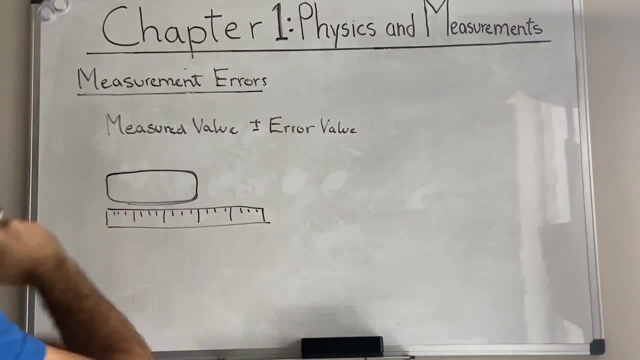 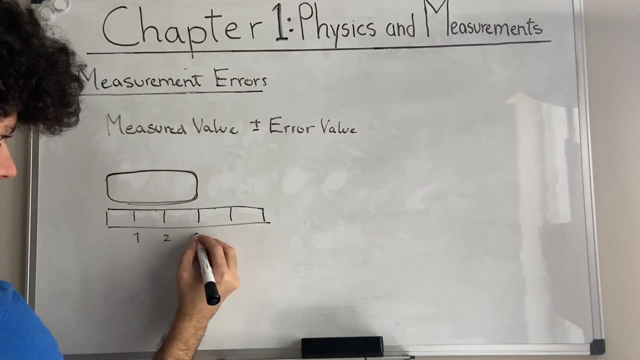 okay, three. okay, now forget about these measurements. it just considers to be a ruler and let's say, actually let's consider the measurements, little measurements, the increments. let's say that this is one inch, two inch, three inches, four inches, five inches. okay, so the length of the ruler is the length of the ruler. 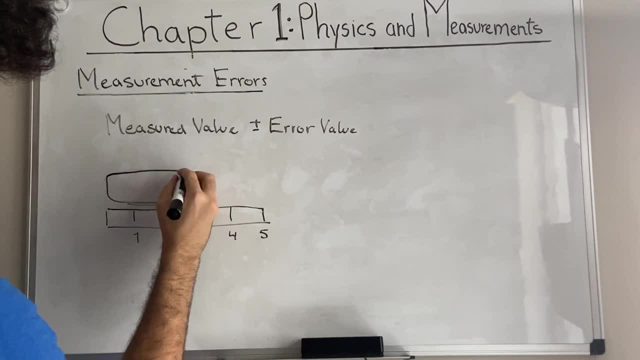 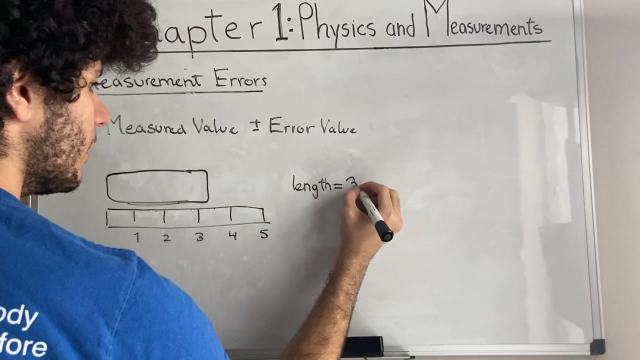 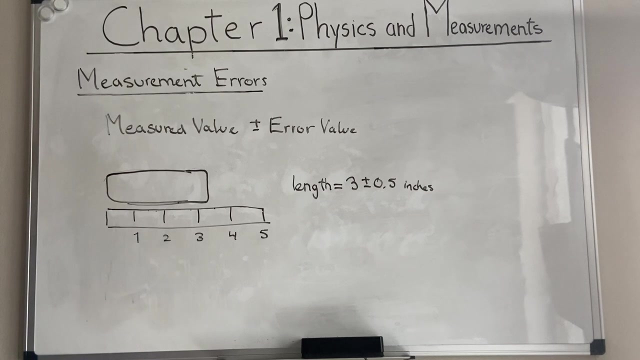 of this box we. a proper way to report this value would be as such, the length is equal to 3 plus or minus 0.5 inches. so basically, we're finding the smallest, the smallest increment, which is one inch. we divide that by two, and thus we find our error value. otherwise, the only measurement that we can 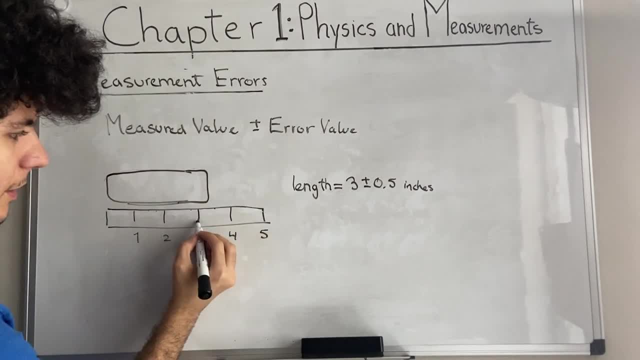 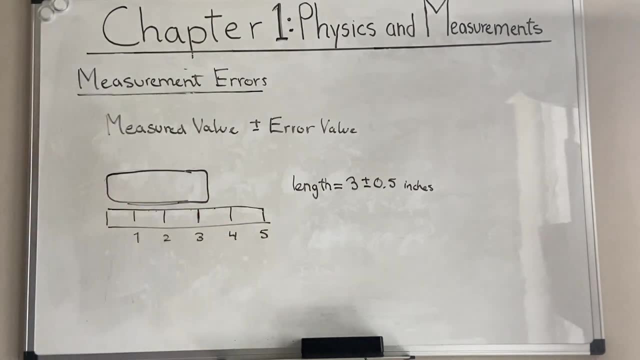 be certain of the measured value. is three right? because there's no, there aren't any measurements in between three and four, so we can't be sure of such a measurement. and with this way of noting measurements we basically are considering how many significant figures we want to add to the 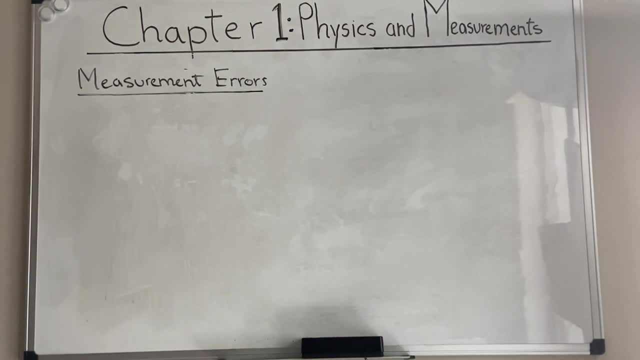 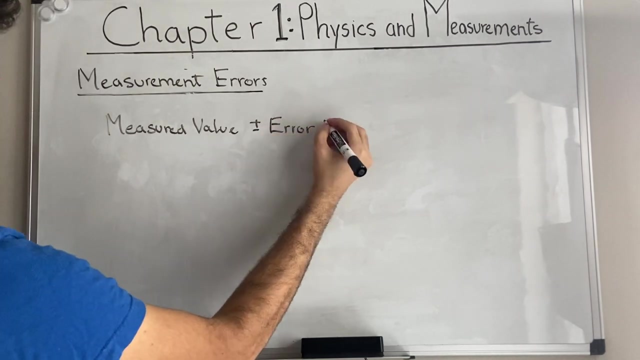 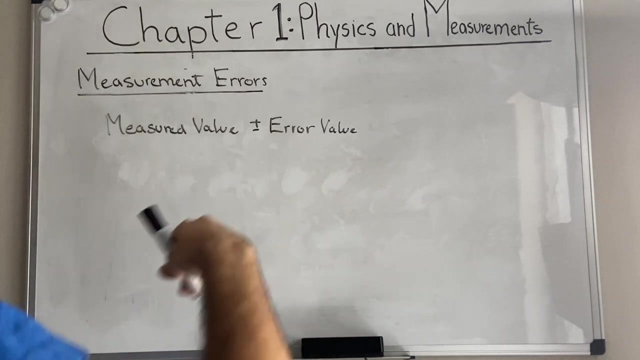 all measurements are subject to error, and so, ideally, every measurement should be reported as a measured, measured value- um, um, really running out of ink- plus or minus an error value. by adding this, we're basically considering, we're accepting the fact that our measurement will not necessarily be perfect and that there will actually will never be perfect. 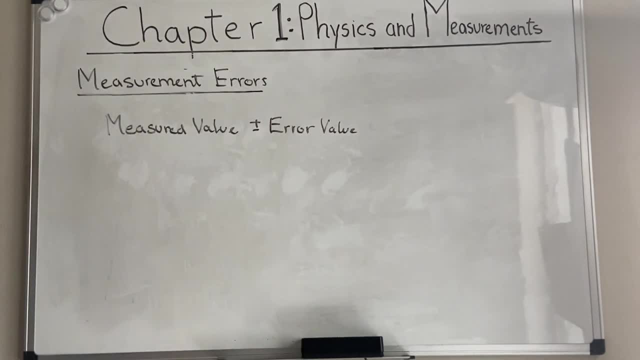 there's always going to be a certain amount of error and certainty in our measurement. so an example: say, we have a block of something that we're trying to measure and we have a ruler. three bang, okay, three, oh Okay. now forget about these measurements. just consider this to be a ruler and let's 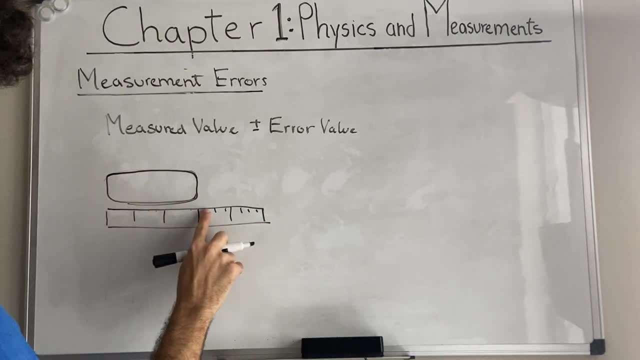 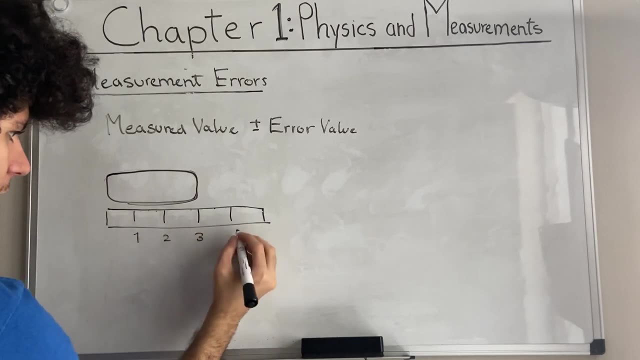 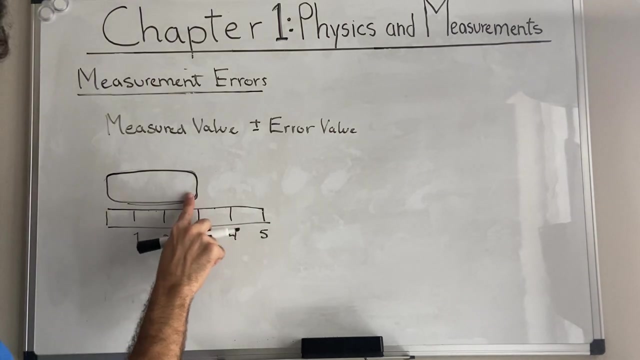 say, actually, let's consider the measurements, the little measurements, the increments. Let's say that this is 1 inch, 2 inch, 3 inches, 4 inches, 5 inches. okay, So the length of this box. a proper way to report this value would be, as such, the length. 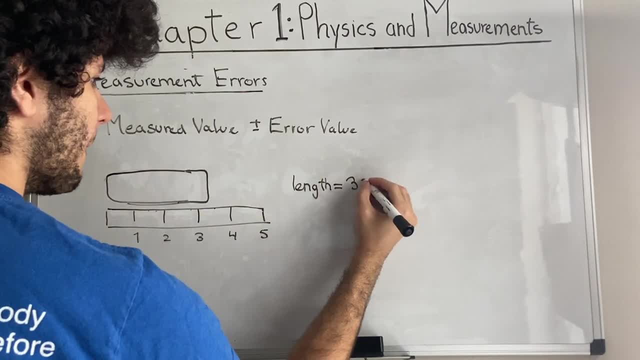 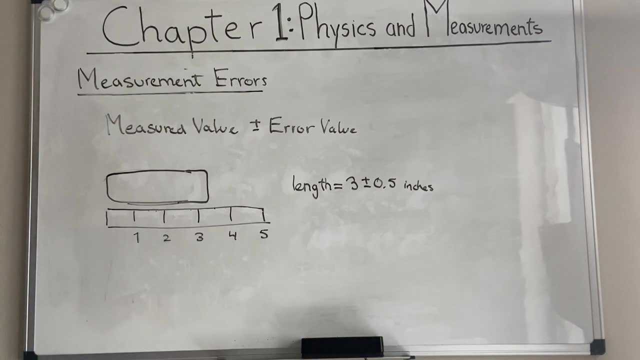 is equal to 3 plus or minus 0.5 inches. So basically, we're finding the smallest, the smallest increment, Which is 1 inch. we divide that by 2, and thus we find our error value. Otherwise, the only measurement that we can be certain of the measured value is 3, right. 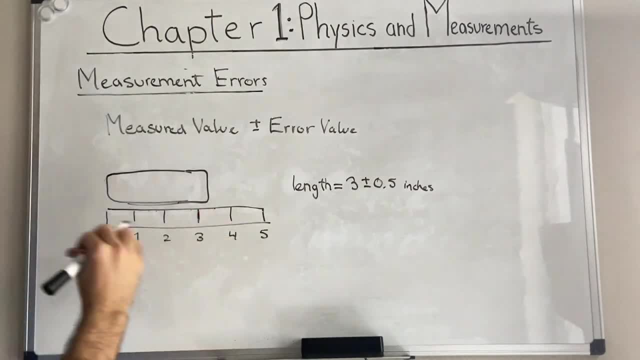 Because there's- no, there aren't any measurements in between 3 and 4, so we can't be sure of such a measurement. And with this way of noting measurements, we basically are considering how many significant figures we want to add to the number right. 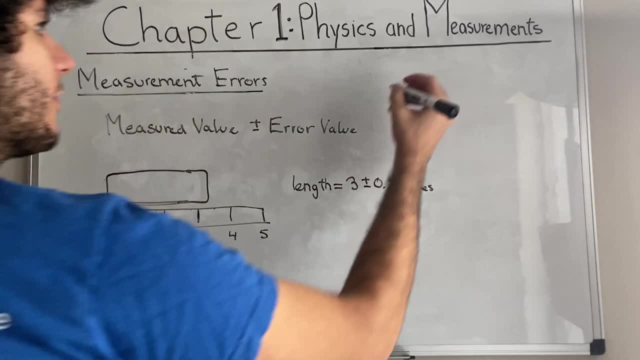 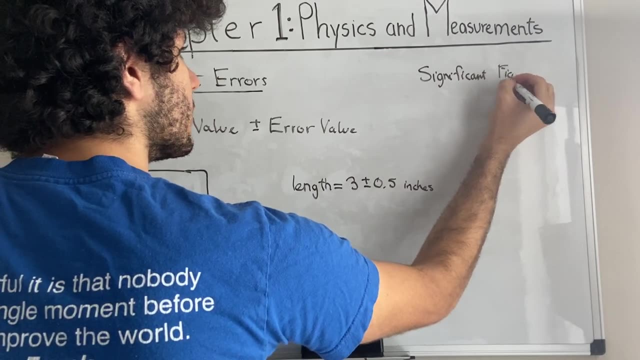 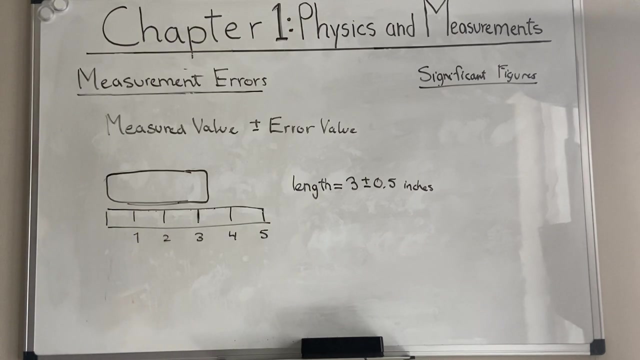 So, and I'm going to explain that right now- So significant figures, significant figures, these are basically the digits that carry meaningful contributions to the measurement's resolution, And that might sound a little bit daunting. you might be asking, like: what does that mean? 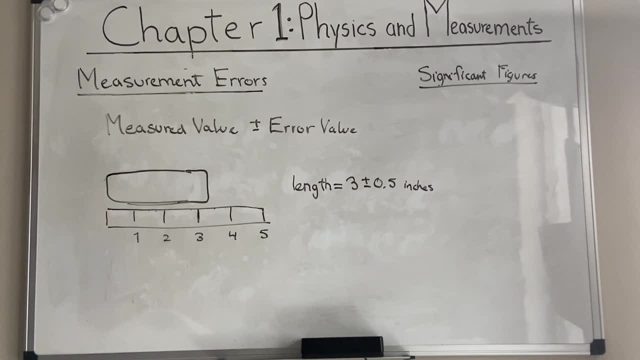 Well, the number of significant figures indicates the accuracy of a measurement, So it basically helps us determine how accurate a scientist was while he was measuring something, depending on if he was using a very good tool or if he was using his eye to determine the. 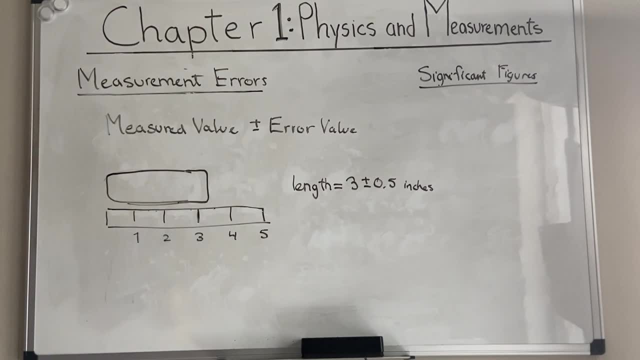 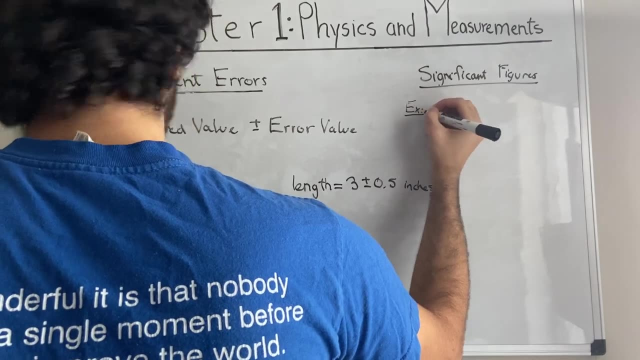 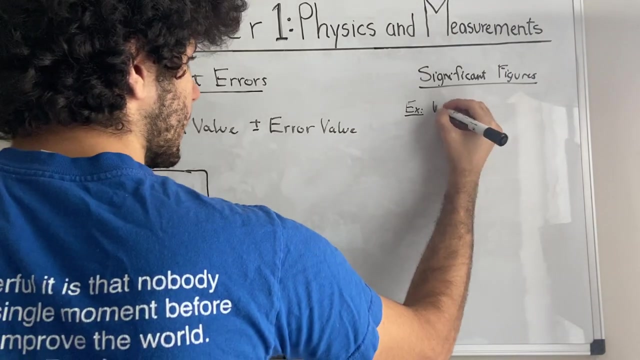 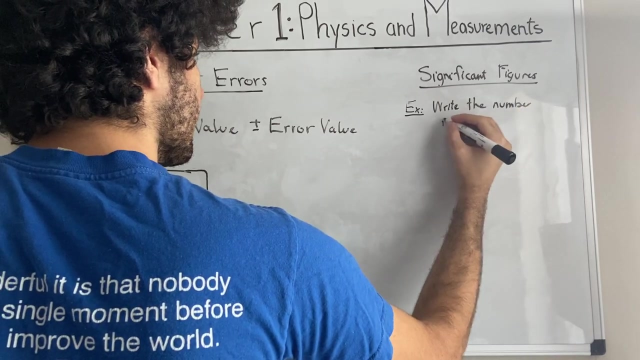 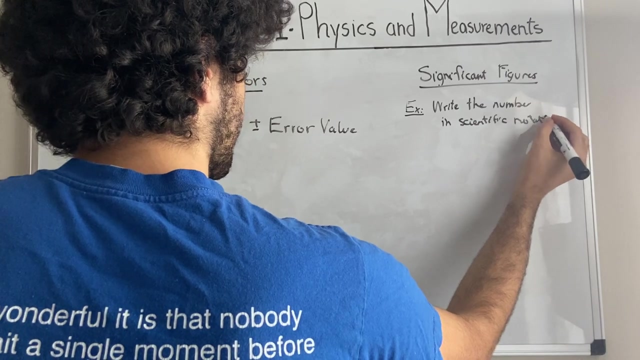 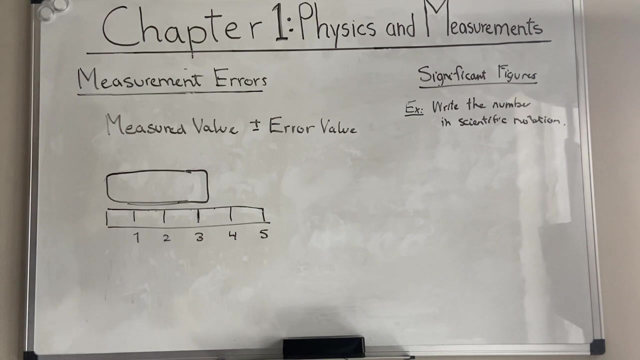 length of an object, which is very imprecise, Inaccurate I mean. So an example for significant figures would be the following: To write, to write the number in scientific notation, something that we're going to use quite a bit, especially in labs, not as much in actual theory, right? 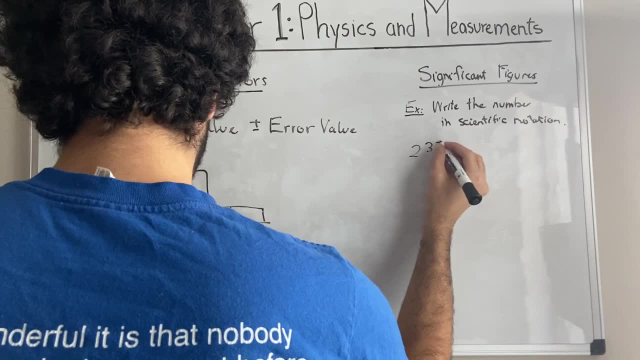 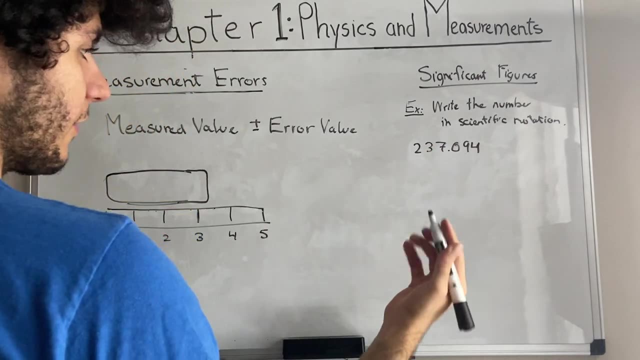 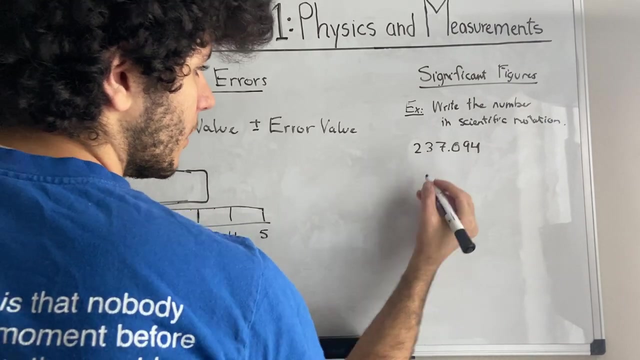 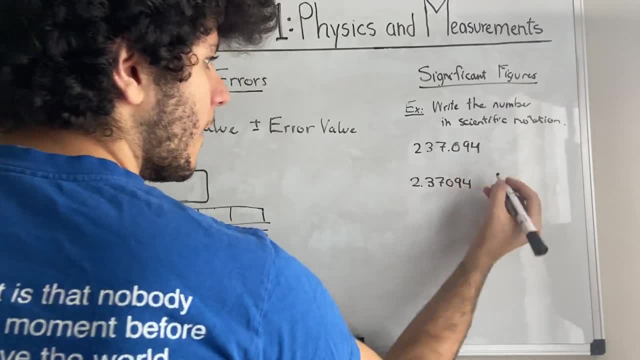 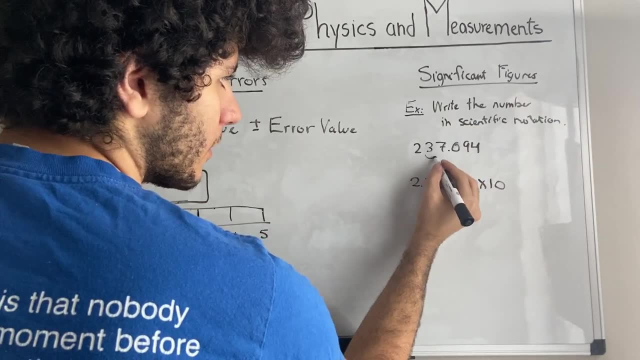 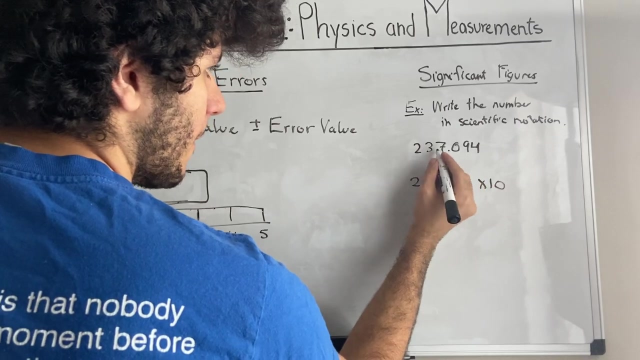 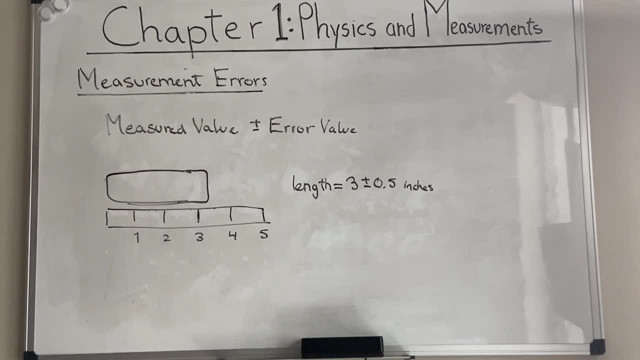 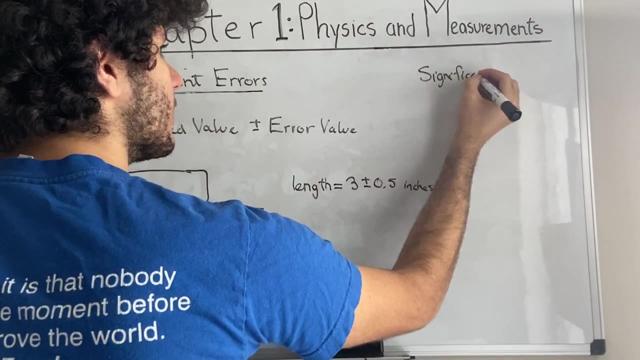 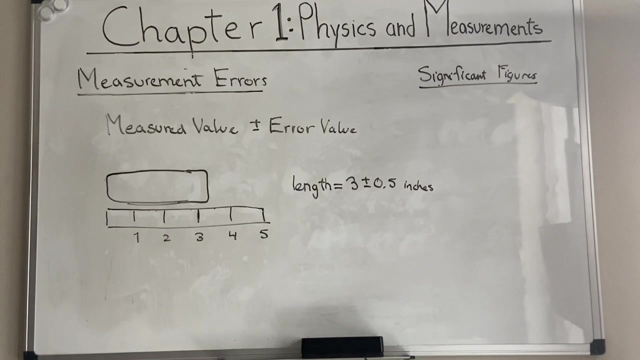 number right, so I'm gonna explain that right now. so, significant figures, figures, these are basically the digits that carry meaningful contributions to the measure measurement's resolution, and that might sound a little bit daunting. you might be asking: like what? what does that mean? well, the number of significant figures indicates the accuracy of a measurement. 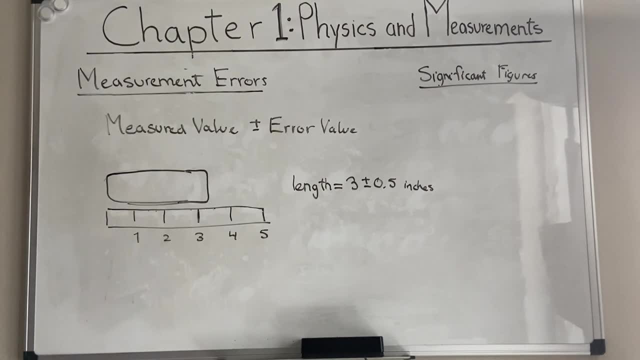 um, so it basically helps us determine how, how accurate a scientist was while he was measuring something, depending on if he was using a very good tool or if he was using his eye to determine the length of an object, which is very imprecise, inaccurate, I mean. so an example for significant 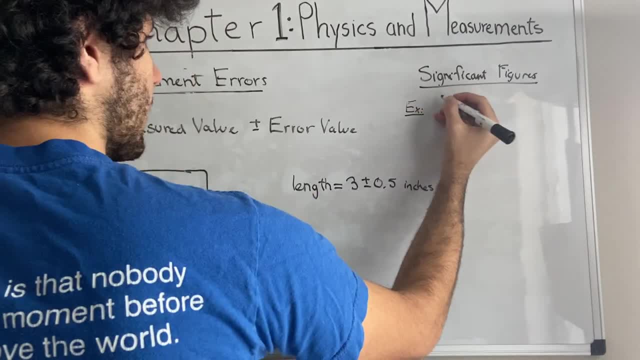 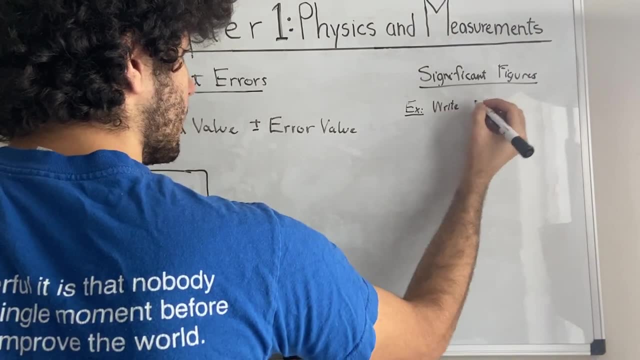 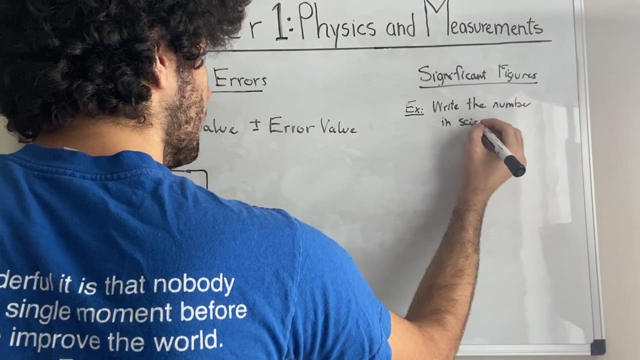 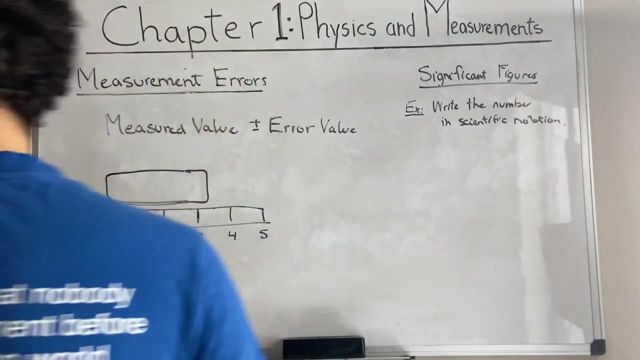 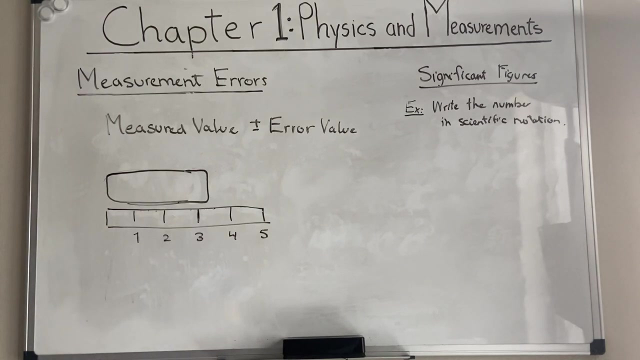 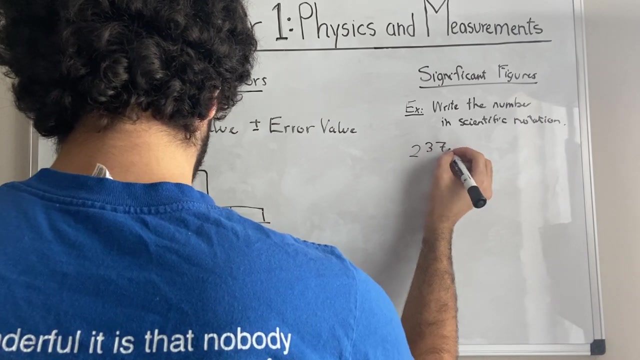 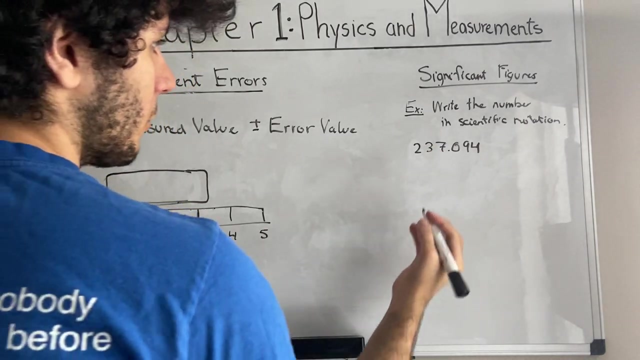 figures would be the volume to write right the number in scientific notes, something that we're gonna use quite a bit, especially in labs, not as much in actual theory, right? so we have 237.094. if we want to write this number in scientific notation, we're gonna want to. 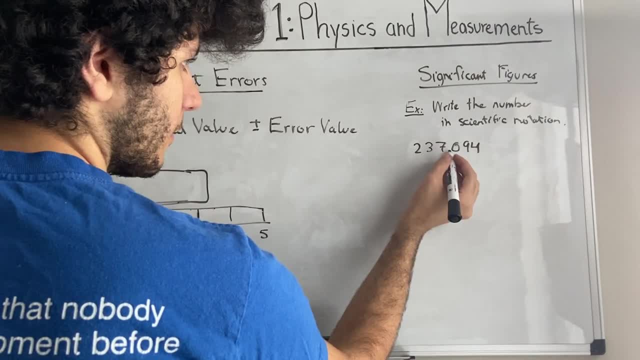 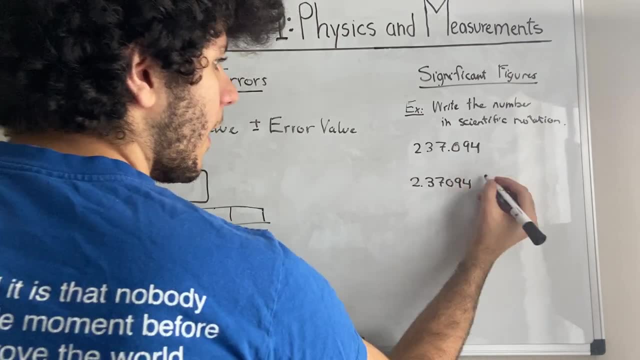 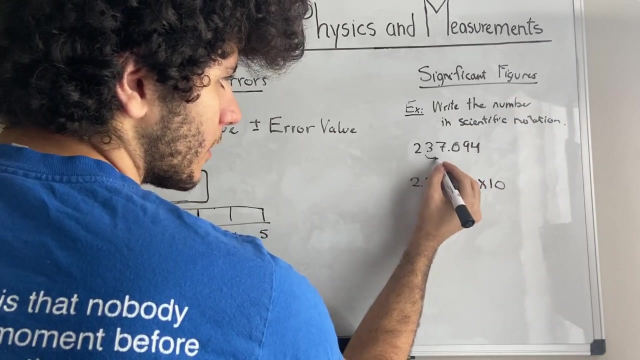 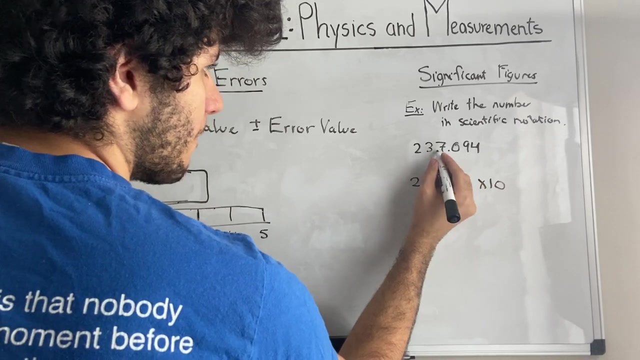 have um, the decimal point over here, so 2.37094, and then we're gonna multiply by 10 to the something to the x, and in this case it will be two, since we there's two, we moved the decimal point by two places to the left, meaning there's: 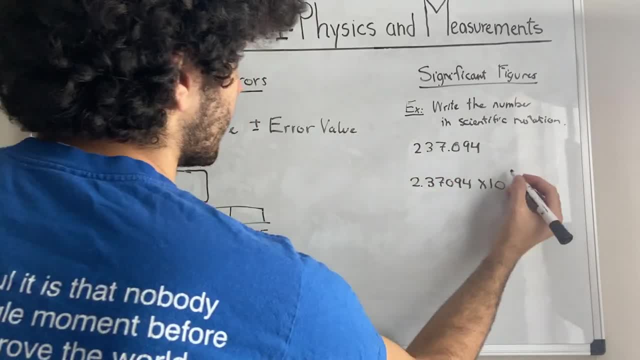 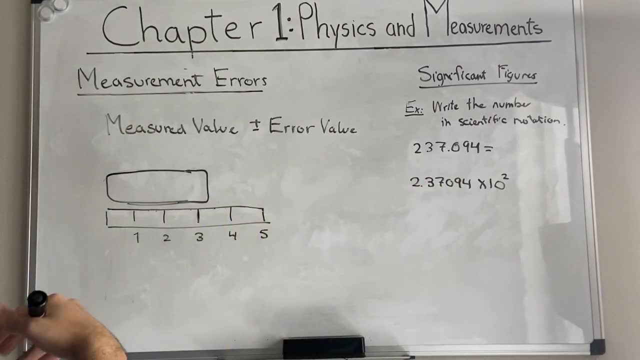 a hundred, that should be added to this number, or should that should be multiplied. so this is equal to four, and then we have back to zero, considering this is an editing real GDP on the decimal point. so divide by one and divide it. this to the sum of all the arguments that we actually have. 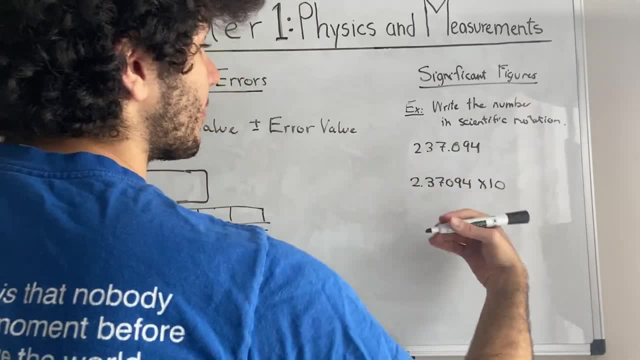 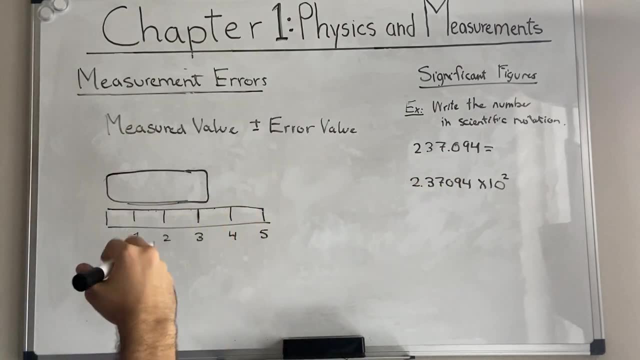 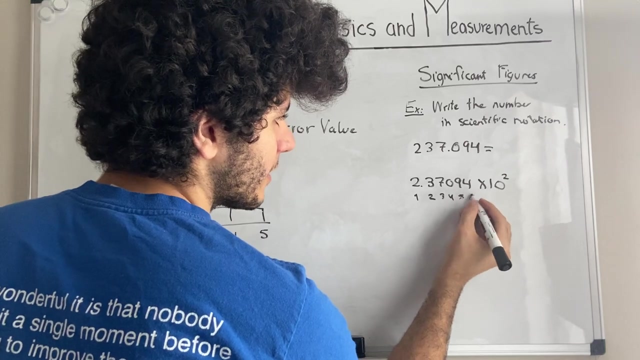 meaning there's a hundred that should be added to this number, that should be multiplied. So this is equal to that and that's scientific notation. And usually we use scientific notation to determine how many significant figures we have in a number. In this situation we have 1,, 2,, 3,, 4,, 5, 6 significant figures. 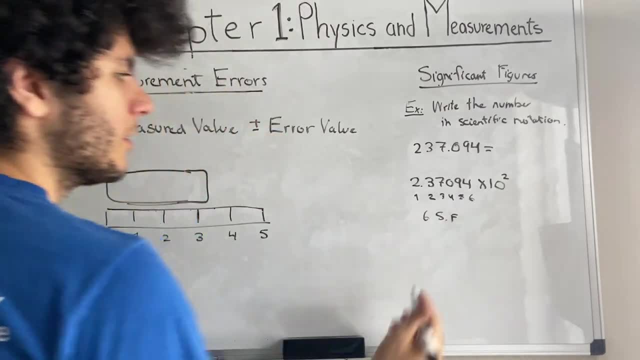 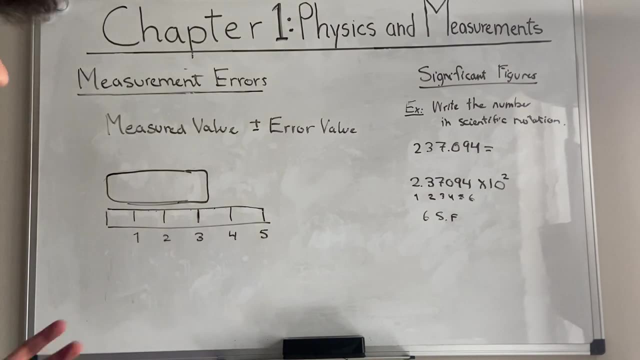 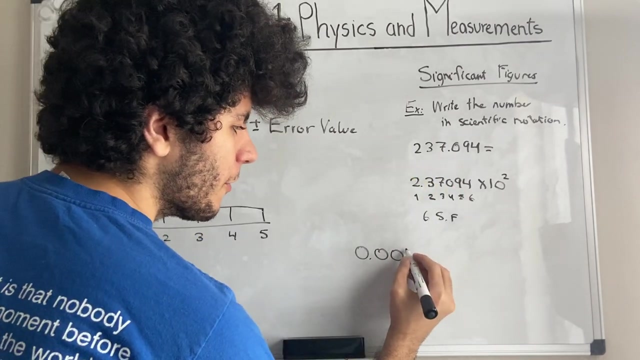 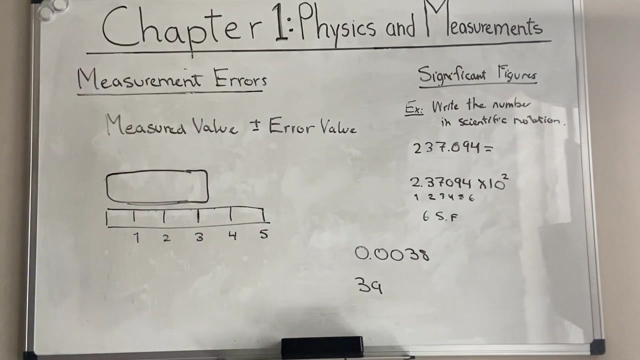 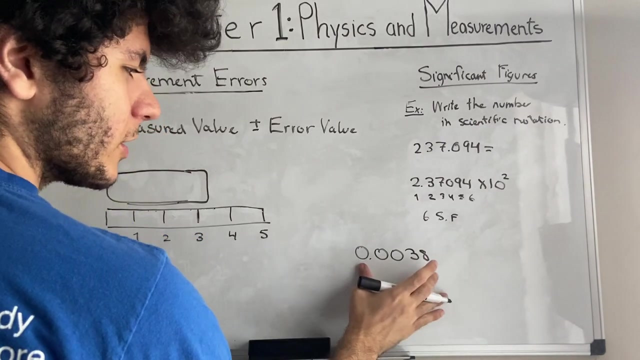 So 6SF Right. And in other situations where we have zeros such as this, Zeros not in the middle of the number, but rather before the number or after the number, Like this, Hold on. let me just deal with this first example. 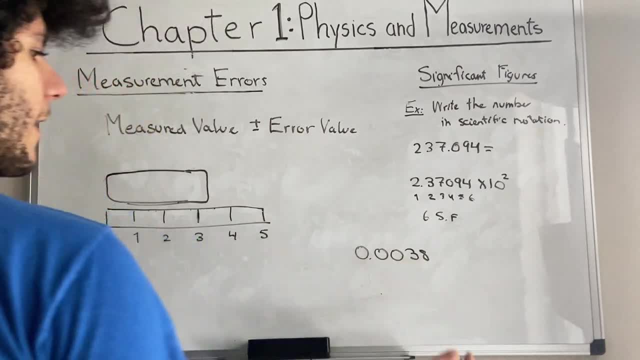 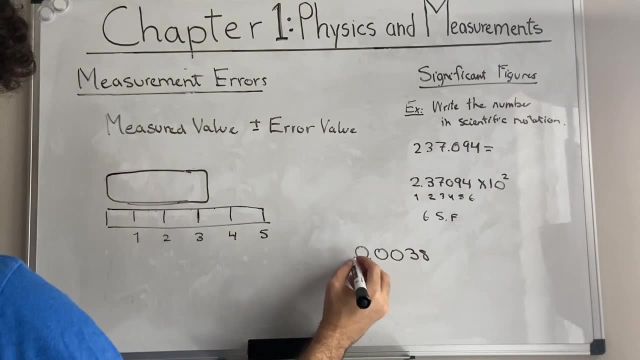 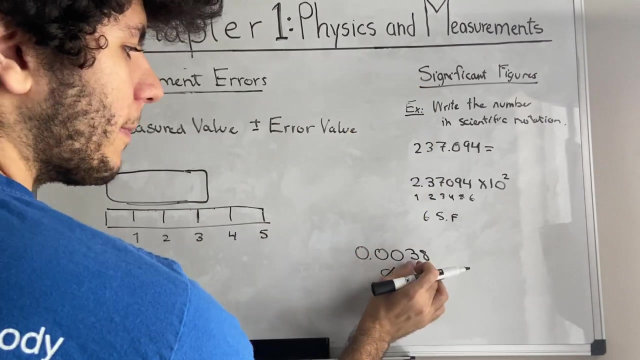 If we have, If we have zeros that precede the other numbers, then we actually do not consider these ones. These ones are not considered as significant figures, And the reason being is that these just determine how far away from Just like what position these numbers fall in. 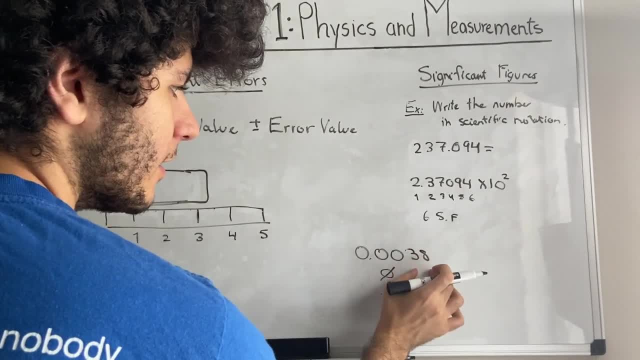 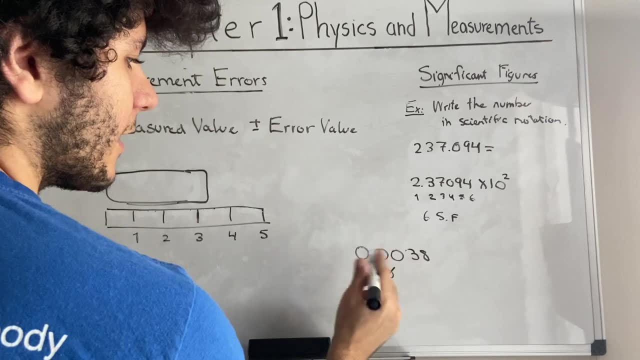 Basically saying that these 38. It's not just, It's not 38. This is: It's a very, very, very small number. Instead, like if it was, If we just wrote 38, that would be much larger than this. 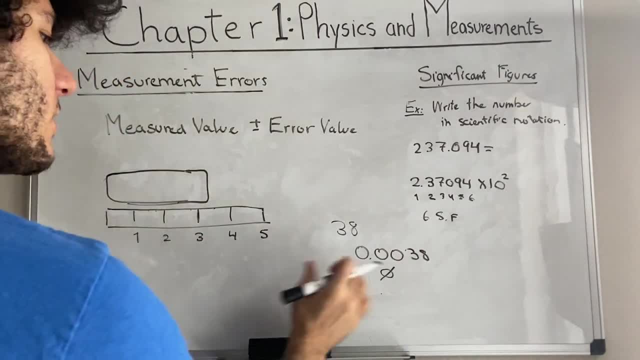 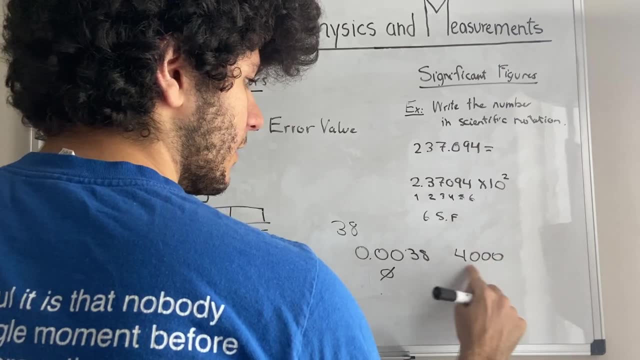 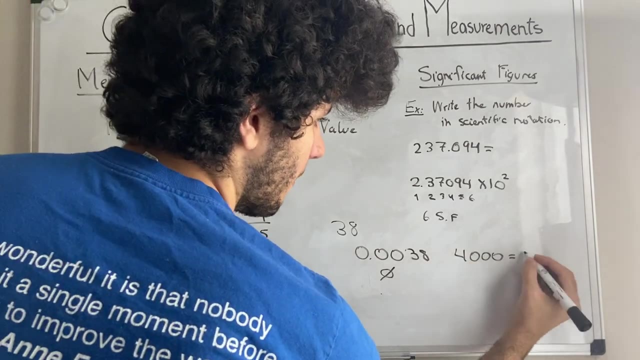 And the zeros just help us figure out how small this number is Right. On the other hand, if we had 4,000, these numbers are important Because if we put this into scientific notation, It would be written as 4,000 times 10, to the negative 3.. 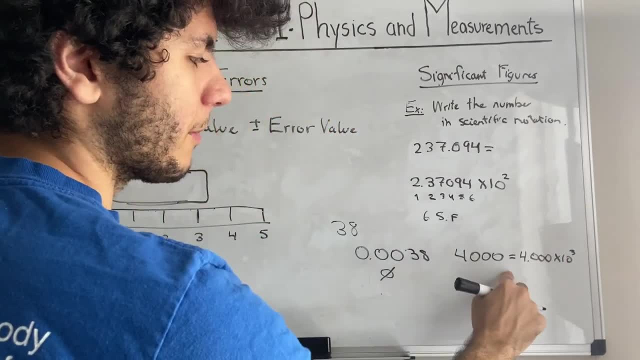 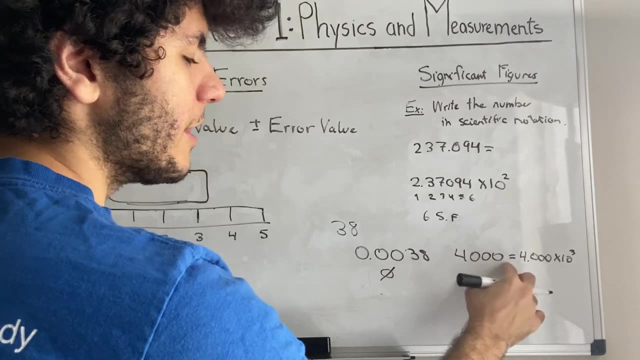 Times to the 3. Right. So you see, these numbers could have been other numbers if they were not significant, But they aren't. Or, and also, if these weren't significant numbers, then we wouldn't have written them here. 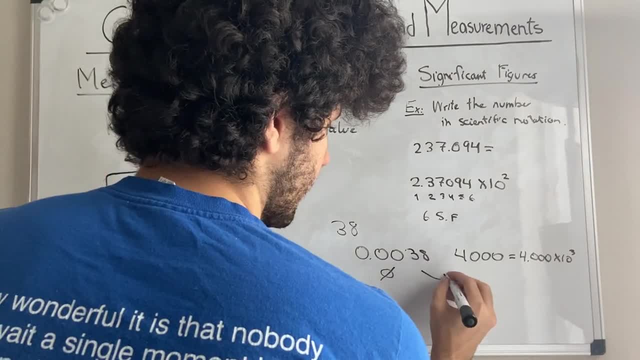 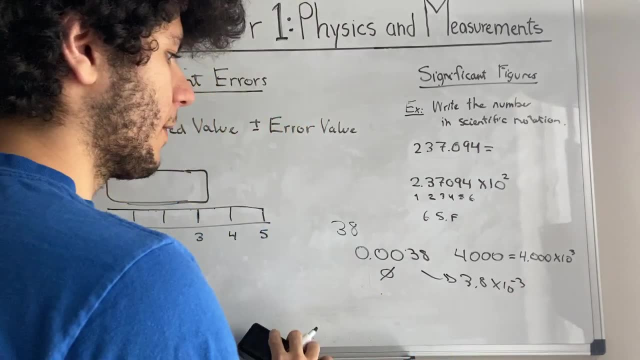 Yeah, Same thing goes for this. We can also write this as 3.8 times 10 to the 1,, 2,, 3. Negative, 3. Right, But we don't Well actually, Oh no. 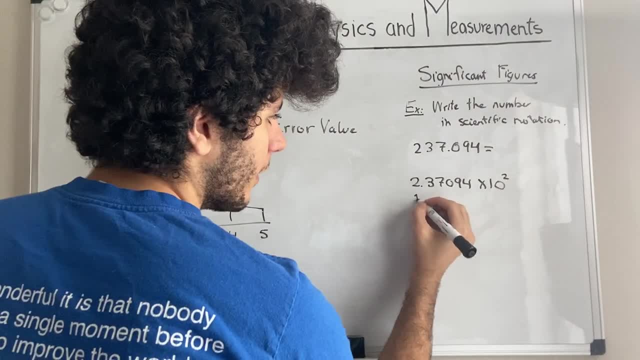 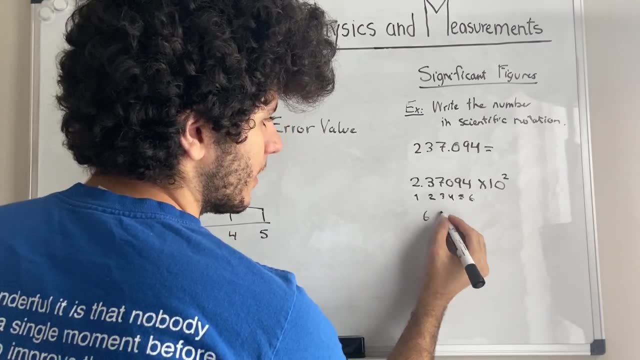 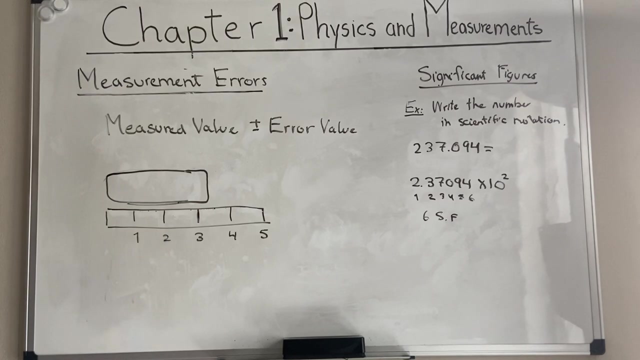 you see, that's what hands worries me. so if we're gonna try, then first we're gonna just multiply the number, break the science down to chapter two, since we don't have that much, guys, am I still there? what if we were? just like I wanna change the number. 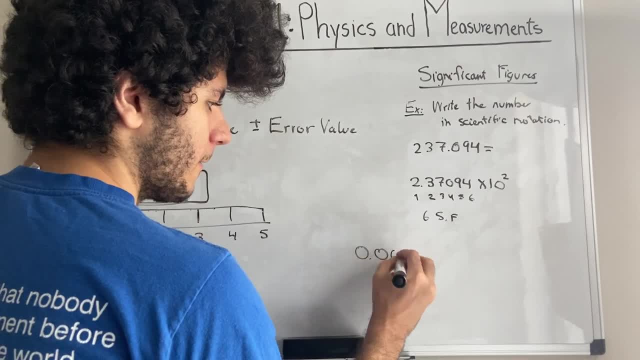 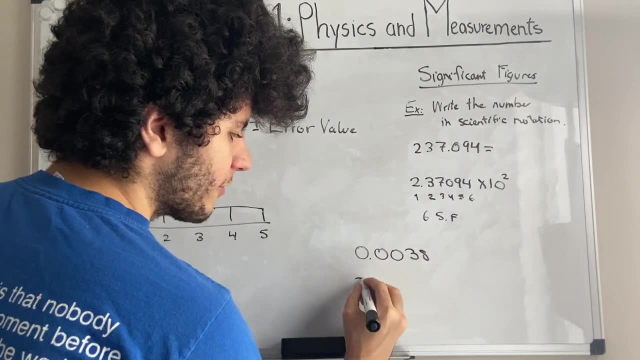 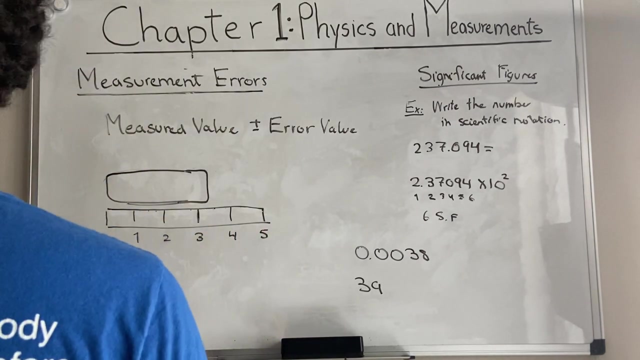 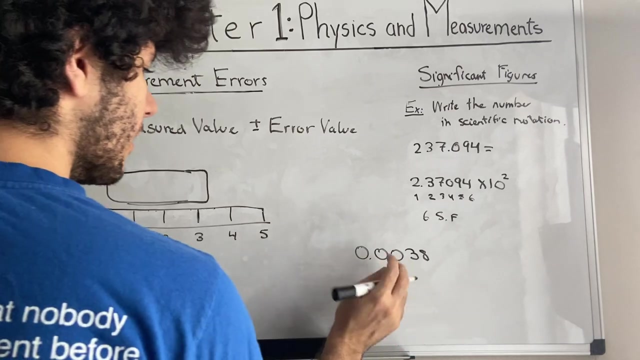 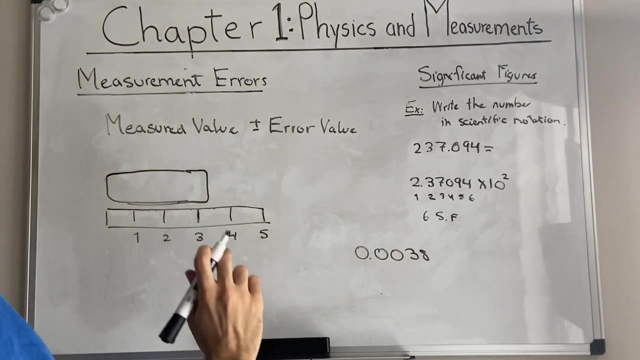 Zeros such as this, zeros not in the middle of the number, but rather before the number or after the number, like this. Hold on, let me just deal with this first example. If we have zeros that precede the other numbers, then we actually do not consider these ones. 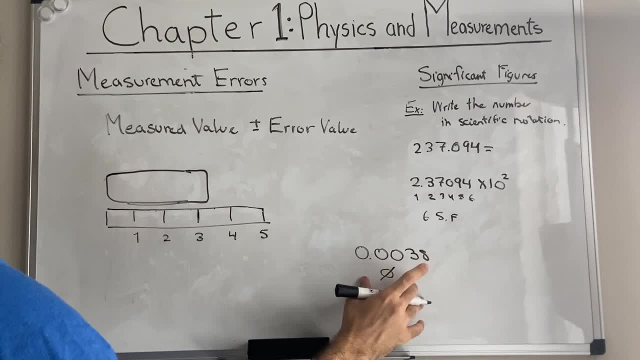 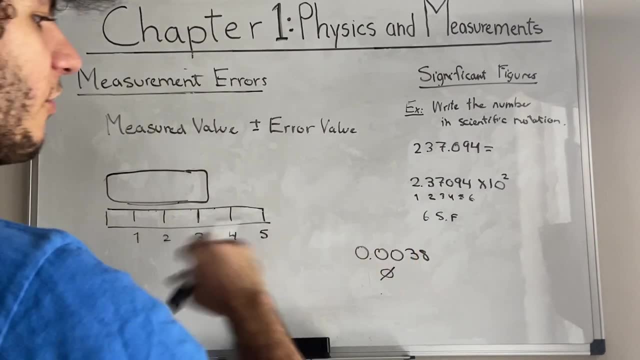 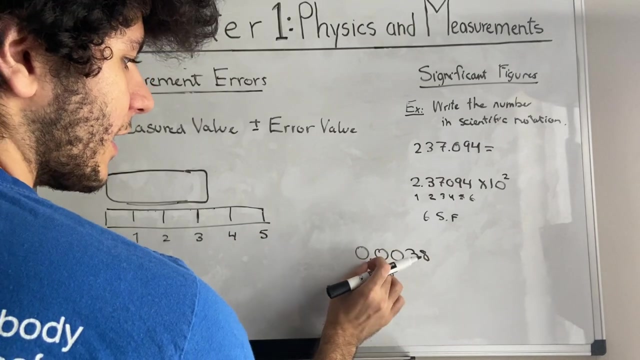 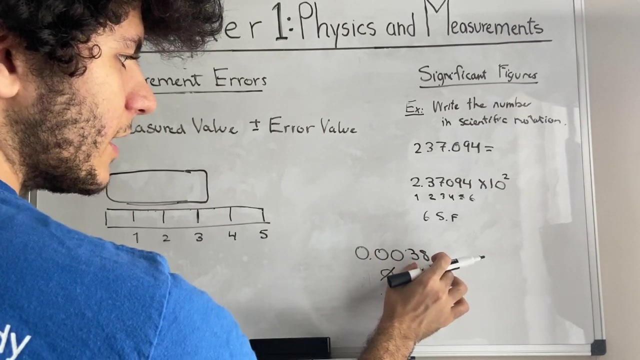 These ones are not considered as significant figures, And the reason being is that these just determine how far away from just like what position these numbers fall in. Basically saying that these 38 is not just, it's not 38. This is, it's a very, very, very small number. 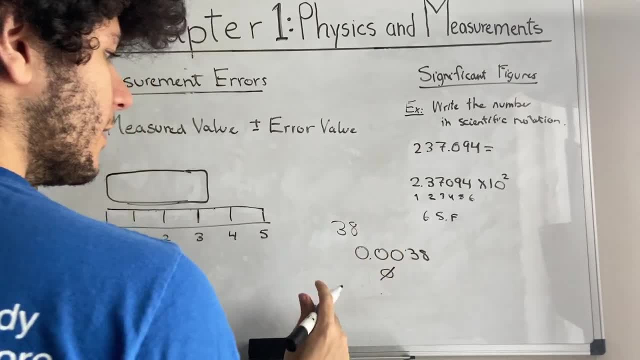 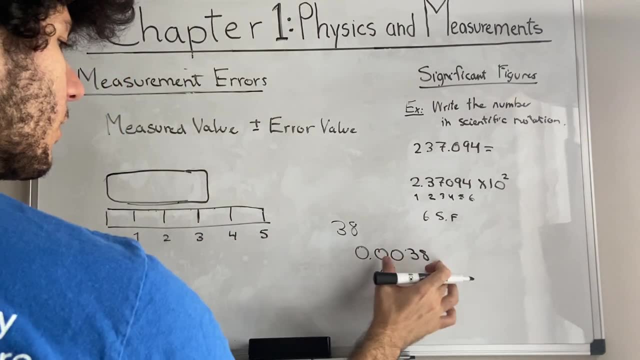 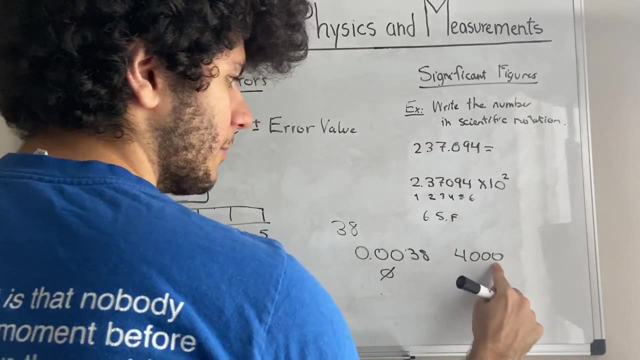 Instead, like if it was, if we just wrote 38, that would be much larger than this, And the zeros just help us figure out how small this number is right. On the other hand, if we had 4,000, these numbers are important. 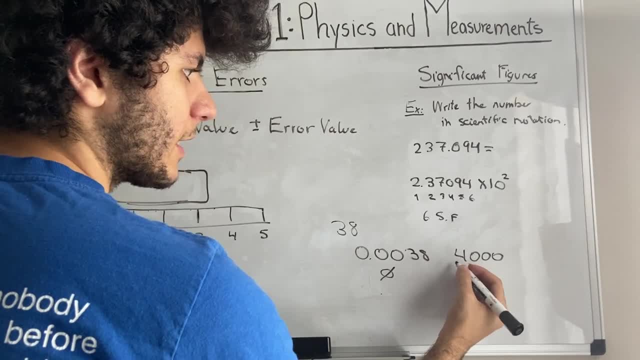 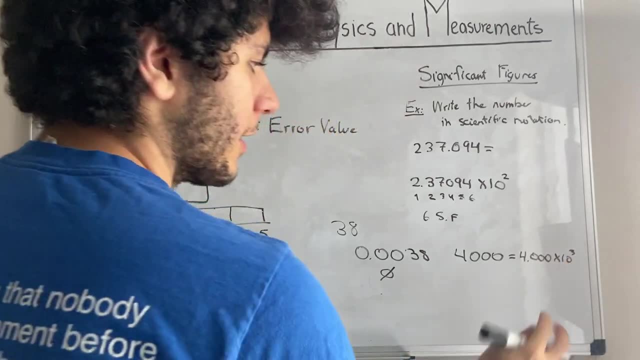 Because if we put this into Scientific notation it would be written as 4.000 times 10 to the negative, 3, times to the 3, right. So you see, these numbers could have been other numbers if they were not significant. 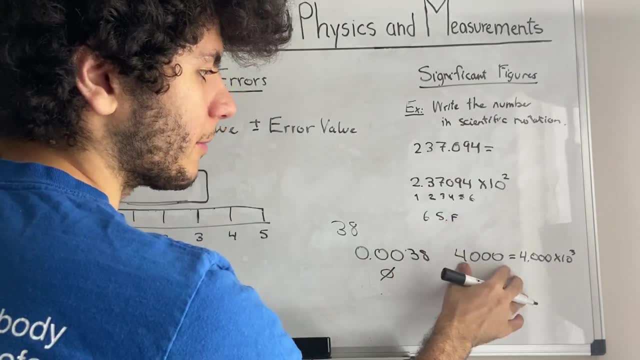 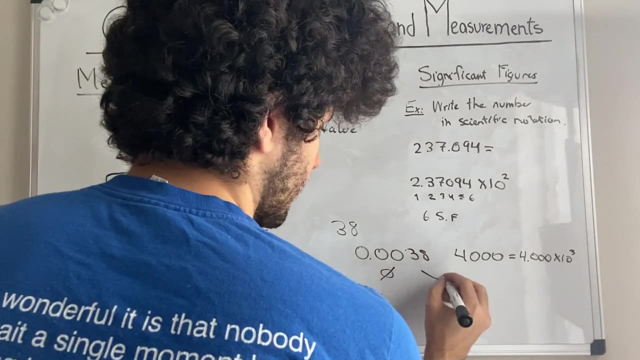 But they aren't. Or, and also, if these weren't significant numbers, then we wouldn't have written them here. Yeah, Same thing goes for this. We can also write this as 3.8 times 10 to the 1,, 2,, 3, negative 3.. 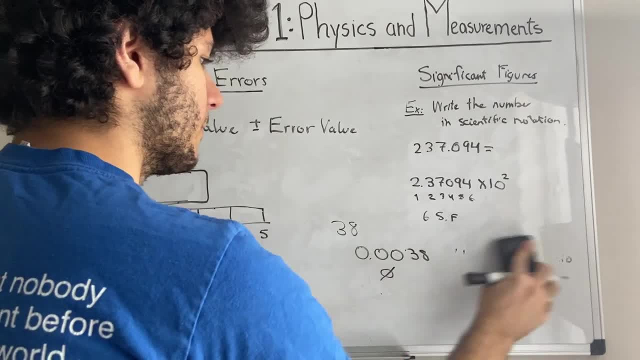 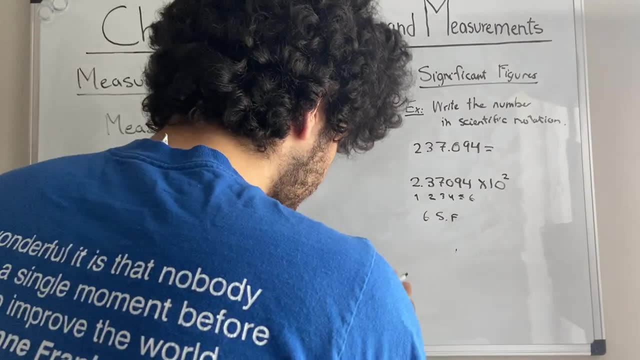 Right, But we don't. Well, actually, no, what am I saying? We do? Oh, we should. It's a better way of writing them, Especially if we're considering significant figures. Got something going on over here. I'll ignore that for now. 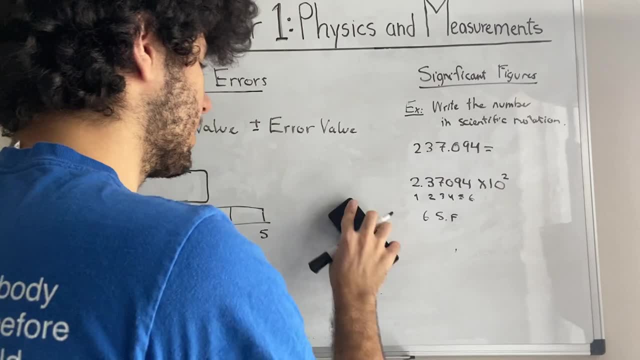 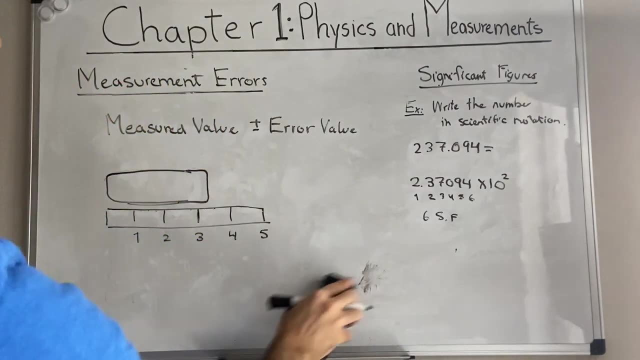 What am I saying We do? Oh, we should. It's a better way of writing them, Especially if we're considering significant figures. Got something going on over here. I'll ignore that for now, Okay. And when we're using measurement errors. 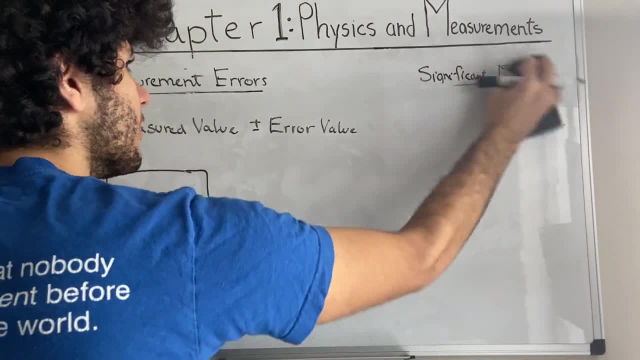 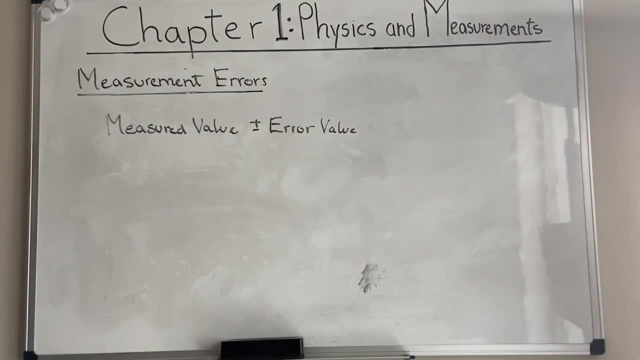 we actually have a way of determining how many significant figures there are in a number, And allow me to explain. If we have, say, a length of a road and the length of the road is measured to be 1,500 meters, 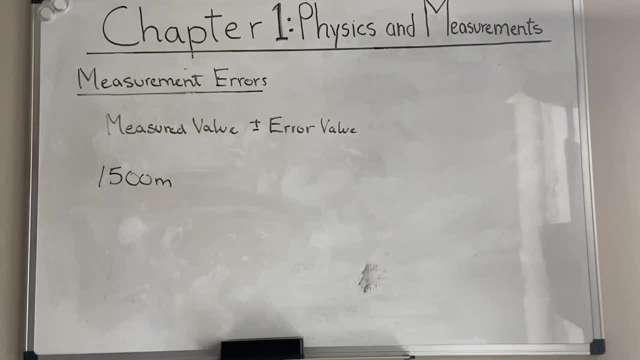 Depending on the error value, we will have a way of knowing how many significant figures we have in the number. So say, if this was 1,500 plus or minus 100, and I'm going to remove the unit and add it to the end. 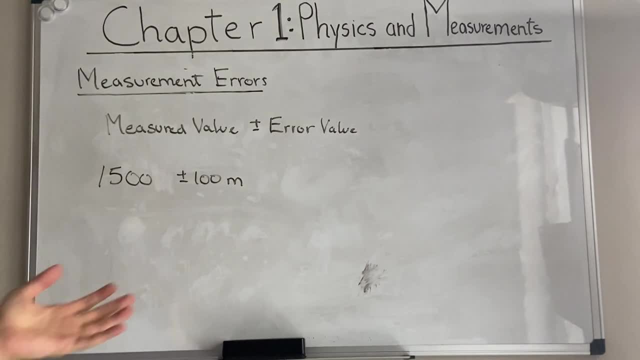 If we had this meaning. This is pretty inaccurate. Let's call this like someone just eyeballing the road to just guess how long it is. So if we eyeball it and we end up with this much uncertainty, then we basically have to understand that this number could go all the way down to 1,400 or go all the way up to 1,600. 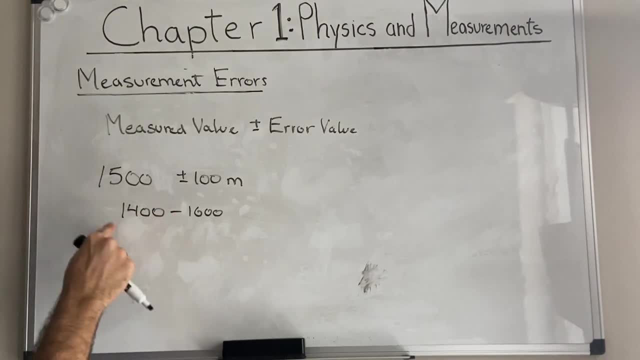 Right, That's what this is saying, If the number, the actual measurement, is somewhere in between these two numbers, But we'll never find out what, where exactly, And because we are, We can't be certain of these two digits like what they will be. 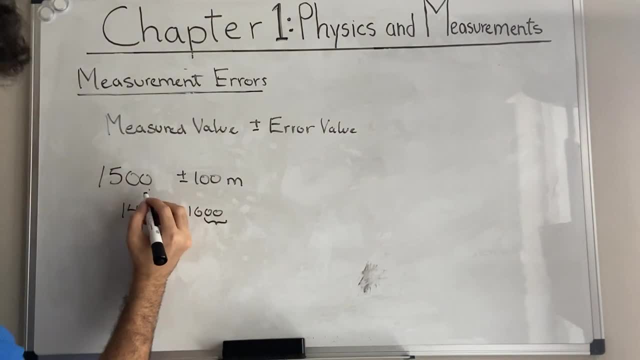 We're absolutely. we have no idea. These could, this could be one through nine, This could be one through nine. Well then, these are not significant figures. On the other hand, the five, though, one might say: well, these are not significant figures. 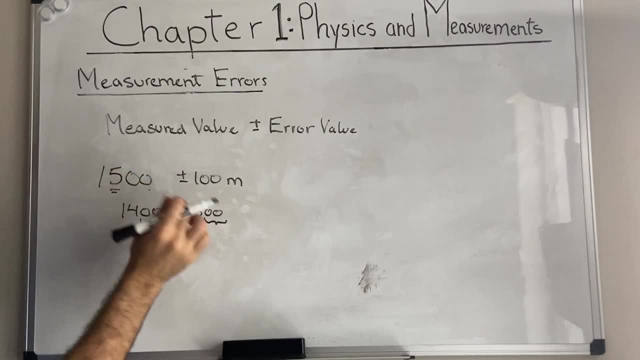 On the other hand, the five, though. one might say, well, these are not significant figures. One might say that, oh, it can be four, five or six. Well, we've actually trimmed the crowd. We have an idea. 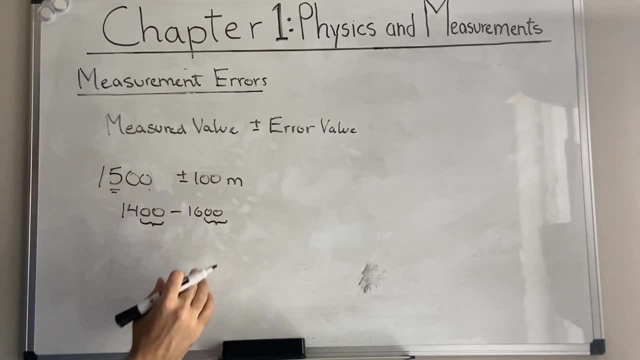 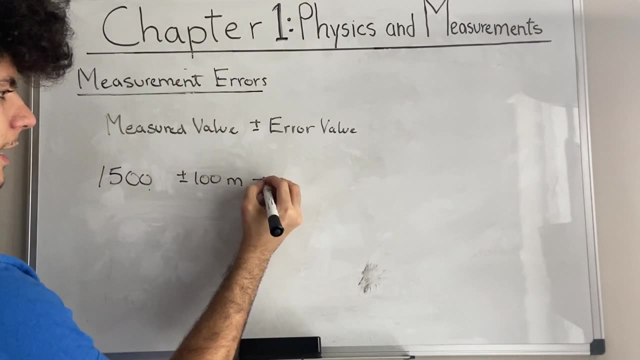 We have. we know that it's either between- it's either four, five or six, Meaning it's somewhat certain. So that will be the first of our significant figures. So this situation we have, this could be written as as such. 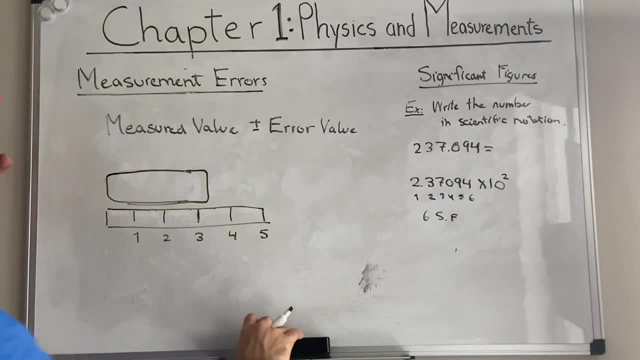 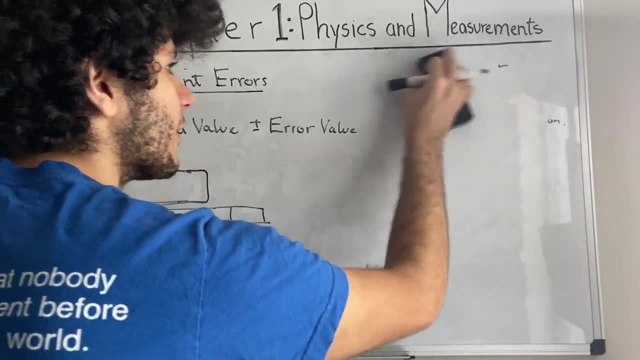 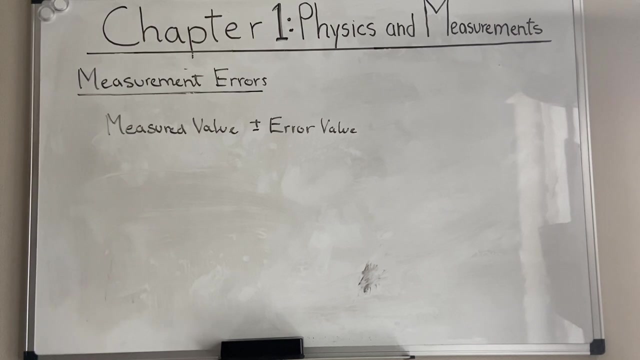 Okay, And when we're using measurement errors, we actually have a way of determining how many significant figures there are in a number. And allow me to explain. If we have, say, a length of a road, And the length of the road is measured to be 1,500 meters, 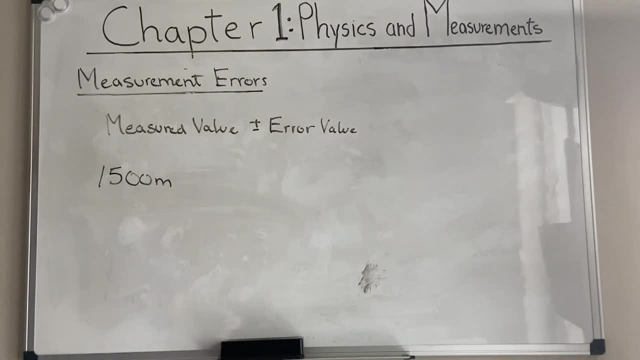 Depending on the error value, we will have a way of knowing how many significant figures we have in the number. So say, if this was 1,500 plus or minus 100, and I'm going to remove the unit and add it to the end. 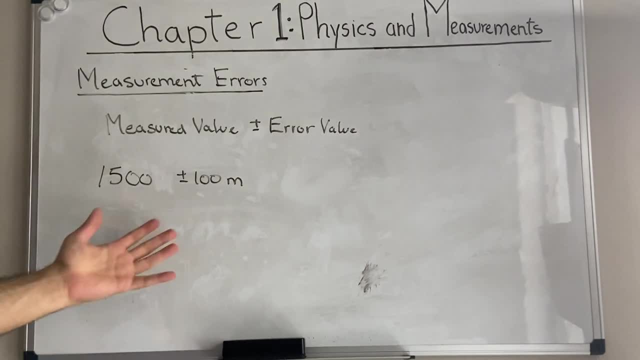 If we had This Meaning. this is pretty inaccurate. Let's call this like someone just eyeballing the road to just guess how long it is. So if we eyeball it and we end up with this much uncertainty, then we basically have to understand that this number could go all the way down to 1,400 or go all the way up to 700. 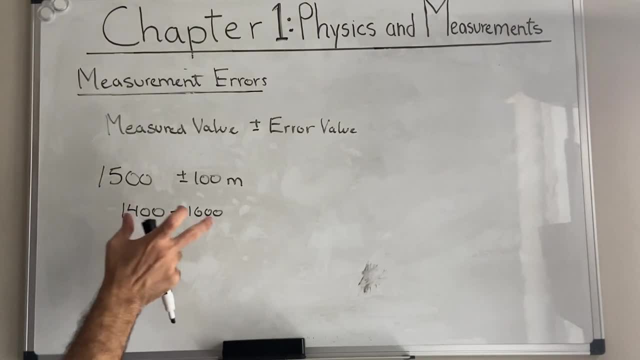 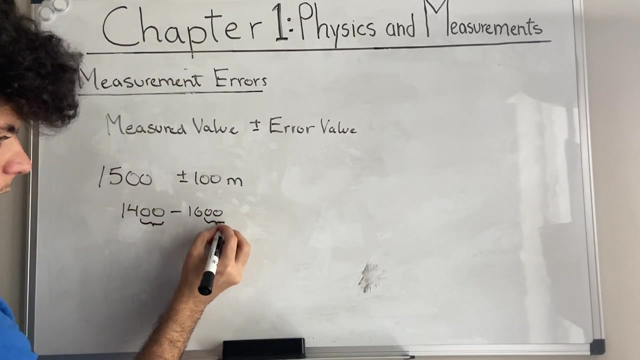 Right, That's what this is saying, If the number, the actual measurement, is somewhere in between these two numbers, but we'll never find out what, where exactly, And because we are, we can't be certain of these two digits like what they will be. 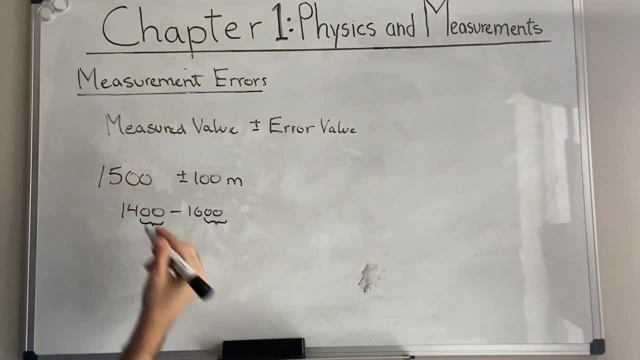 We're absolutely, we have no idea. These could, this could be one through nine, This could be one through nine. Well then, these are not significant figures. On the other hand, the five, The five, Though one might say that, oh, it can be four, five or six. 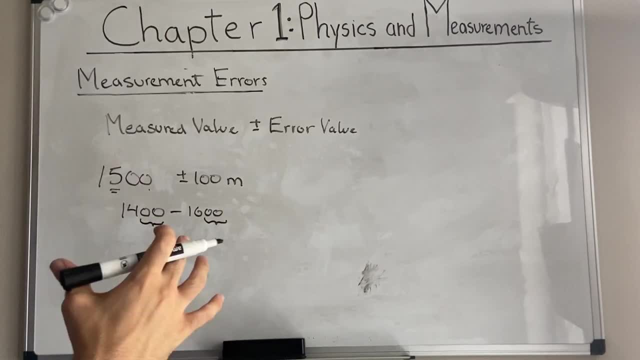 Well, we've actually trimmed the crowd. We have an idea, We have, we know that it's either between. it's either four, five or six, meaning it's somewhat certain. So that will be the first of our significant figures. 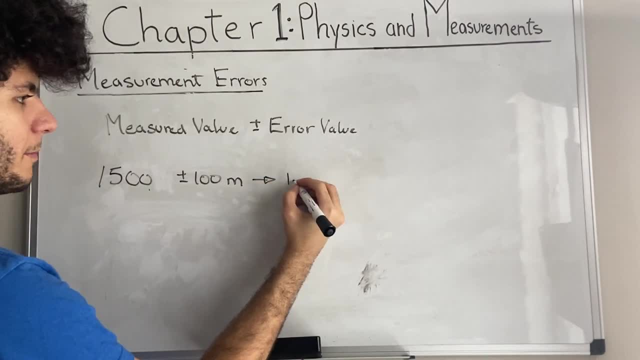 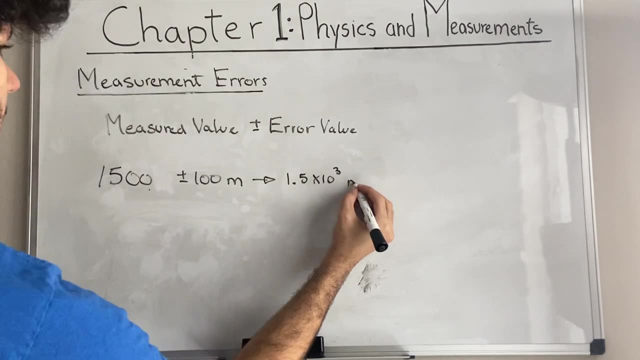 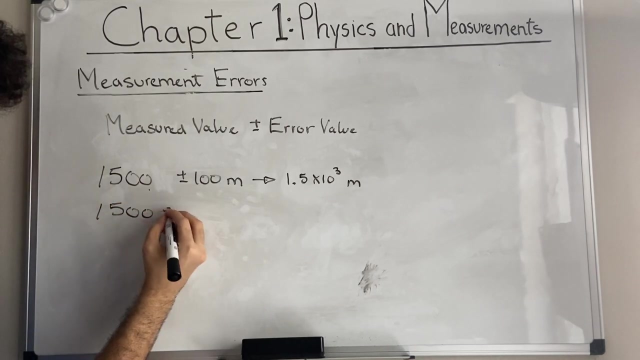 So this situation we have, this could be written as as such: One, two, three meters. So you basically have two. You have two significant figures. If we wrote this as 1500 plus or minus 10 meters, then we're dealing with a bit of a different situation. 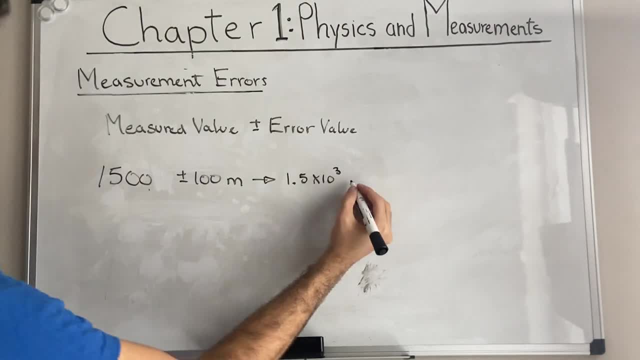 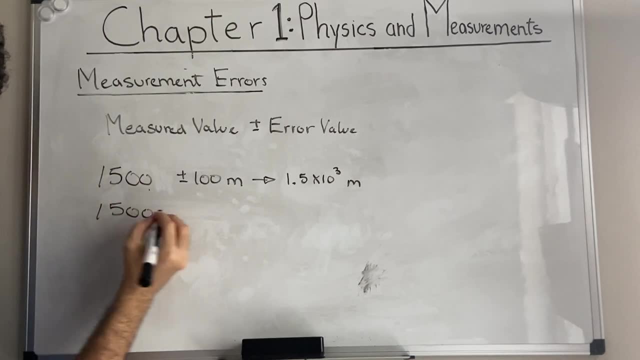 One, two, three meters. So you basically have two significant figures. If we wrote this as 1500 plus or minus 10 meters, then we're dealing with a bit of a different situation. We know that the 1500, the one, the five will always stay the same. 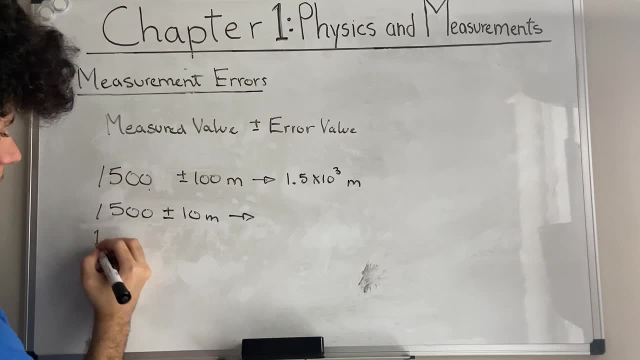 The zero will either be- well, actually, the one will always stay the same- The five can either be a five or a four, And then the zero will either- Oh, it's a four- be a one or a nine. right, well, actually, it can also be a zero if it's exactly on. 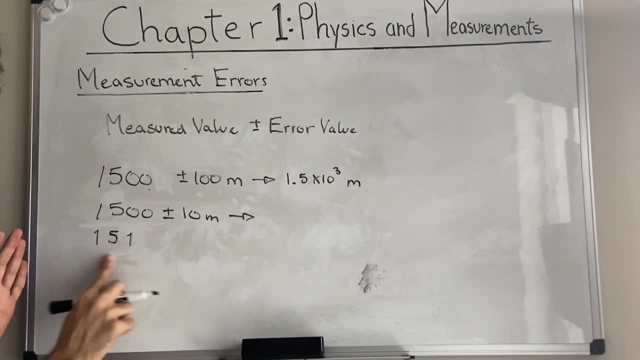 the spot, but basically this: this is basically how far it can reach. these are like the limits: you can either go up by one or go down by one, and because of that we have an idea of what this number can be. it can be as small as 1490 and as 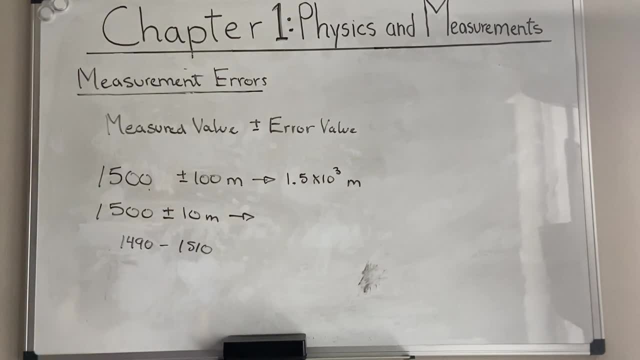 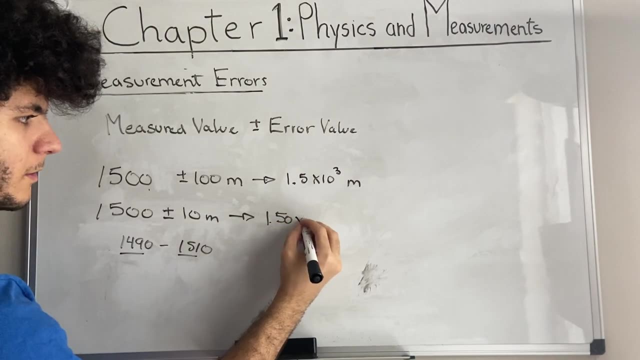 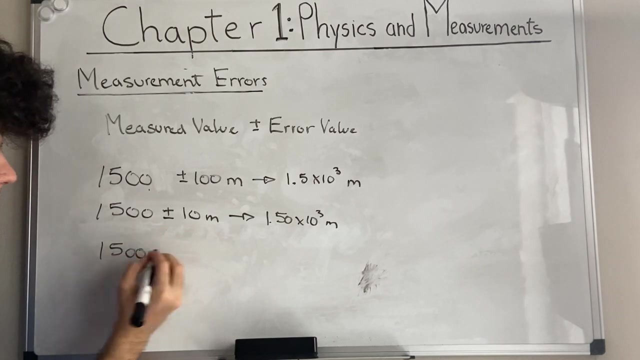 high as 1510. therefore, we have an idea for these three numbers. so we have three significant figures and if you follow this pattern, if we were to say that someone measured the road with a one meter inaccuracy, then well, error value, then we would have this: 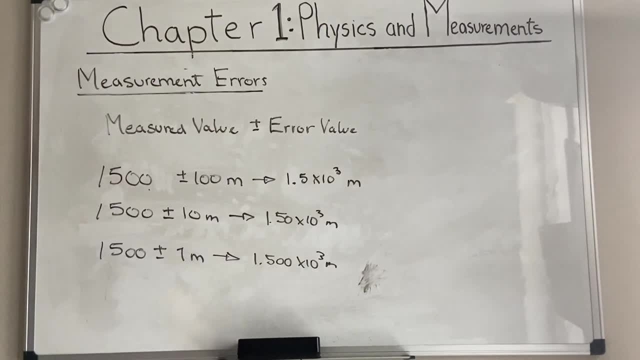 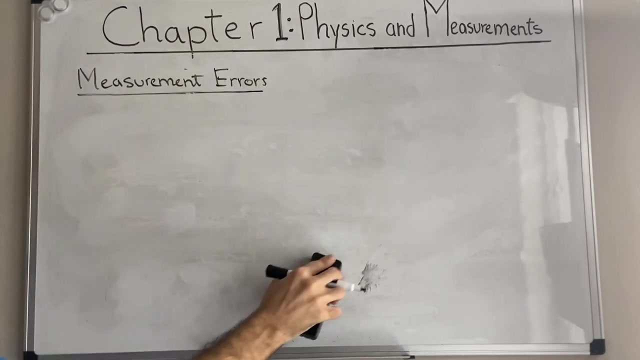 this being four significant figures, which is an excellent measurement, I would say at least. all right, let's see. yes, so in our lecture, basically every single other video I will be making, we will not really be concerned by error, measurement errors, because they take up a little bit too much time and they're a 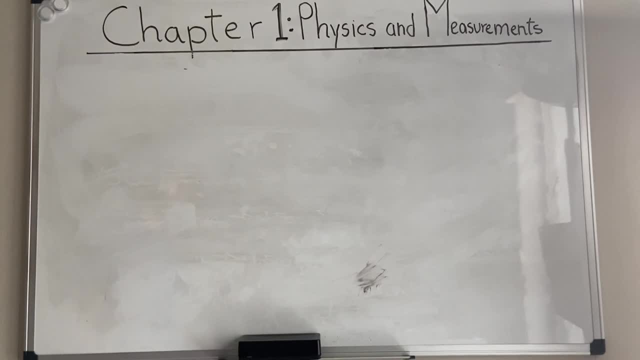 little bit off, like the point of physical well, at least in the class, which will be just to learn the concepts and apply them properly in every problem, and I would say that one good, two good rules for, like our lecture, will be to round off only at the end of the calculation. 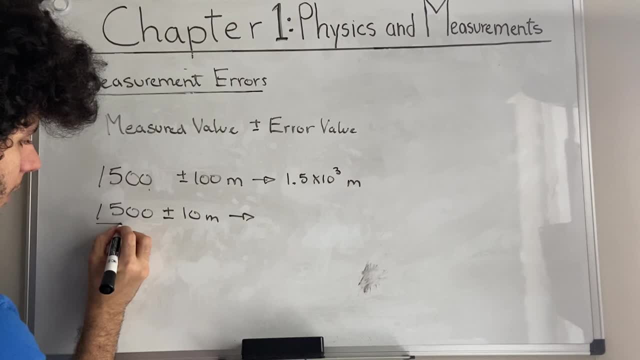 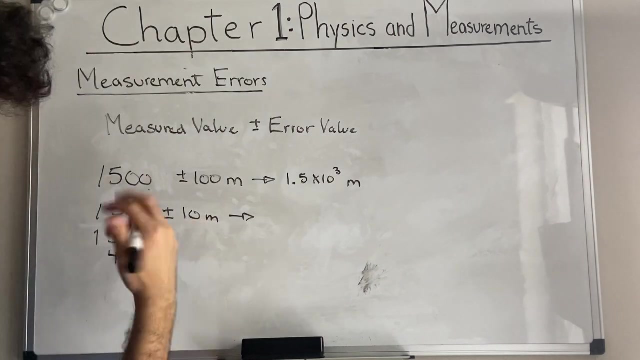 We know that the 1500, the one and the five will always stay the same. The zero will either- be- well, actually, the one will always stay the same- The five can either be a five or a four, And then the zero will either be a one or a nine right. 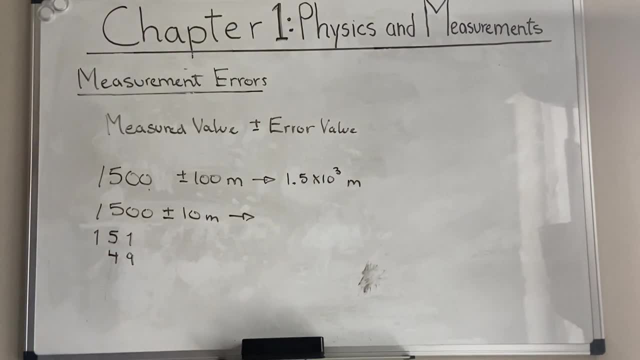 Well, actually it can also be a zero if it's exactly on the spot, But basically, this is basically how far it can reach. These are like the limits: It can either go up by one or go down by one, And because of that, we have an idea of what this number can be. 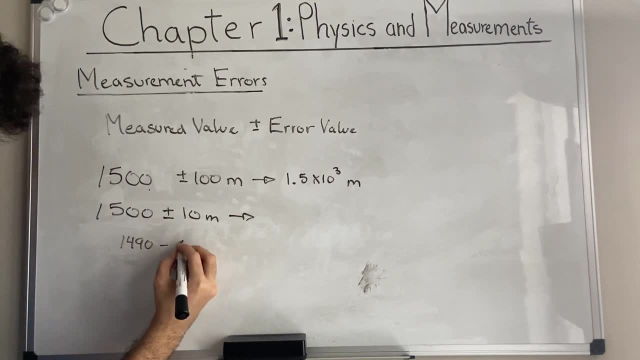 It can be as small as It can be as small as 1490 and as high as 1510.. Therefore, we have an idea for these three numbers. So we have three significant figures And if you follow this pattern, if we were to say that someone measured the road with a one meter inaccuracy, 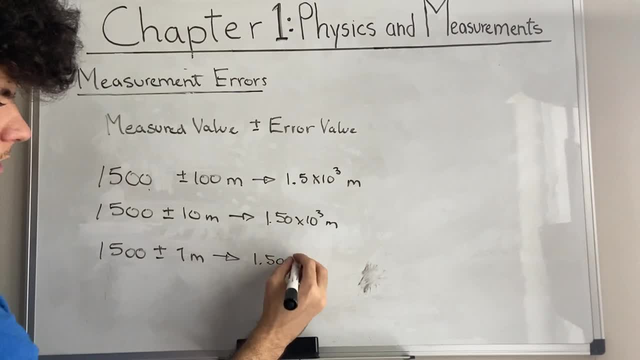 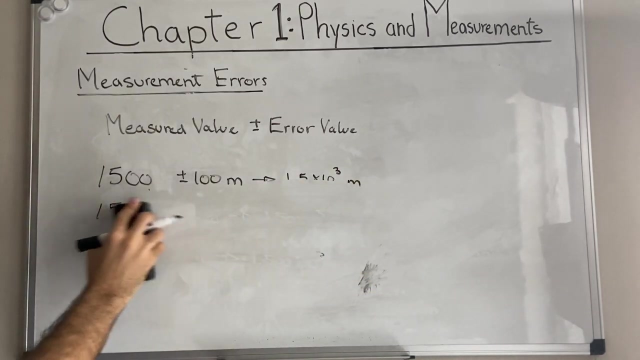 well, error value, then we would have this, This being four significant figures, which is an excellent measurement, I would say at least. All right, Let's see. Yes, So in our lecture, basically every single other video I will be making. 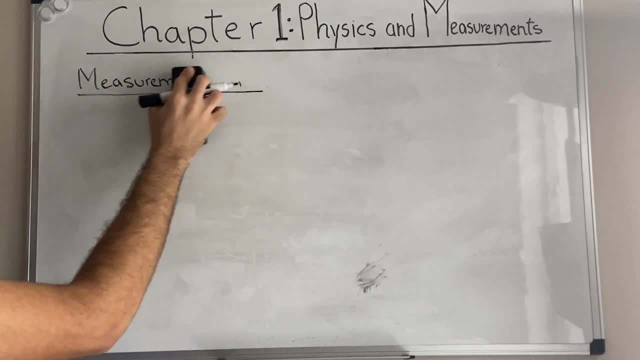 we will not really be concerned by error measurement errors because they take up a little bit too much time and they're a little bit off, like the point of physics. well, at least in the class, which will be just to learn the concepts and apply them properly in every problem. 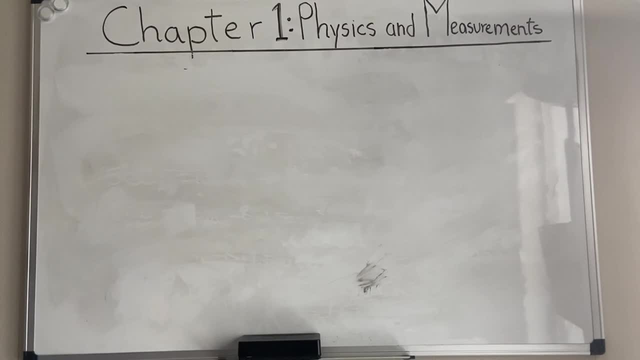 And I would say that one good, two good rules for like our lecture will be to round off only at the end of the calculation to make sure that we have, like, the numbers that we have are as legitimate as possible, And we'll actually try to keep at least three decimal places in that answer. 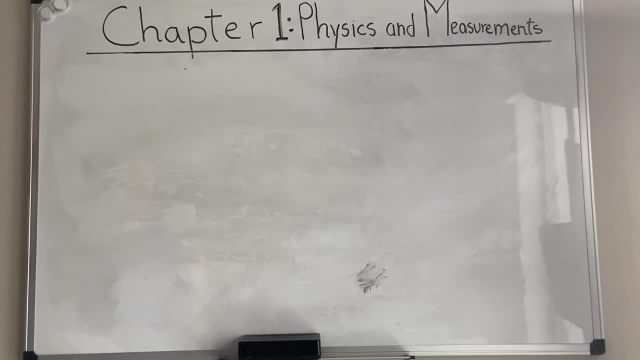 to make sure that we have isn't like the numbers that we have are as legitimate as possible, and we'll actually try to keep at least three decimal places in that answer. one final thing that we're going to talk about is the number of we're gonna go over in chapter one is mass density, which starts to this is: 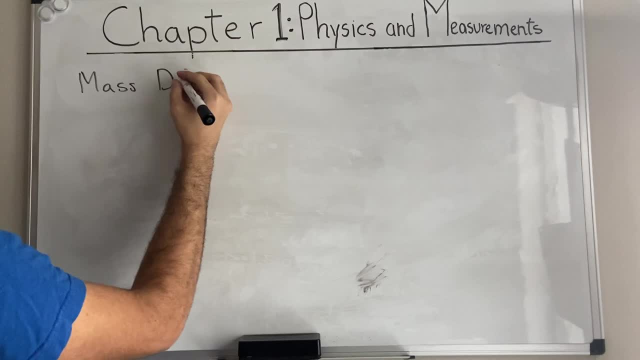 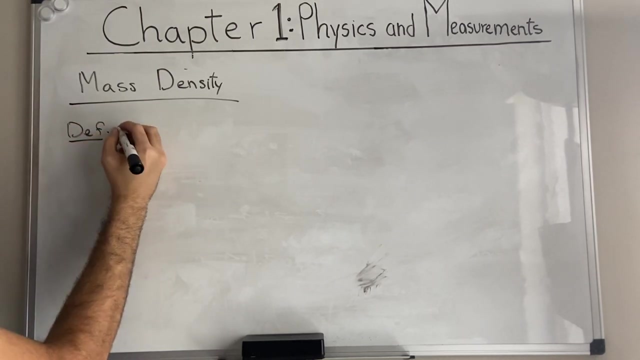 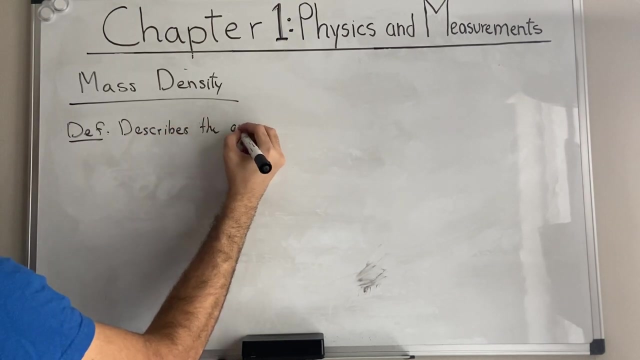 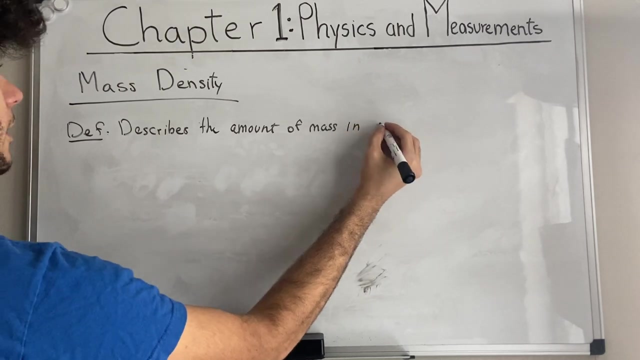 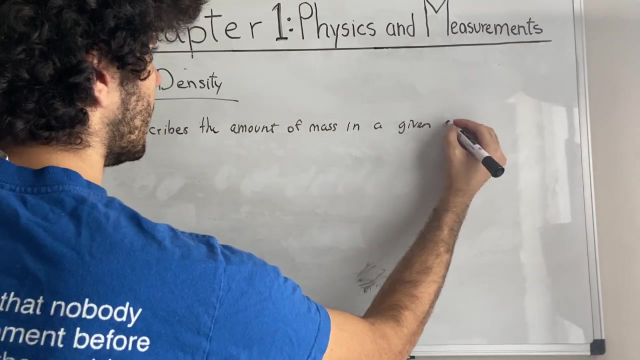 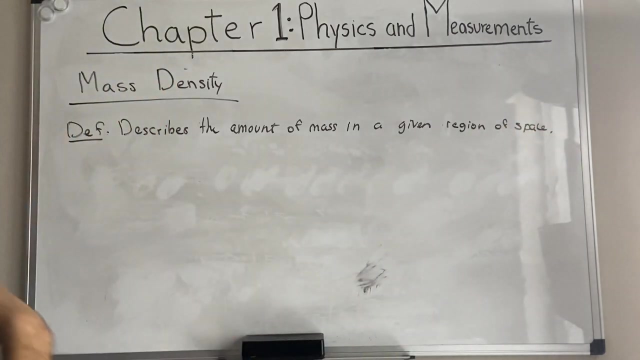 starting to be a topic that we will be dealing with much later in chapter 10: mass density. mass density is basically, basically allows us to describe. it describes the amount of mass of mass in a given region, region of space. without a doubt, you've already heard of this idea, basically. 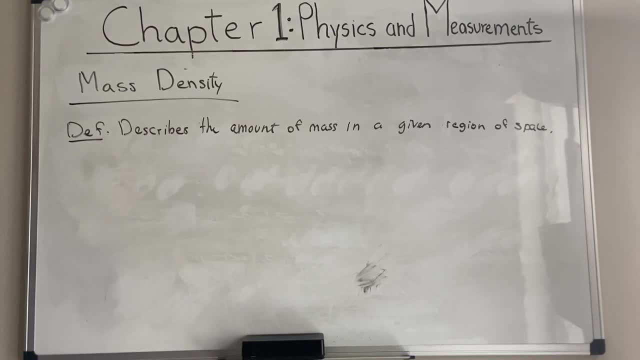 something that's you've probably already dealt with the situation. if you have something that's very dense and you throw it in the pool, it will sink because its density is higher than the water. on the other hand, if you have something that's not very dense, it will actually float on the water because its 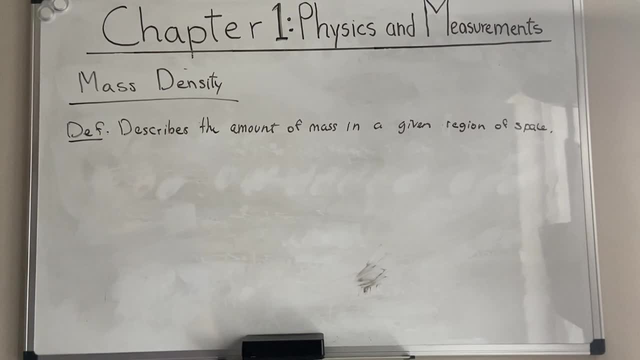 density isn't as high. um so, basically what that means, and if if you're familiar with that idea, density has nothing to do with how big an object is. you can have a small cube of metal which has higher density than a big cloud of cotton candy, because there's a lot of air in this and it's a lot more compact. 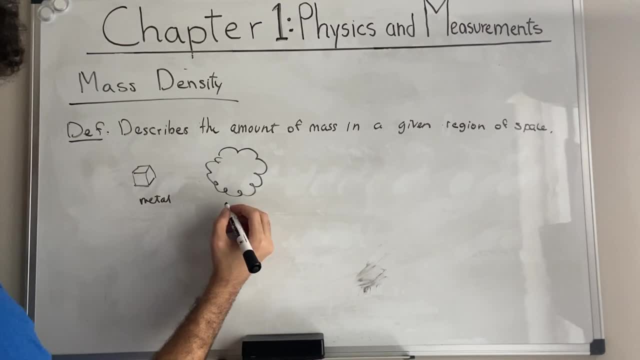 and metal generally has a higher density. so, um, we can call this cotton candy, I guess. and the way that we write mass density, at least in terms of volume, volume mass density. and the way that we write mass density, at least in terms of volume, volume mass density. 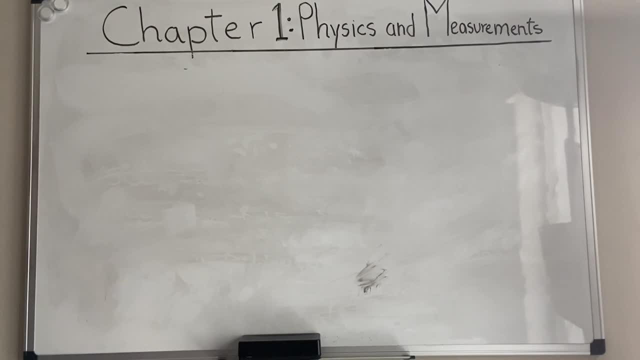 One final thing that we're going to go over in Chapter one is mass density, which starts to. this is starting to be a topic that we will be dealing with much later In Chapter 10, mass density. Mass density is basically, basically. 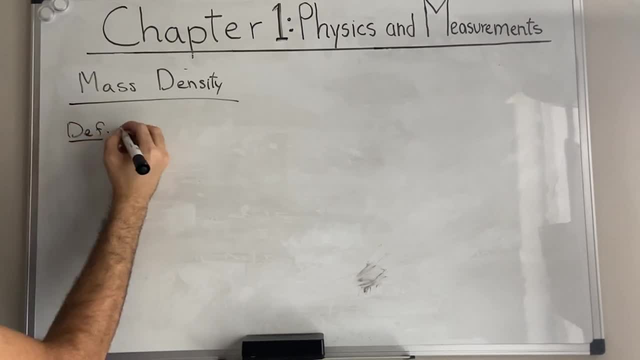 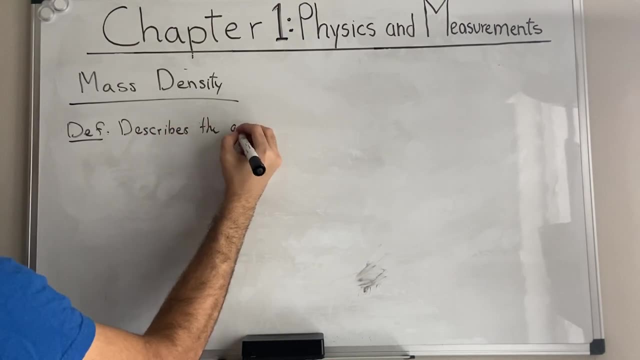 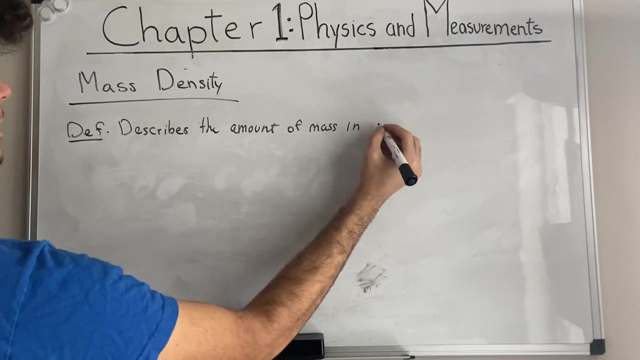 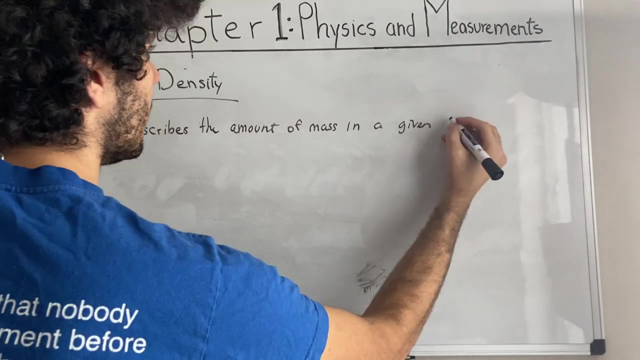 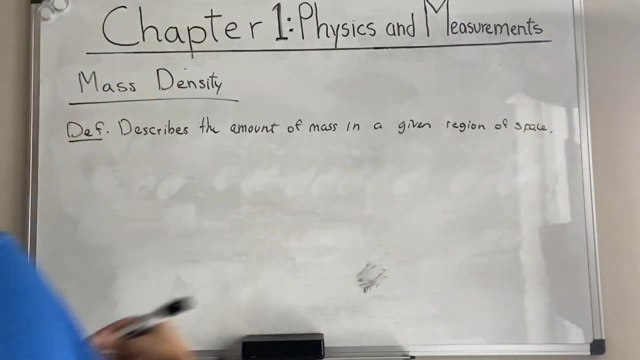 allows us to describe. it describes the amount of mass, of mass in a given region, region of space. Without a doubt, you've already heard of this idea, Basically something that's you've probably already dealt with the situation: If you have something that's very dense and you throw it in the pool. 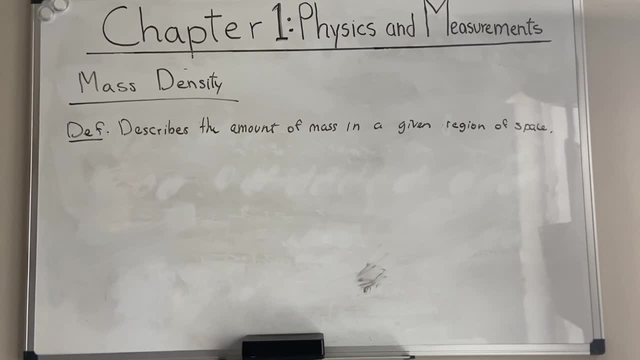 it will sink because its density is higher than the water. On the other hand, if you have something that's not very dense, it will actually float on the water because its density isn't as high. So basically what that means, and if 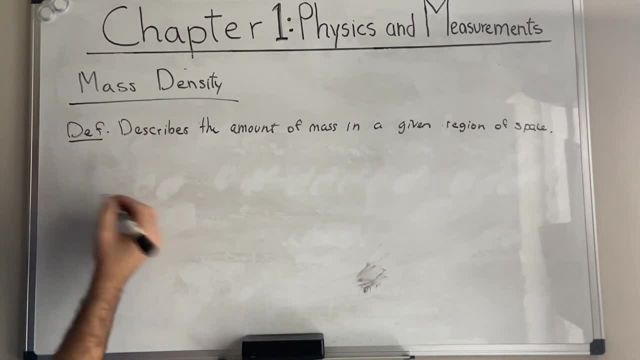 if you're familiar with that idea. density has nothing to do with how big an object is. We can have a small cube of metal which has higher density than a big cloud of cotton candy, because there's a lot of air in this and it's a lot more compact, and metal generally has a higher density. 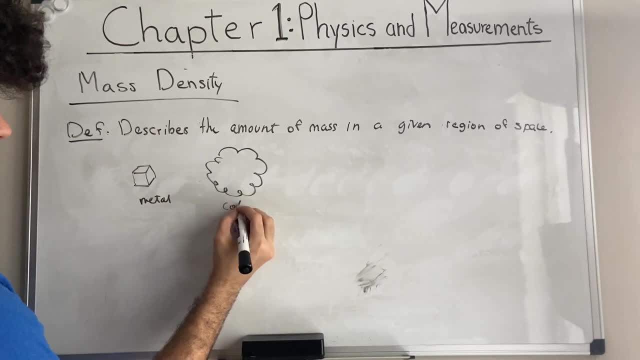 So, um, we can call this cotton candy, I guess Candy. And the way that we write mass density, at least in terms of volume, volume mass density is with this letter, which is rho, And we can say that this one, 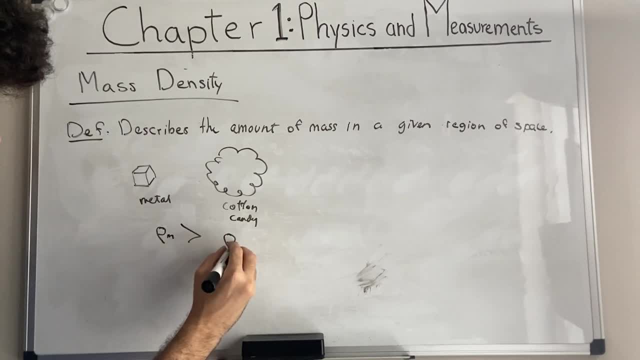 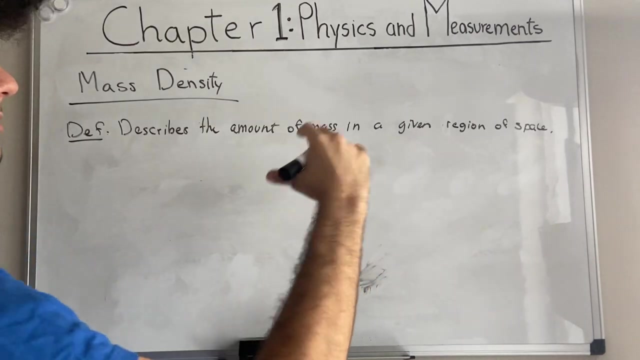 m is larger than p, rho of c, Rho of m is larger than rho of c, But anyways, it's basically a density. mass density is a ratio that connects usually volume and mass, And this definition just says region of space. 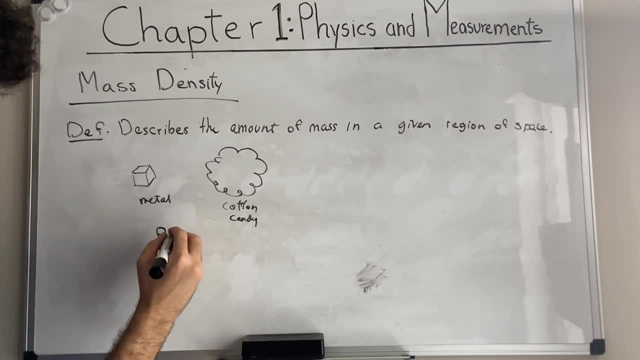 is with this letter, which is rho, and we can say that this one of m is larger than a rho of c. rho of m is larger than rho of c, but anyways, it's basically a density. mass density is a ratio that connects usually volume and mass, and this definition 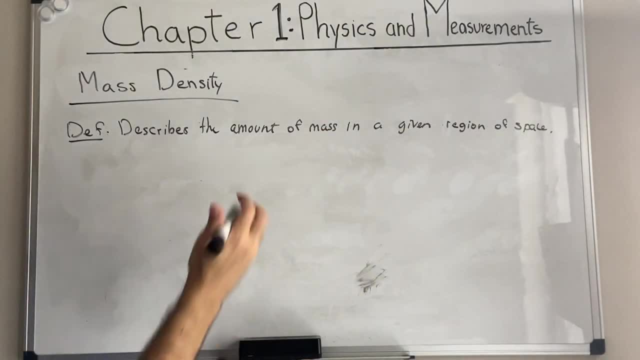 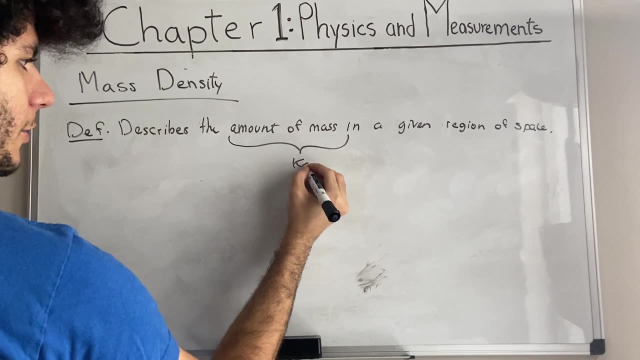 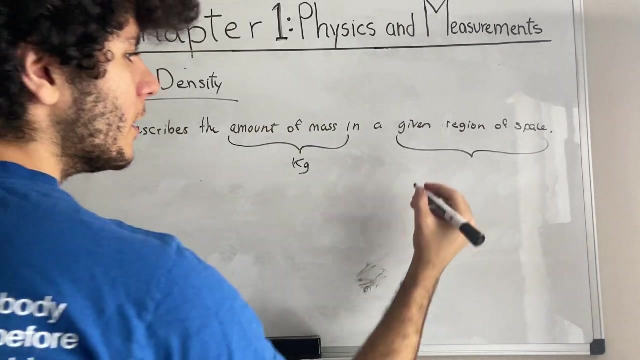 just says region of space and you're going to see why in a second. but basically um amount of mass, that's our kilogram right and a given amount of space. you might be tempted to just say meters cubed, but actually it can be meters, meters squared or meters cubed. 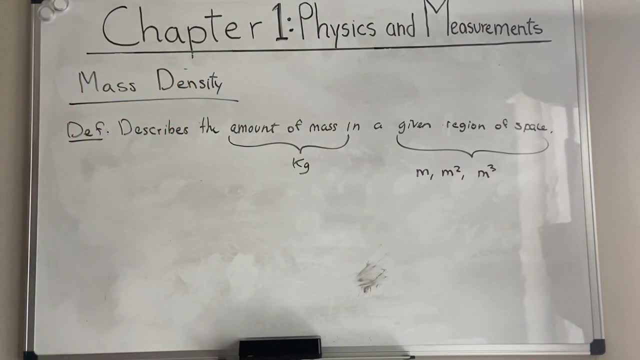 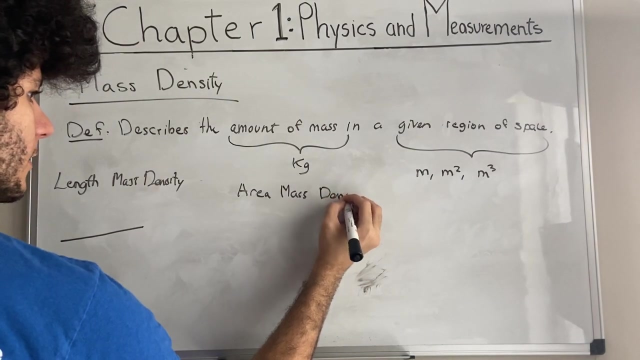 and we're gonna see how right now. um so, basically, we have three different types of mass density. we have the length- mass density, mass density, which is which- let me just write this. then we have the area mass density- mass density, mass density. next, we have the volume mass density. 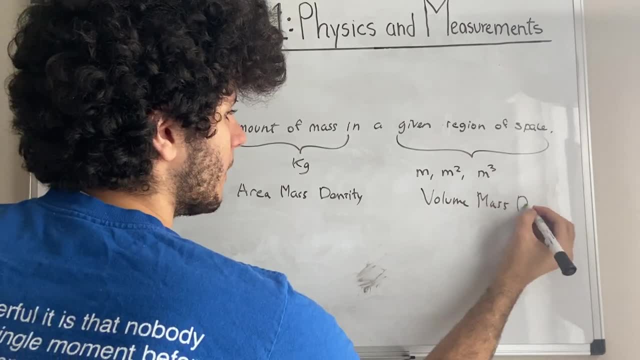 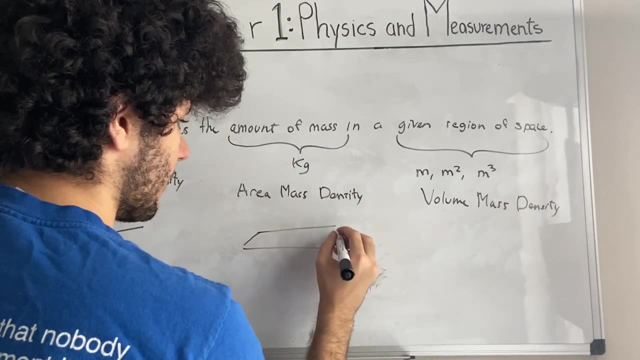 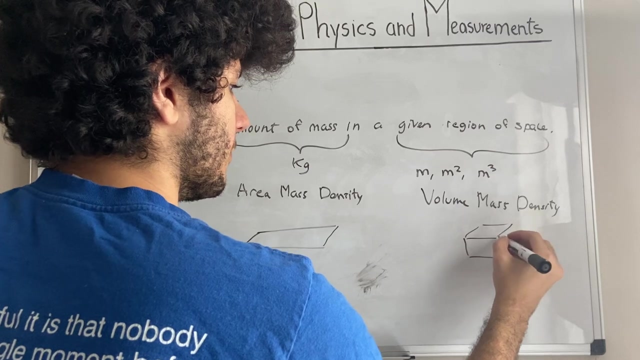 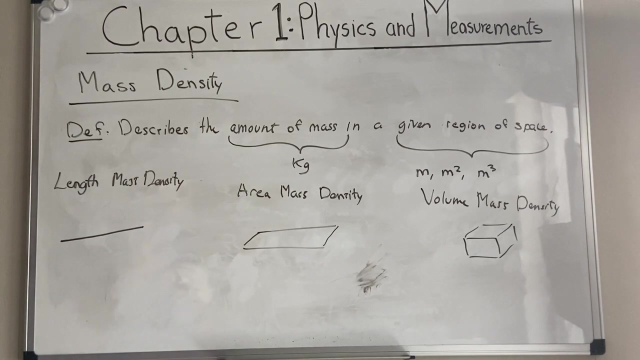 which is something that everyone is more familiar with. let me just draw something so that we can understand this a little bit better. this is a plate, and here we'll have a little volume, a little block of something. let's call that a brick, maybe, all right. so, basically, in every situation, for every given region of space, for this portion of space, 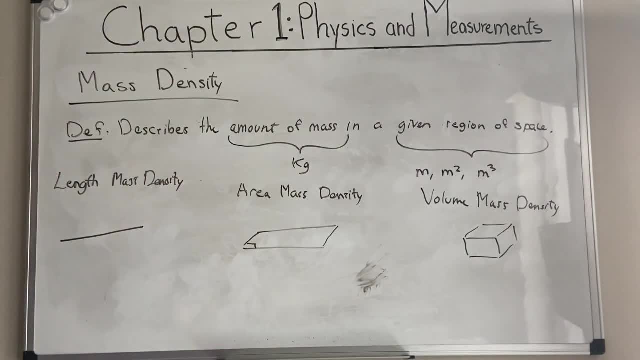 there is a certain amount of mass right, and that mass is not necessarily the same everywhere in this plate. one side of the plate might be constructed of a material that's much more well. no, actually let's say it's constructed the same material. it's much more complex. you might be in a particular place, you mightirella. there's a lot of wrong places to go around the other side of the plate. there might be construction over the other side. you might certainly be having problems if you have a lot community over the plate, right. so 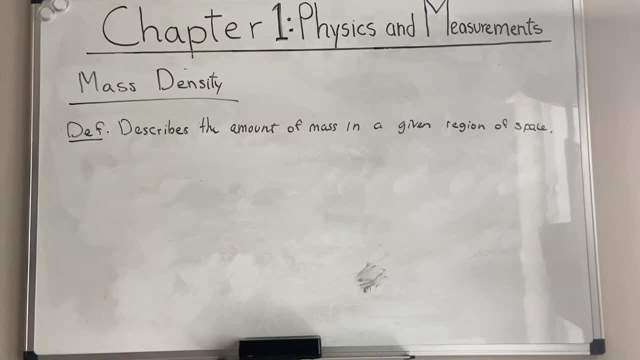 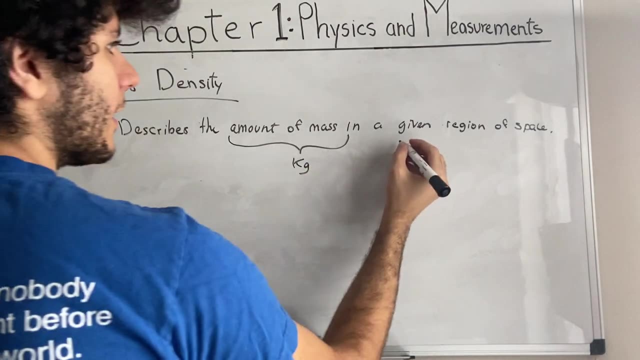 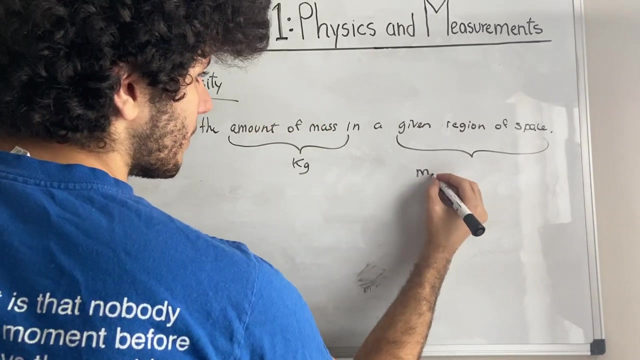 and you're going to see why in a second. But basically um amount of mass, that's our kilogram right And a given amount of space. you might be tempted to just say meters cubed, but actually it can be meters. 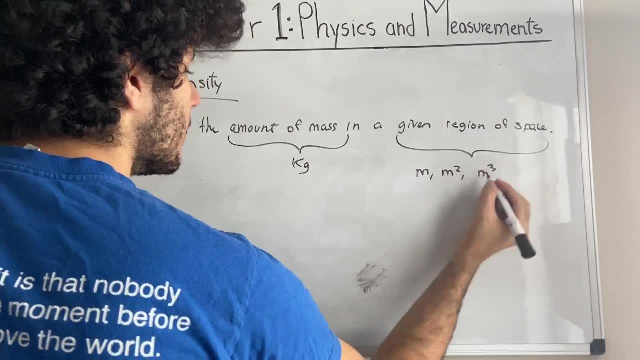 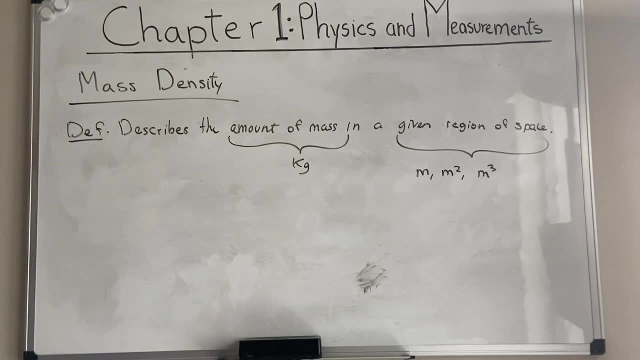 meters squared or meters cubed, And we're going to see how right now. Um so, basically, we have three different types of mass density. We have the length mass density, mass density which is which? let me just write. 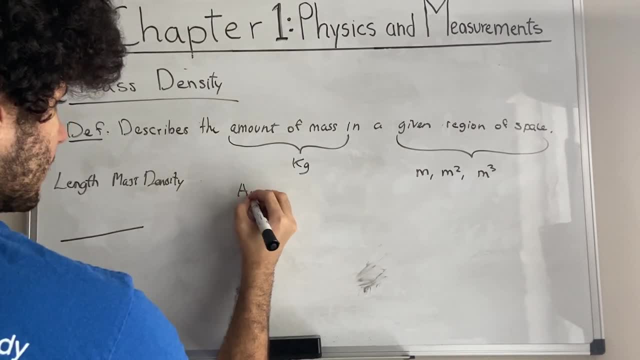 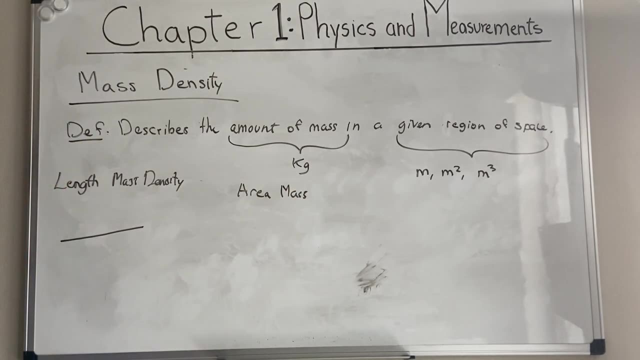 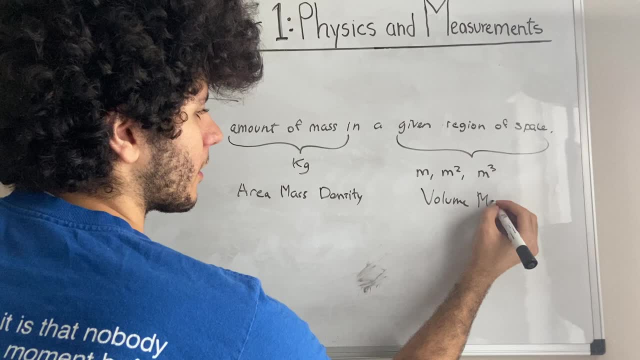 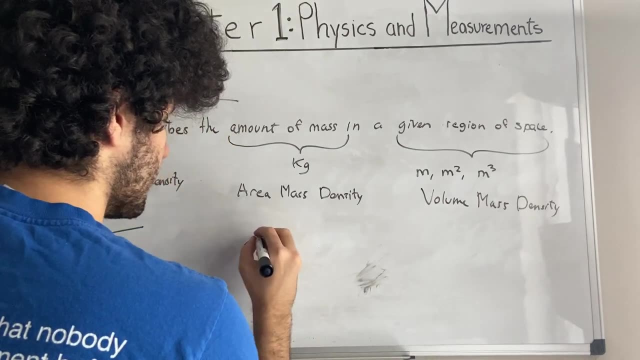 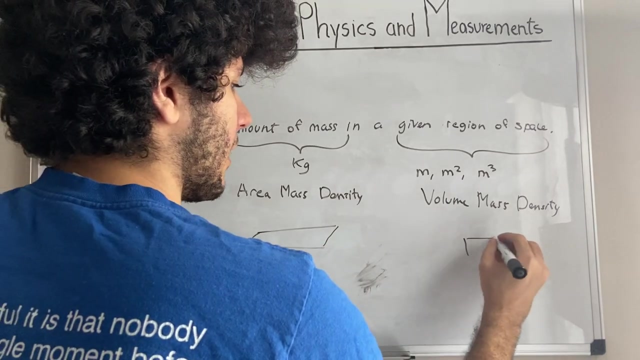 which is something that everyone is more familiar with. Let me just draw something so that we can understand this a little bit better. This is a plate, And here we'll have a little volume, a little block of something. Let's call that a brick. 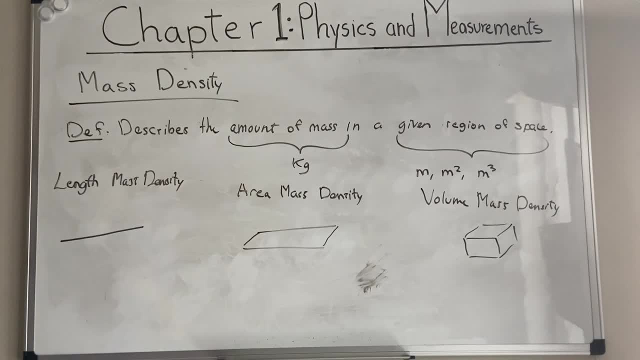 maybe All right. So basically, in every situation, for every given region of space, for this portion of space, there is a certain amount of mass right, And that mass is not necessarily the same everywhere. In this plate, one side of the plate might be constructed of a material that's much more. 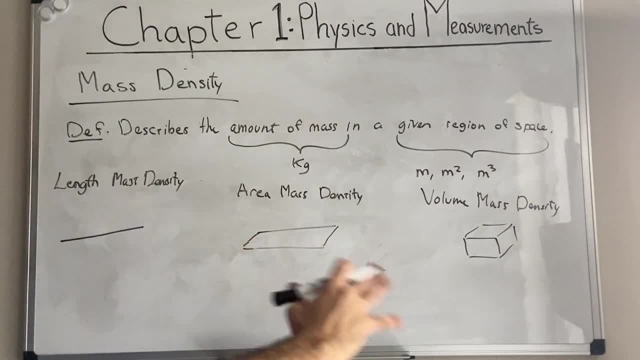 well, no, actually, let's say it's constructed the same material everywhere. It might be more compact and dense in certain areas, though it doesn't show in its volume. It's very, very thin but very heavy, And the other side might be very light. 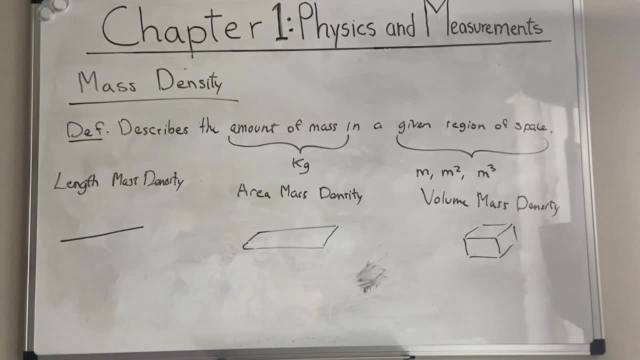 as though there's little mass, There's no mass And in a given in a large volume, right, And that applies in all three scenarios. In this scenario, this looks like just a line, but and it is a line. 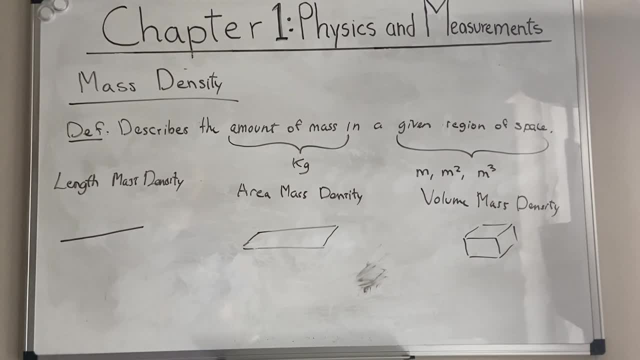 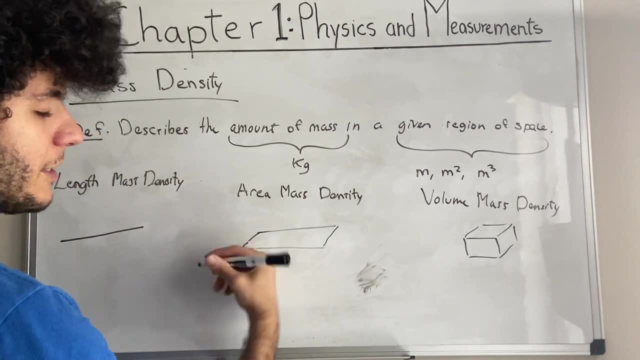 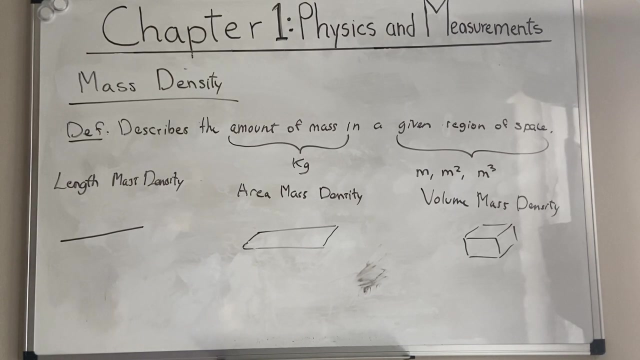 material everywhere. It might be more compact and dense in certain areas, though it doesn't show in its volume. It's very, very thin but very heavy, And the other side might be very light, as though there's little mass. There's no mass and in a given in a large volume, right, And that applies. 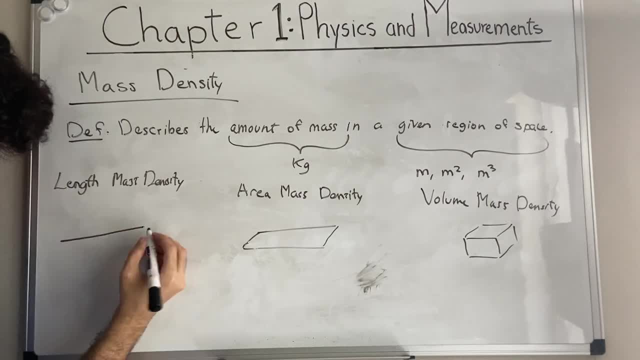 in all three scenarios. In this scenario this looks like just a line, but- and it is a line, but there could be a large amount of mass here. I guess let's put arrow up mass, and then over here, low mass. And over here let's say this low mass as well, Let's say that this is very heavy. 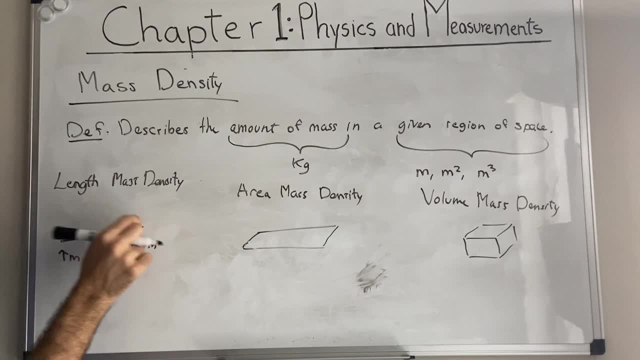 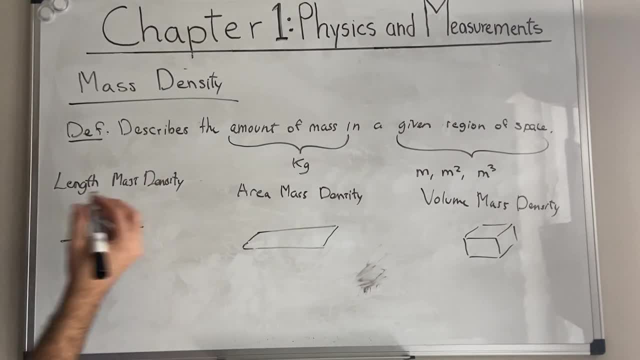 are just for different dimensions. Here we have a 1D situation, Here we have a 2D situation, Here we have a 3D situation. In this situation we're basically dealing with, like a paper, a scene from the side. Let me grab one really quick. If you look at a sheet of paper, it's very thin from. 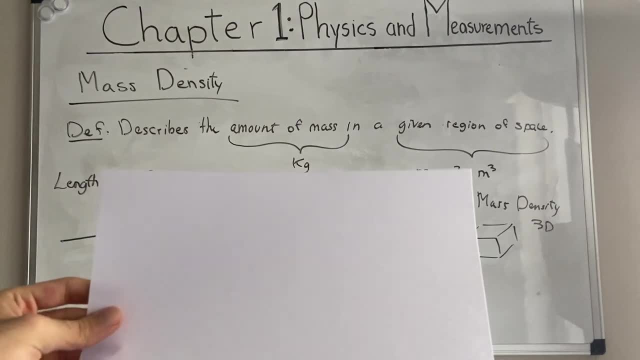 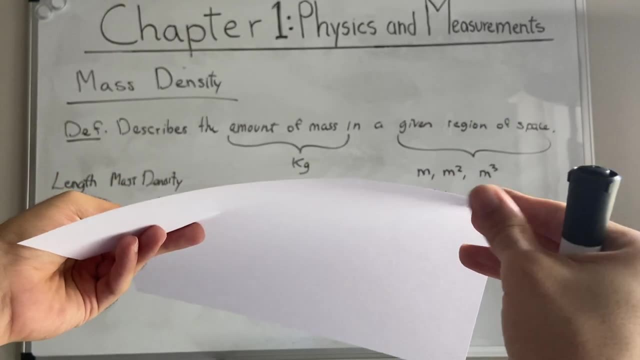 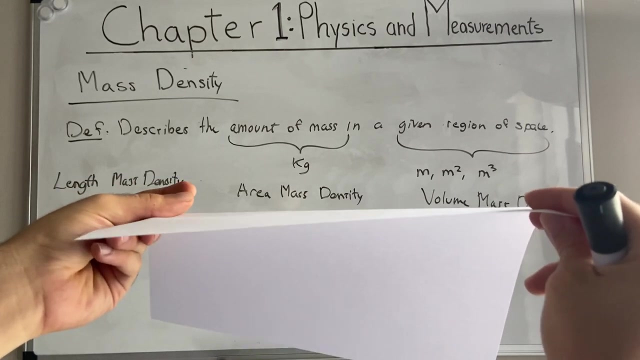 the side, And though pieces of paper are equally dense everywhere, I would suppose we can imagine that on one side there's more mass than the other, despite there being, despite it just being like a line and not more, not having more space on one side or the other right, And this can go. 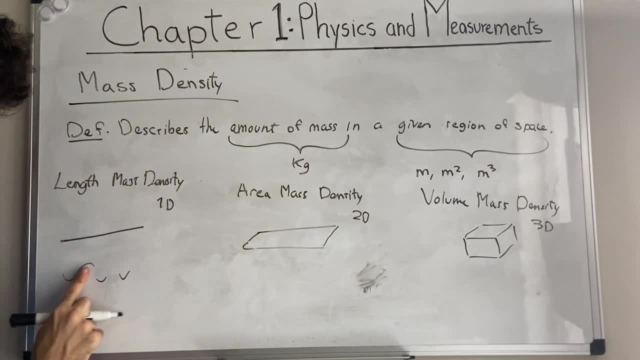 this can also work for: like: no, actually this cannot work for that, Or can it? No, no, no, this can't I. hmm, No, we'll just deal with one line. actually. No, this could work. 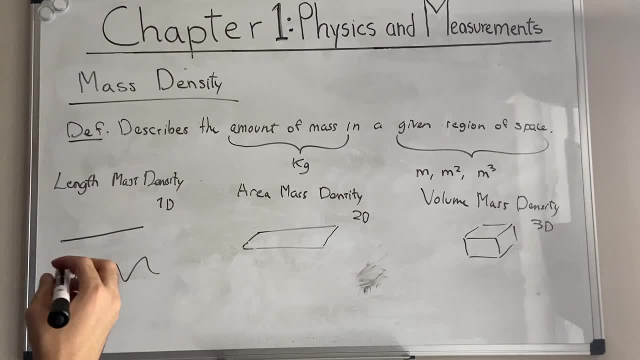 for this too, like a squiggly line. Yeah, it would work as well For mass density. would that work? No, actually I don't think so. Not 1D, I'm sorry. Area mass density- it's the same concept. 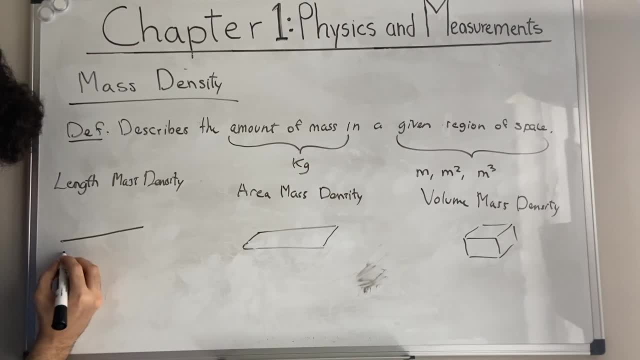 but there could be a large amount of mass here. I guess let's put arrow up mass, And then over here, low mass, And over here let's say this low mass as well. Let's say that this is very heavy. 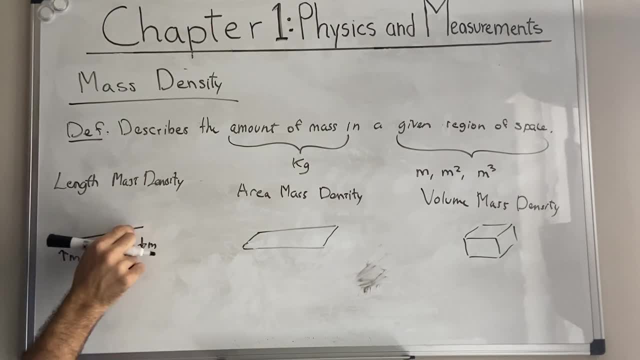 And then here is lower. is it a little lighter, lighter and lighter, right? So that's basically how we define density in anything mass density. It's just that these different scenarios are just for different dimensions. Here we have one. 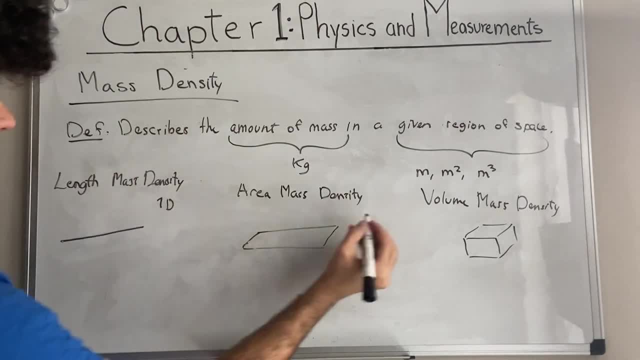 a 1D situation, Here we have a 2D situation, Here we have a 3D situation. In this situation where we're basically dealing with like a paper, a paper, a seam from the side, Let me grab one really quick. 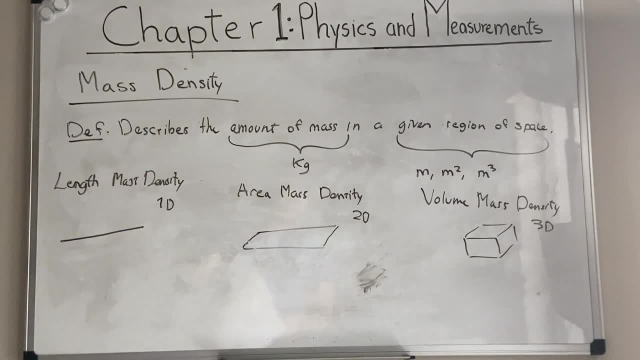 If you look at a sheet of paper, it's like a sheet of paper. It's like a sheet of paper. it's very thin from the side And though pieces of paper are equally dense everywhere, I would suppose we can imagine that on one side. 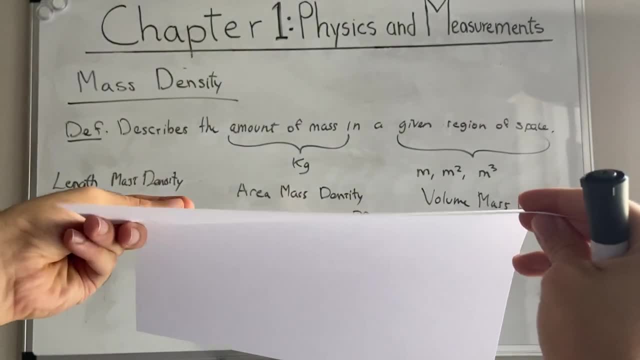 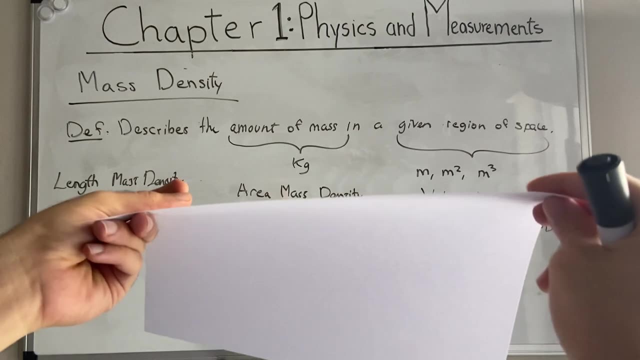 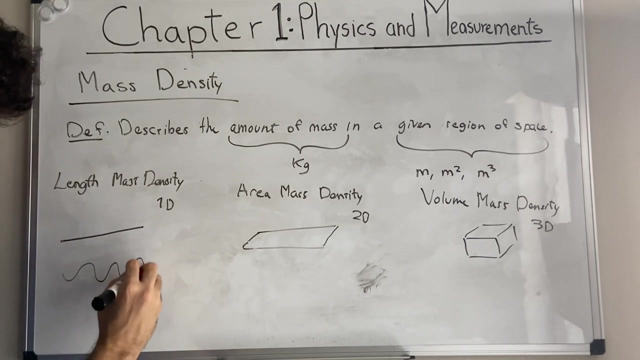 there's more mass than the other, despite there being, despite it just being like a line and not more, not having more space on one side or the other right, And this can go. this can also work for like no, actually. 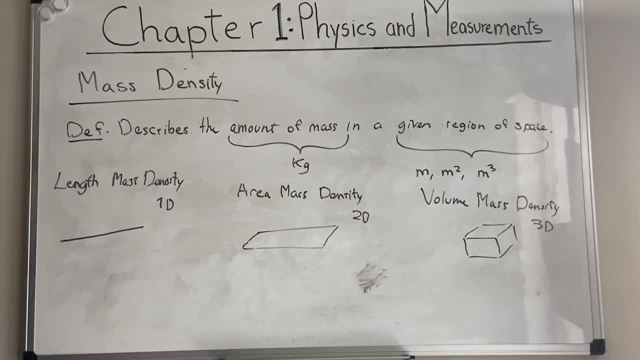 this cannot work for that, Or can it? No, no, this can I? hm, no, we'll just deal with one line actually. No, this could work for this too, like a squiggly line. Um, yeah. 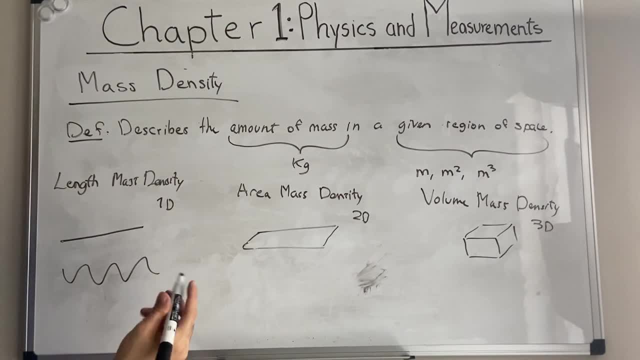 it would work as well. Um, for mass density, would that work? No, actually I don't think so. Not 1D, I'm sorry. Area: mass density- it's the same concept. It's the same concept. 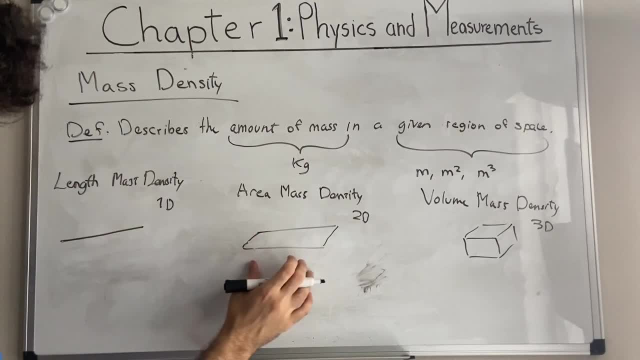 So it's the same concept but we're dealing with a plate and here we're dealing with a volume, And the reason I'm talking about this is because we have a way of um just deriving mass from these, different from equations that define the mass density of a line.